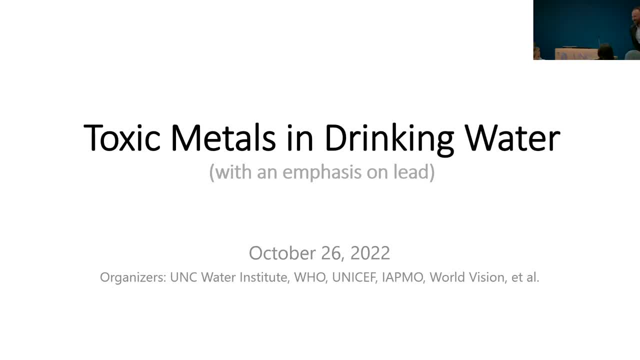 Yeah, if anyone in the back wants to scoot forward as much as possible. there's going to be some good dialogue in PowerPoint, But I'll have some smaller writing so you may want to be able to read some of the slides. Okay, great. 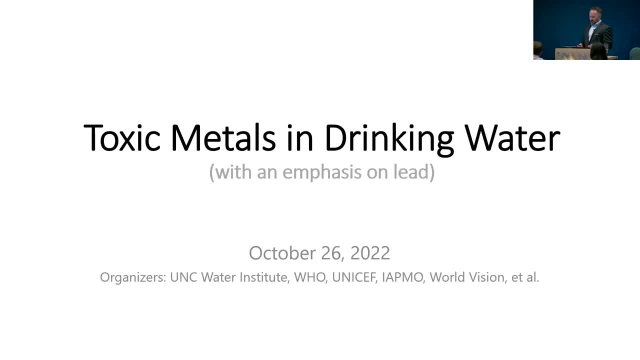 So we will go ahead and get started. Thank you so much for coming to today's session. Toxic Metals in Drinking Water. We'll talk about quite a few different contaminants in water throughout the day and the issues that we're seeing, But with a particular focus on lead. before we get started, I want to introduce myself. 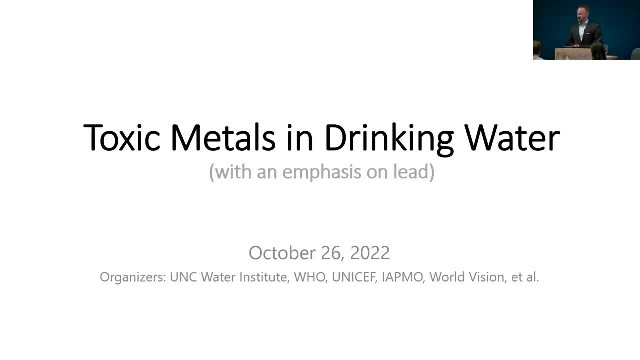 My name is Dane Hanson. I'm with the International Association of Plumbing and Mechanical Officials. We're a global trade association that's been around for about 100 years. We do plumbing codes, standards, specifications, training and also certification of testing of products. 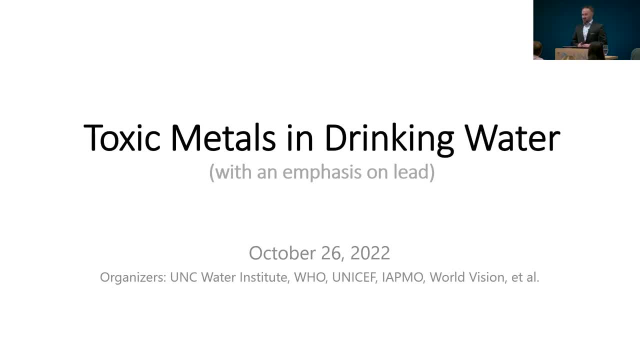 So a little bit about that. We test and certify in the United States about 99% of the plumbing market and we do this globally as well. So we make sure products are compliant with lead contamination flow rates and any other contaminants or plumbing specifications or standards. 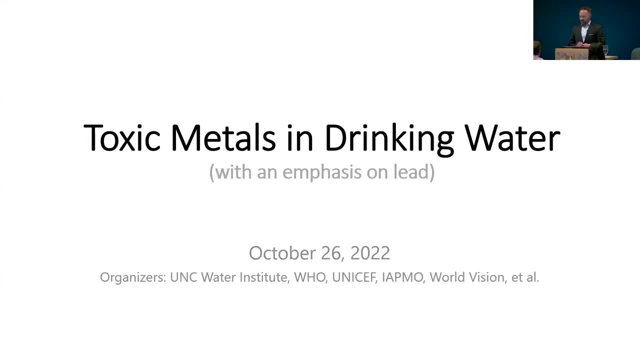 So we do this globally and we work with many in this room on implementation of projects overseas as well, And you'll hear from my colleague today, Christopher Lindsay, and others. I do want to let everyone know that this is being recorded. It will be relayed asynchronously in a couple of days. 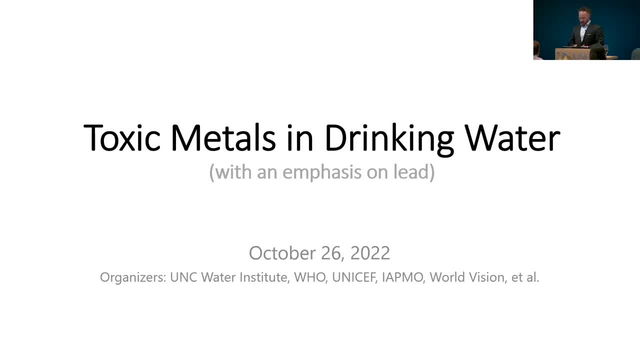 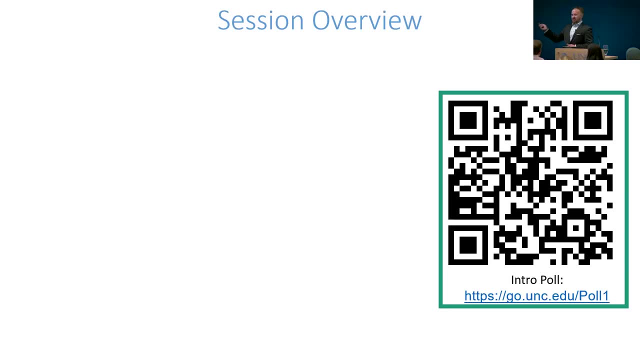 So we can replay it and people can watch it later on. One thing I want everyone to focus on: if you can, if you can, pull out your phone and scan this QR code. this is a way to introduce yourselves to us And then when we start having communication with the team- and there's some on the sides- 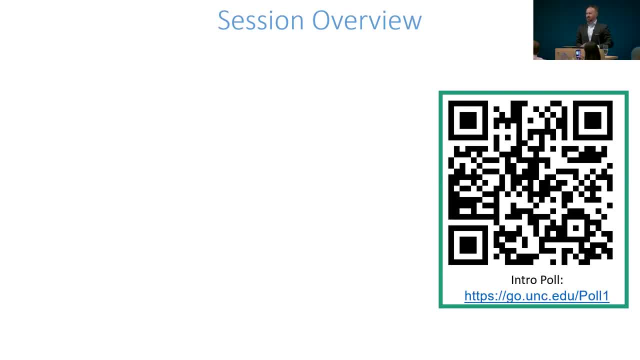 if your camera on your phone doesn't pick us up, there's posted around the room here as well, So you can also input your information, your name, kind of some background about you, so we know who's here And we can start engaging with you. 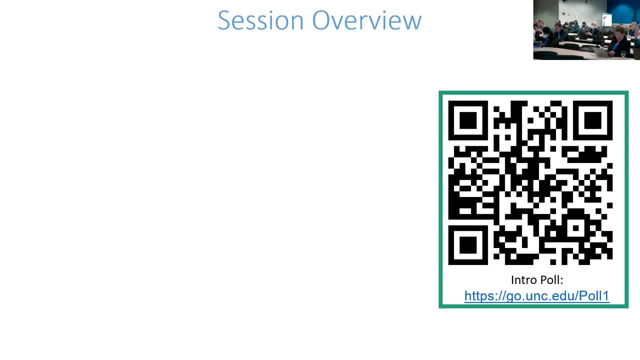 And also for follow up later, and we'll do a few different QR code polls as we start developing questions, because we want to hear from everybody. So for you to want to submit a question on virtually, or if you want to go to the microphone, 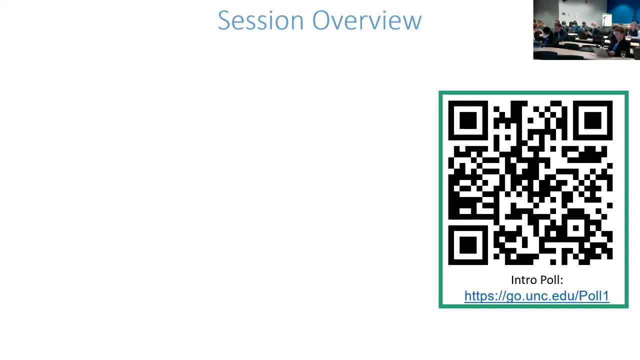 and do it as well. we will be able to talk about this for a little bit. So if anyone has any issues, let us know. And again, we want to make this as an interactive as possible. This is a really special opportunity. 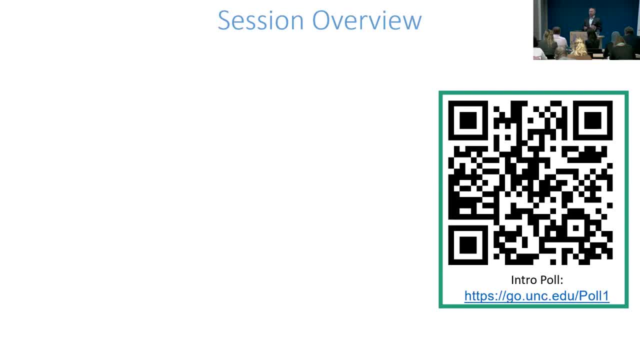 And I think I've mentioned this before. I want to highlight why this is such an important issue. So we've talked at this conference and in our work a lot of times. we talk about various pathogens in water, bacteria, things to that effect. 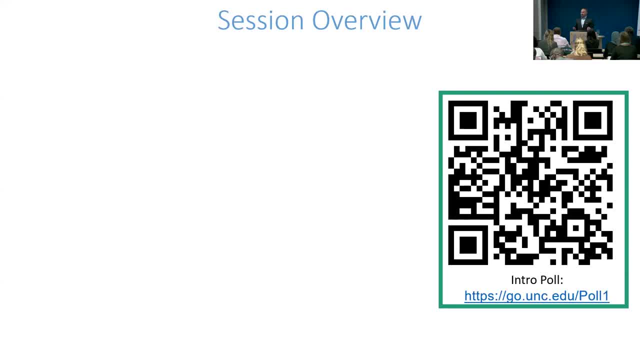 Oftentimes we don't talk a lot about the lead and other trace minerals and metals within water specifically. We don't get into that level of detail often. Oftentimes it's we pick one or the other: Let's address the bacteria in water or let's address them. 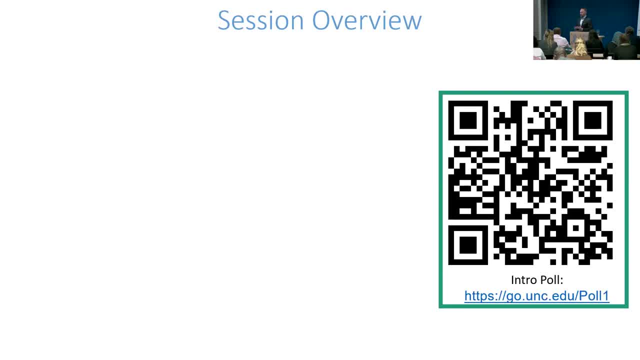 These can be done together And the beauty with this issue is This is all solvable. We can address these issues because a lot of them it's through the products and materials that are being used. We've come across this and it's very neat because we're here at UNC. 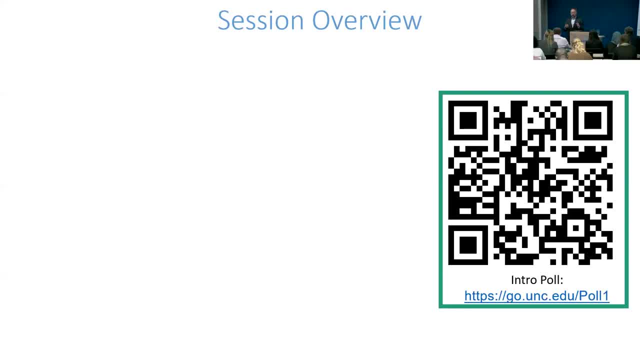 And the great thing here is we actually had this discussion years ago with many people on this panel. At this time back- I think it was in 2016,, 2016 or 2017, we started to come across issues where there was a prevalence of lead in drinking water in communities where various materials 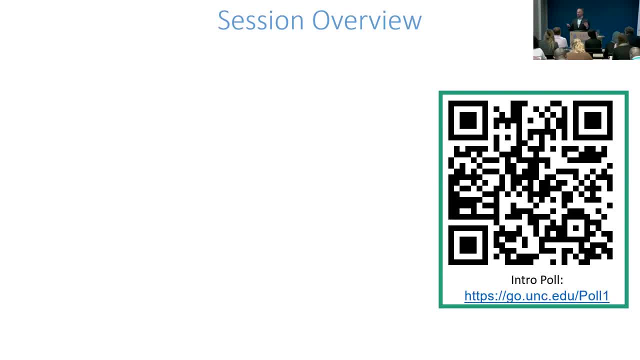 and hand pumps were installed And we're starting to find early on. this is a big deal: World Vision, WHO, UNC and many others. we had these early discussions and said, wow, we need to dig into the bottom of this. 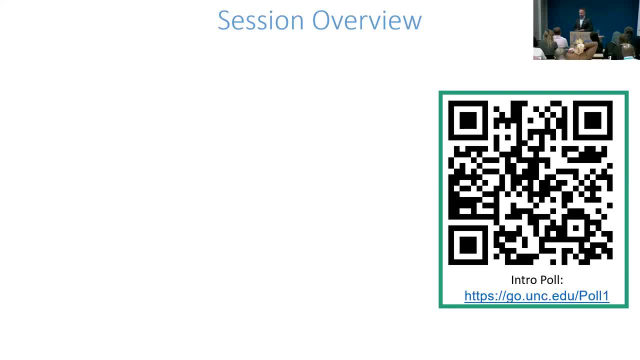 We need to get to the bottom of this, of what is happening and through incredibly great work by World Vision, WHO and UNC and others. So it's kind of fitting that we can come back and report on some of these findings, some of the effort that's been done, because this discussion happened years ago at this conference. 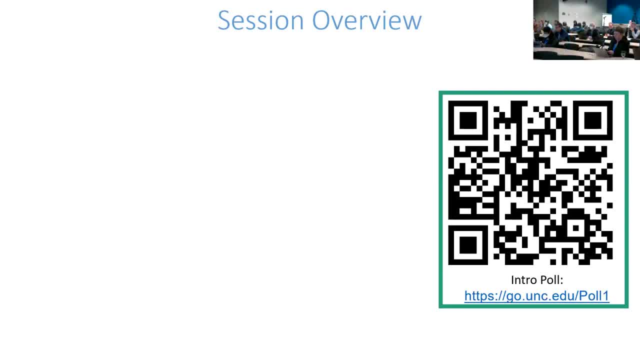 when it's actually this big cohort. A cohort came together to try to figure out how to address this. So I want to talk a little bit about today's presentation and how we're going to kind of the structure of it. So we will start off, we'll bring in some presenters which we'll introduce and we'll 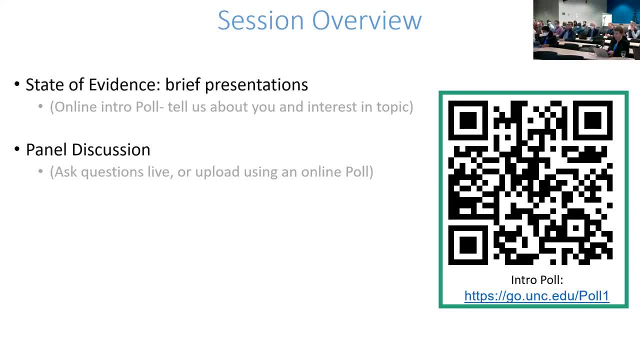 have the state of evidence, talk about what the issues are out there. We will then have some polls that we can engage with the panels and get to know them and get to know the issues and actually answer any questions you may have. We will then move into a panel discussion. 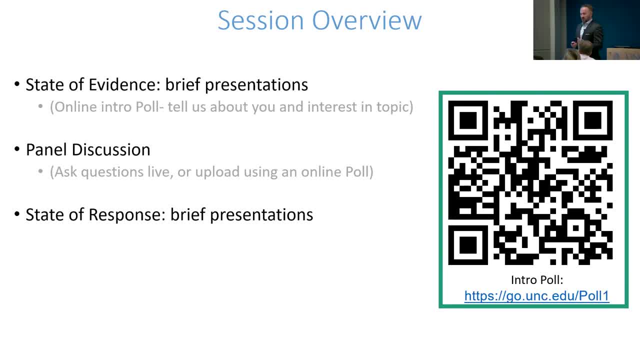 I'll be able to talk about some of the issues, Thank you. So we'll be able to engage, hear what's going on and how prevalent this issue is and what people are doing to address it. We will then, you know, have a state of responses. 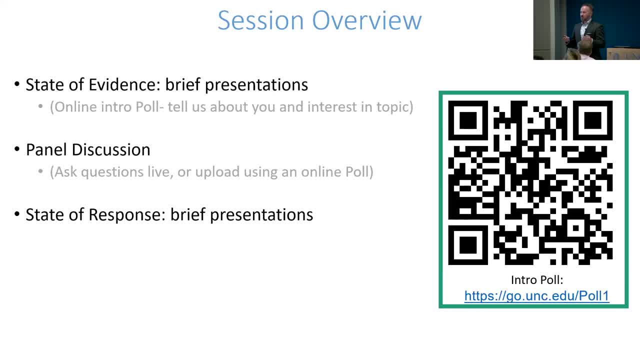 So we have additional organizations who will come up and talk about what is happening now, what is the industry doing to try to correct this problem and how do we all come together to make this work? And then again we will break into groups. if we have time, hopefully we will break. 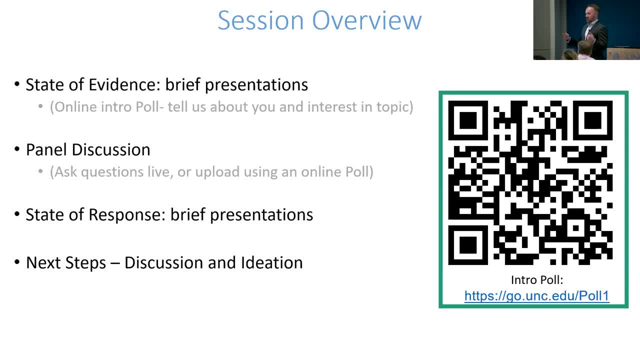 into groups and small groups to kind of run through some ideas of how we can come together and solve these problems from everyone's perspective and ask the questions And kind of do a recap. We will upload these and people who submitted their information- we have contact information. 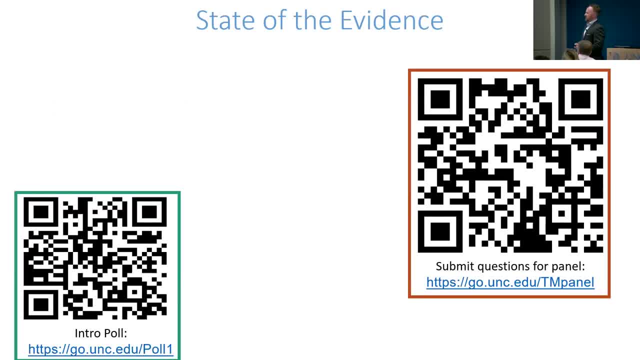 we'll be able to continue to collaborate with you on this idea. So, as we begin to move into the panel side, hopefully you've everyone's included your information. here's another QR code So, as things come up as we talk to the panels, you may want to scan this as well, because 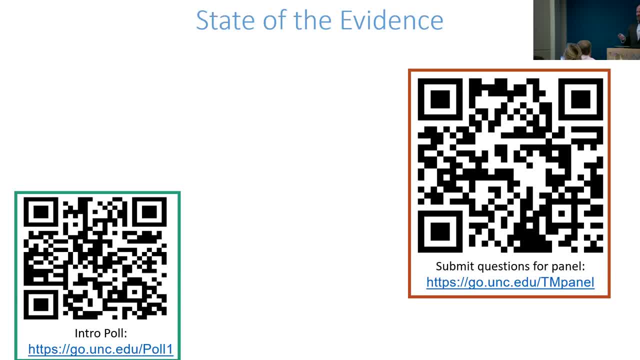 this is going to take you to a place to be able to submit questions, And over here we have questions. These questions are going to be populated on the computer here where we can try to respond to them and engage. So we'd love to invite our panel to talk about the state of the evidence currently right. 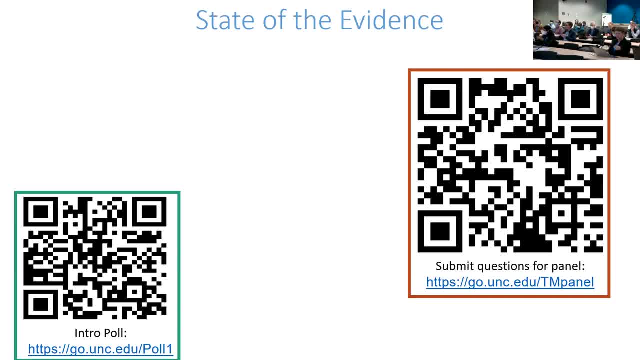 now. So we have Sid Roy when we call your name, if you can come up and join the panel. He's an environmental engineer and research associate with UNC. We have Jorge Alvarez Sala, who's online virtually, who will join us as well. 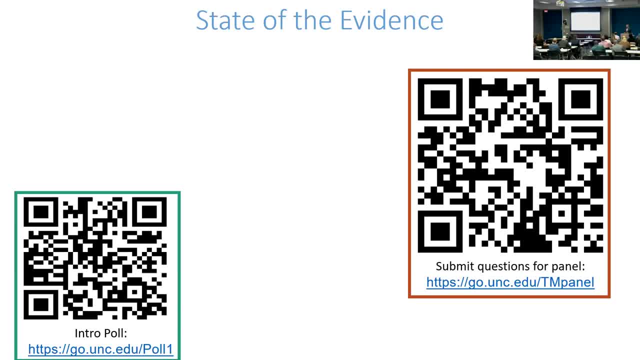 He's a senior advisor for water and climate resiliency at UNICEF. We have Jenny Redman with RTI International. she's a director of environmental, health and water quality, And we also have Jennifer DeFrance, who's the WASH technical advisor for the WHO. 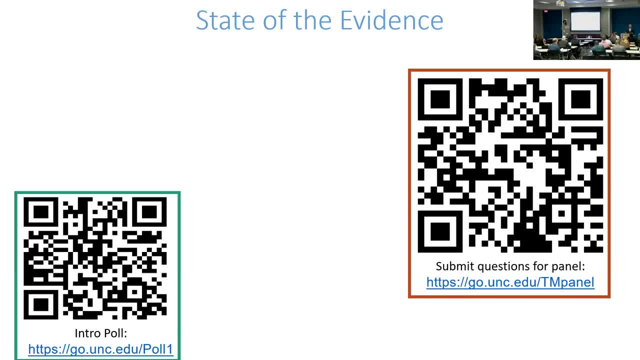 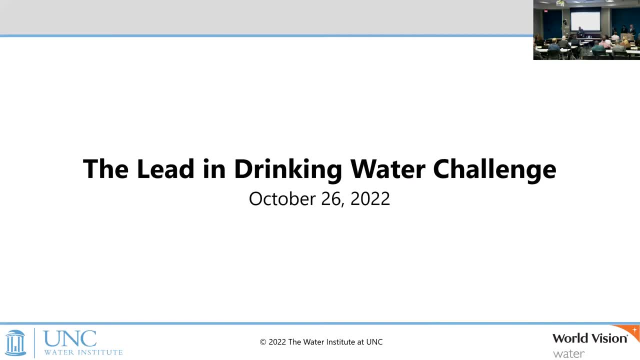 So we appreciate people traveling here from other countries to be here as well, So we'd love to have you come up and join us on the panel up here. Jennifer DeFrance, RTI International. Here's the you can scroll through and the presentation should be there. 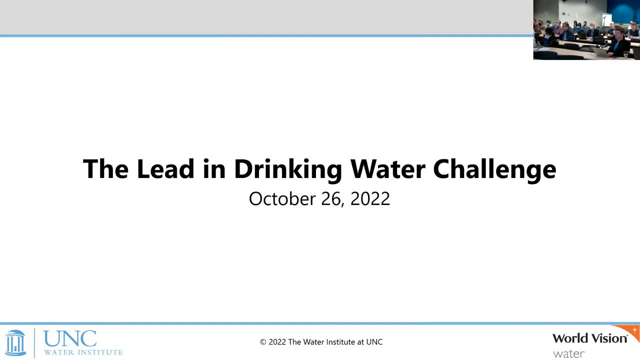 You can sit here if you want to do it, or you want to stand here and do it. It's going to be hard and I'll just stand here. Oh, you can sit there. I want to sit here, Okay, Perfect. Good afternoon everyone. I'll start us off with a quick review of lead in drinking. 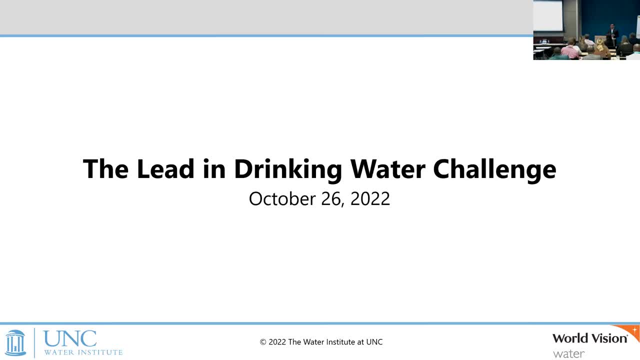 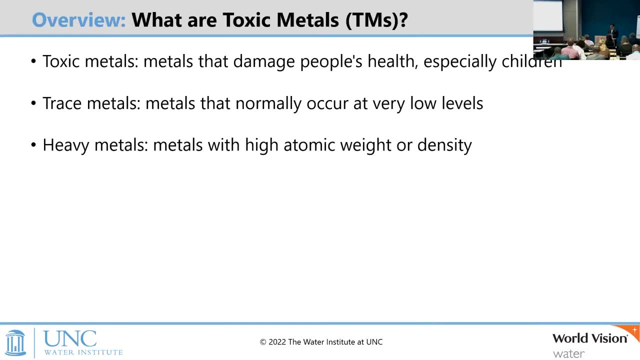 water and talk about the evidence that has been collected over the years by work done here at UNC in collaboration with World Vision. Very quickly, what are toxic metals? And there are various definitions floating around. Toxic metals specifically refers to metals that damage public health, especially health of children. You have trace metals that sometimes that normally. 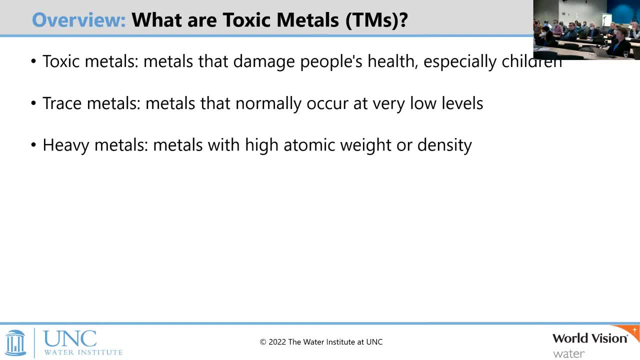 occur at very, very low levels. You also have heavy metals, which are metals with high atomic weight or density, And sometimes all of these intersect. But we decided to go with toxic metals because, you know, fundamentally we care about the intersectionality. 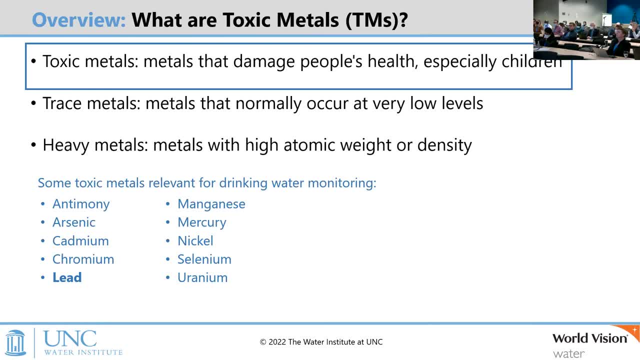 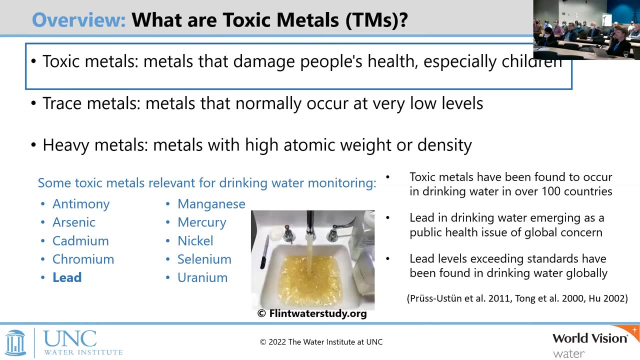 And so here are a list of metals that many of us are working on. Lead is obviously a primary focus. It's a potent neurotoxin. We've known about its dangers for two millennia And I'm sorry you cannot see this, but a lot of reviews and surveys done over the years have shown that toxic metals 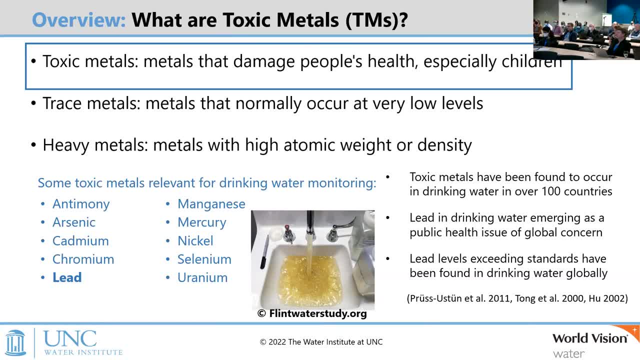 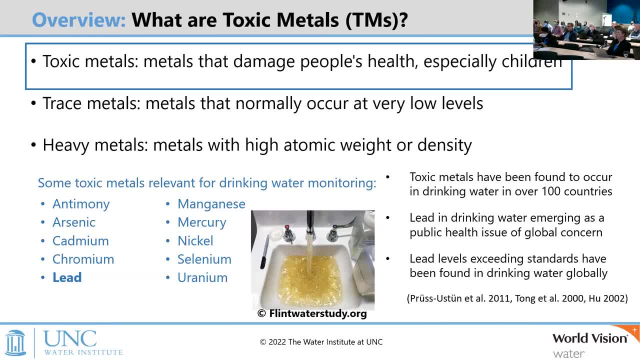 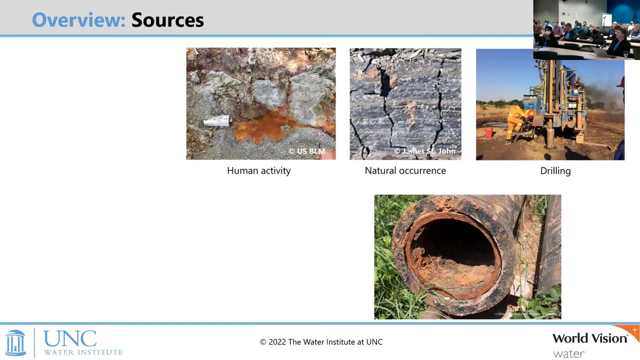 it's a very, very important metal, And it's a very, very important metal And it's emerging as a public health concern of a global nature- The fact that lead levels often exceed standards in drinking water in many of these countries, And obviously these different metals have various sources. 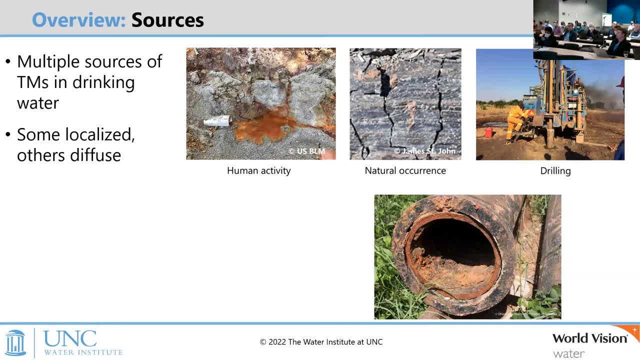 some of them natural, localized, others occurring from corrosion of a lot of these water system components that we've installed over the years. These could be pipes, These could be faucets, These could be other fittings that corrode over time because of aggressive water, chemistry or other factors and cause toxic metal levels to go up in water that. 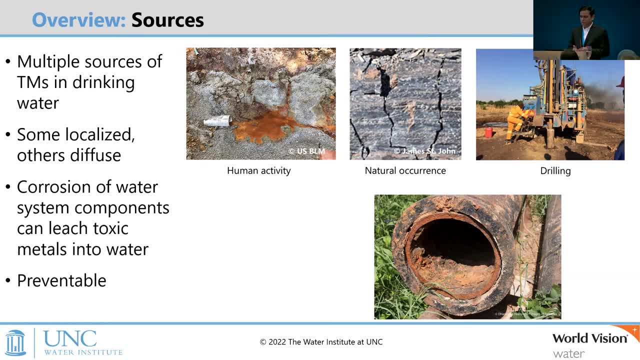 people are drinking. A sad part of this, obviously, is a lot of this is preventable, And so the goal should be figuring out what's going on where and putting in mechanisms, whether it's adjusting water chemistry, changing water system components or changing water system components, And so the 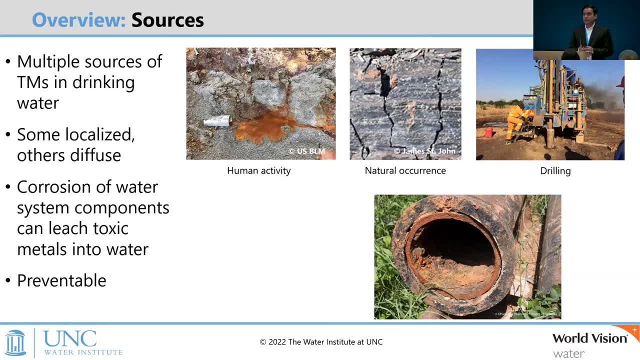 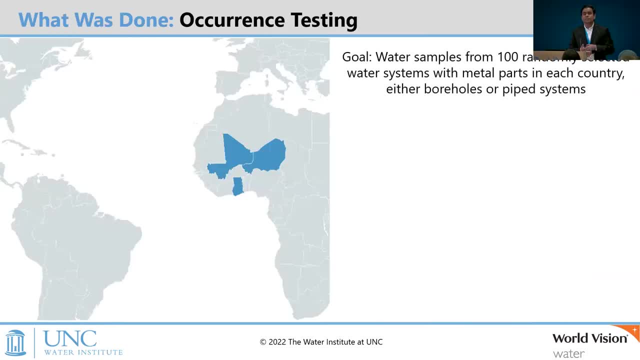 goal should be figuring out what's going on where and putting in mechanisms, whether it's adjusting water system components, whatever the solution, to reduce exposure to the public. Talking about evidence of the work done here, a goal of the 14 country evaluation study, one of the goals was to sample water from 100 randomly. 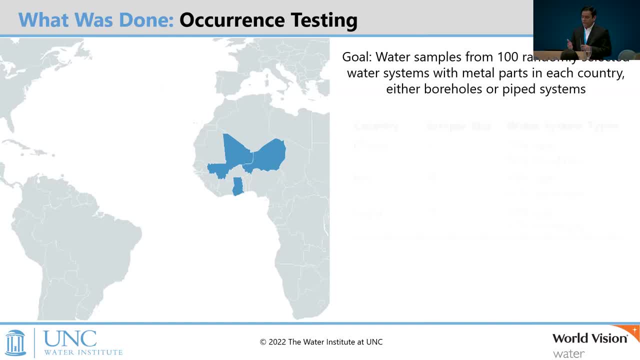 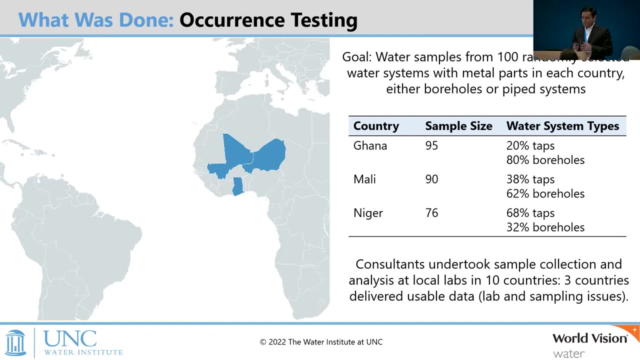 selected water systems with metal parts- And these could be either taps or boreholes- And to see what we find when we do this. And so we had enumerators going around the country and taking these samples And we were able to- well, I say we UNC, I was not here, But great work nonetheless. They were able data from only 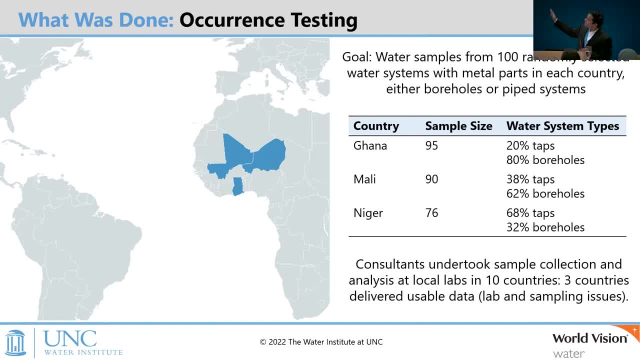 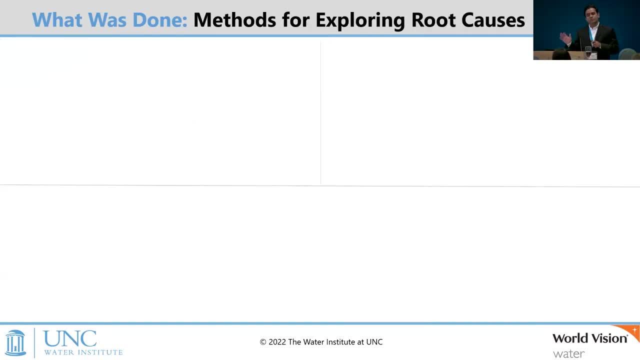 three countries was usable And you can see the distribution of. you know some of these samples came from taps, Some of these came from boreholes, And talking about the methods really quickly on what they did, You obviously had. you know all of these samples came from taps, Some of these came from boreholes, And talking about the methods, really quickly on what they did, 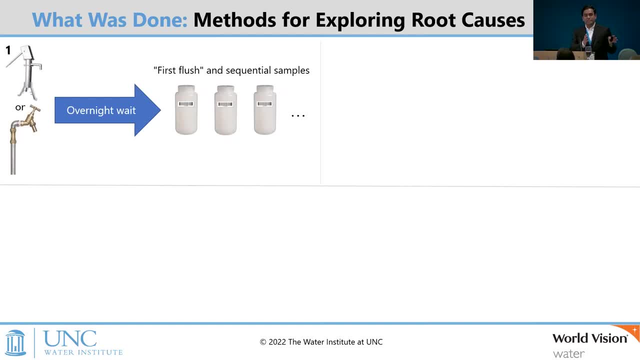 profiling, where you collect, where you let the water stagnate for some time and then you collect the first flush and a bunch of sequential samples to get a sense of you know what kind of metals you're seeing over time. what are the sources of those metals? uh, you have what's called a fully 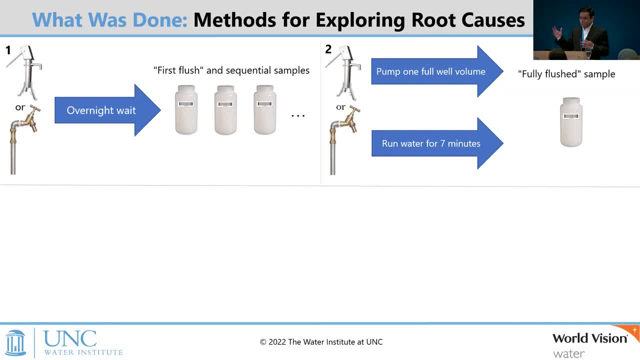 flushed samples, where the entire water system is flushed out, and then you collect a sample to see, uh, what could be. you know what's what, what's there? a third method that's also frequently common is in situ x-ray fluorescence or xrf, and the idea is you actually go and look at the components. 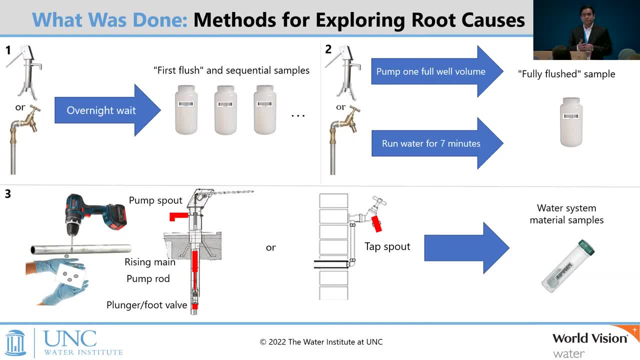 individually and use this handy handheld device to see you know what are the various weight components of these different metals, in a lot of these components. and a final method was actually taking metal samples like a small piece and then shipping it to a lab and then digesting. 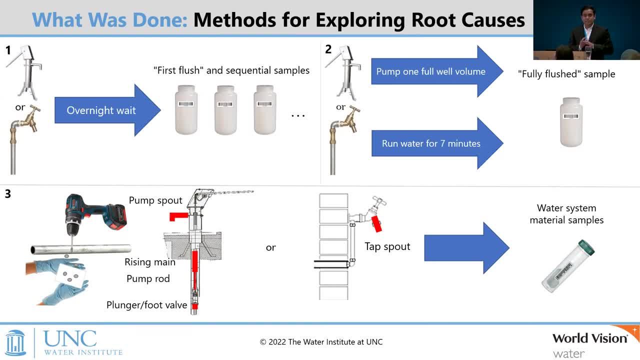 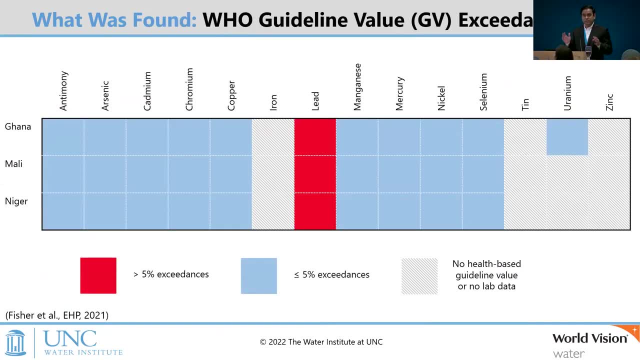 it and seeing what we find. i'm not going to present all the data because there's a lot of it, but here is kind of a big picture summary of all these metals, uh, you know, from the three countries where the data was usable- ghana, mali and niger- and the blue squares represent uh samples. 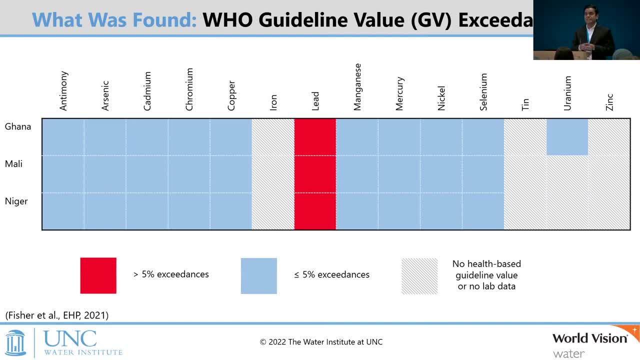 you know, less less than or equal to five percent of samples exceeded the who guidance value, and the red boxes indicate more than five percent of these samples exceeded the who guidance value, and only for lead. this, uh, it was consistent across all three countries that samples exceeded five percent. 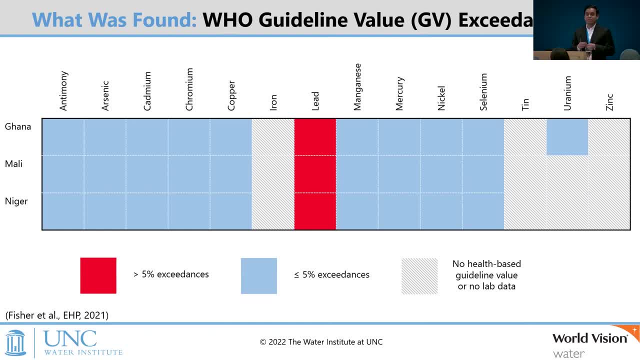 and so, just for your reference, the who led guidance value is 10 micrograms per liter. there were also other metals, for example antimony, iron and nickel, where we saw exceedances, uh for the national standard, which is different, which can be different from the who guidance value. 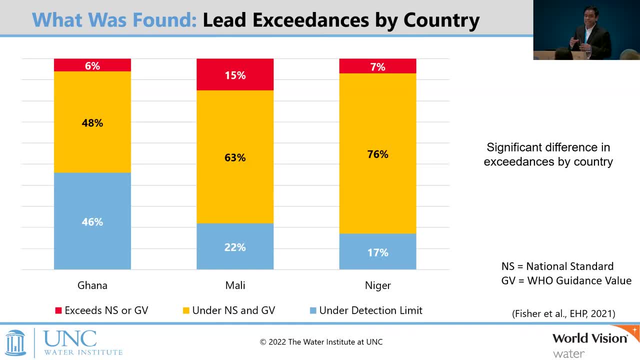 kind of looking at the data in detail. what do you? what do you see? again, the three countries on the x-axis, and you have data. the blue section indicates lead levels under detection limit, which is 0.5 micrograms per liter. the yellow bar represents lead levels above detection limit, but below the who guidance. 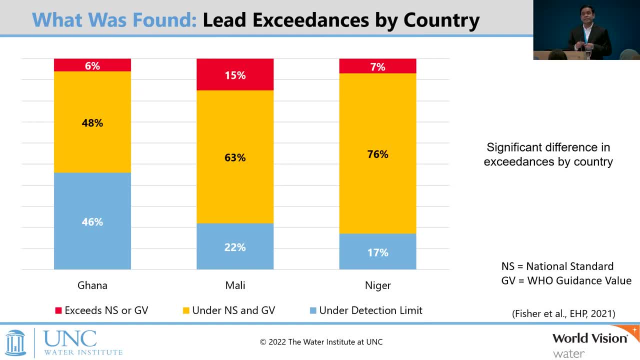 value and the red portion is that level succeeding the who guidance value. so you can see, you know distribution, uh, system level of lead levels. that's the yellow bar, that's the red level of lead levels, significant difference between the three countries. but fundamentally because we know there is no safe. 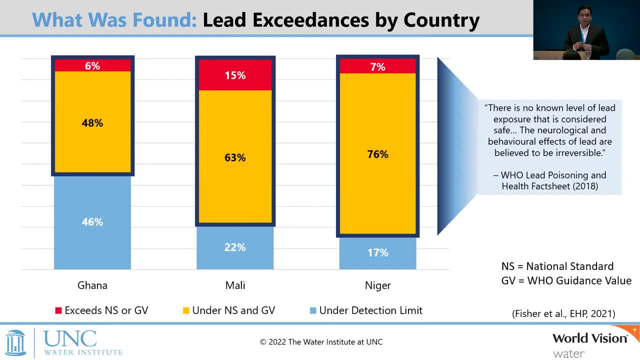 level of lead and the fact that the effects on the on the growing brain, on other body parts, is irreversible. the fact that you know a majority of of these samples we found some lead or a lot of lead, is a cause for concern and hence you know we need to have a proper response to these findings. 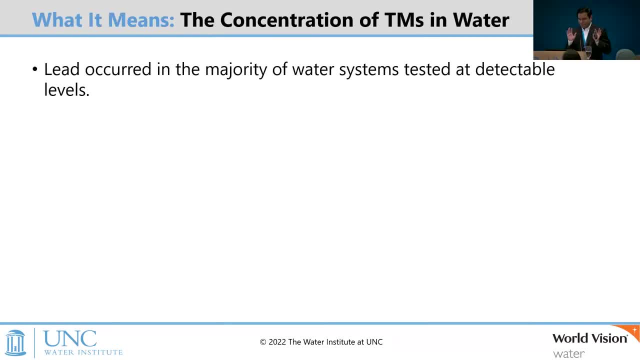 so, in conclusion, uh, you know that was just a couple of graphs, but fundamentally, uh, we know that lead occurs in a majority of the water systems that we tested at detectable levels. um, if you want a single number, over overall nine percent of water samples exceeded national. 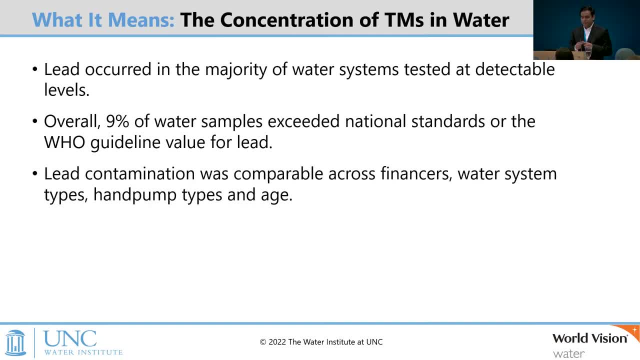 standards or the who guidance value for lead, and i did not present data on this, but lead contamination was comparable across financers, across water system types, across hand pump types and across systems of different ages, ranging from less than three years to more than 16 years. and and the fact that in some countries, uh, there were exceedances for. 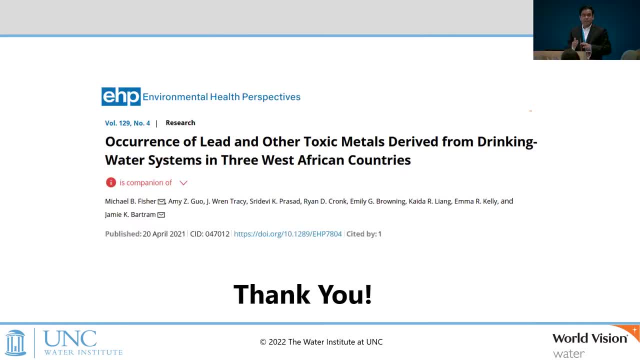 other metals like iron and ghana as well. um, thank you so much. if you're interested in more, uh, a great paper came out in ehp last year and dr mike fisher was the lead author on it and he can answer any questions you may have. 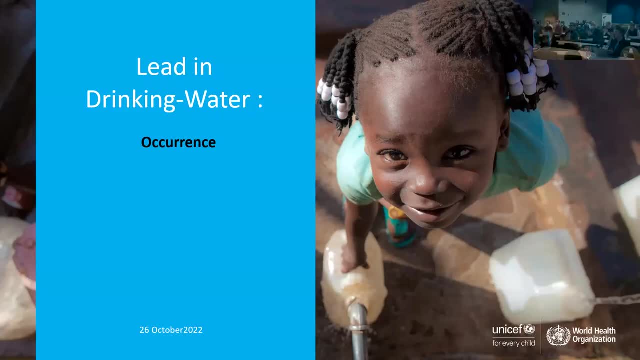 that's it from me. we will now turn it over to our virtual participant. hi, good afternoon everyone. i hope you can hear me. can you, can someone wave, or okay, fantastic, thank you very much. i'm pleased to be here today, although virtually i would have loved to be in a chapel hill. um, i will now provide a bit a brief overview of 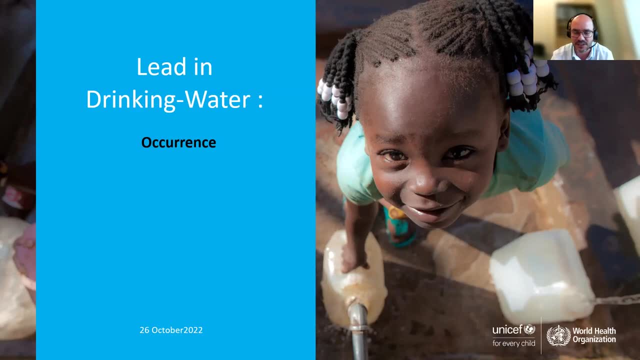 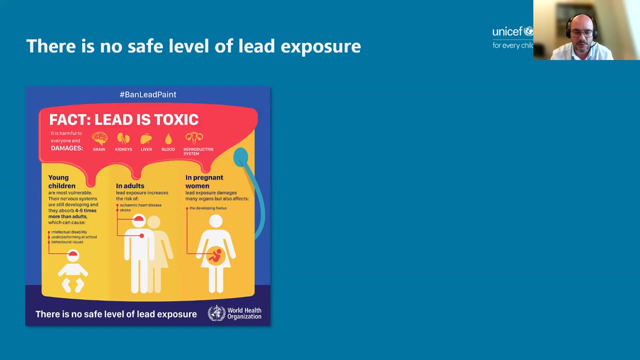 how important is lead in a contamination in in drinking water? next slide, please. yeah, fantastic. so according to who? there is no safe level of lead exposure. let is recognized as a chemical factor, as a chemical of major public health concern that should be included in national drinking water quality standards. 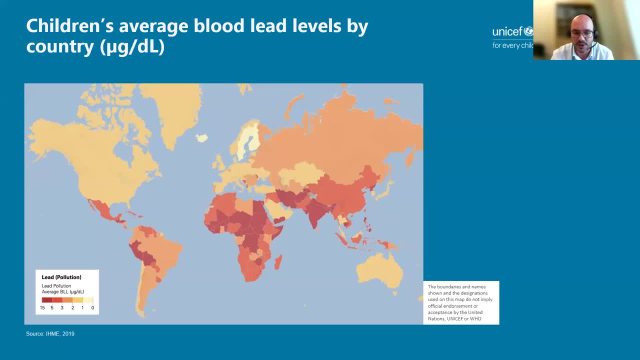 standards and monitored as part of a drinking water quality surveillance program. let sorry things that the previous slide. lead concentrations in drinking water should be kept as low as reasonably achievable. lead is toxic to humans and is particularly harmful to children. damages include intellectual disabilities and their performance at school. behavioral changes. 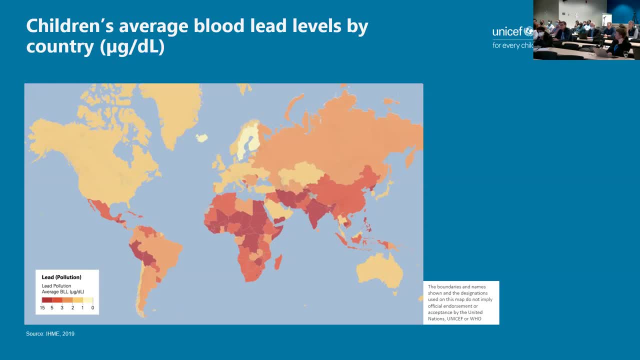 and increased risk of health, health problems such as ischemia and strokes, and fetus development issues in pregnant women. in this slide you can see: yeah, that that was the, the one that they mentioned. but if we move to the, to the, to the, yes, to this slide, the. in this map you can see: 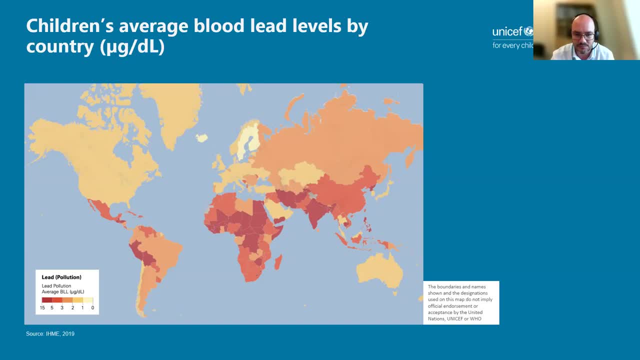 children's average blood lead levels by country. analyzing blood concentrations in children is important not only because uh they are more vulnerable to lead, but also because it is relatively easier to establish the potential sources of those lead concentrations in their bodies. and in a recent research, unicef found that as many as 41 percent of children in georgia- in georgia, the country not 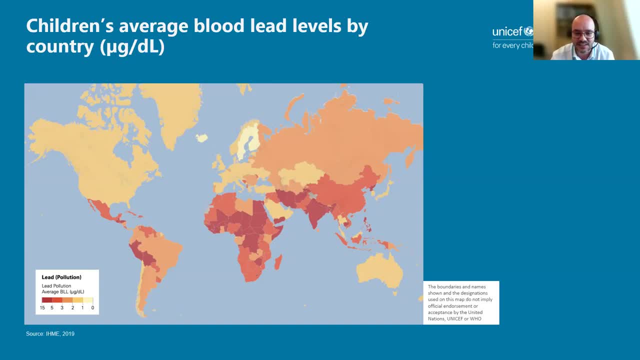 the the state had blood lead levels greater than or equal to five micrograms per deciliter. per deciliter, and while there is no known level of lead exposure that is considered safe for human beings, five micrograms per deciliter is the baseline at which the world health organization. 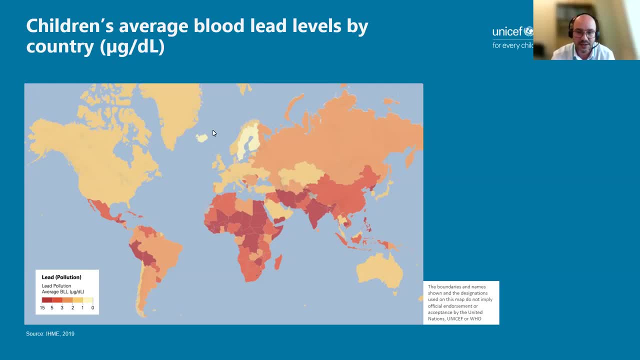 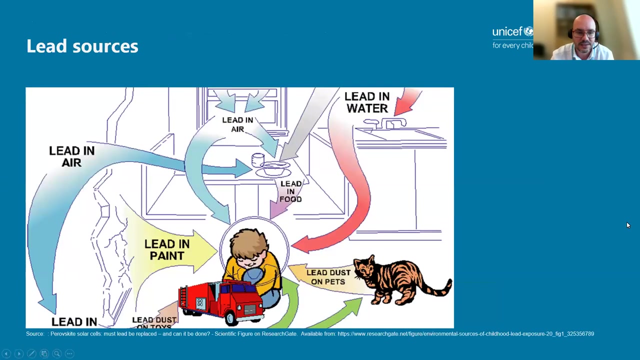 recommends initiating public health action. it is important to mention, however, that those concentrations of lead in blood come from different sources, so not only drinking water. next slide: iste вот please. 224 00, 225, 00, 206 00 00. you can see the different lead sources In the past: lead in fuel, for instance, spread through air. 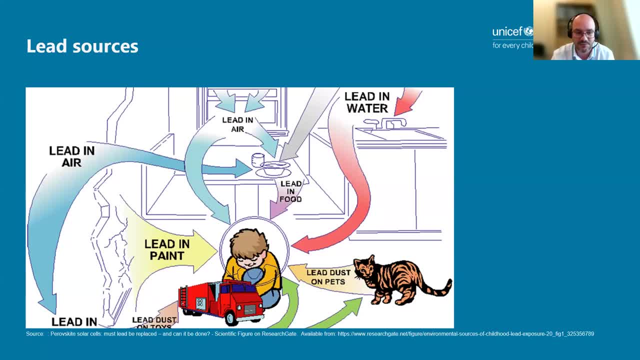 was considered an important source of contamination but, luckily for the world, recently all countries phased out lead additives in fuel, and it is also important to mention that there is insufficient information at the moment about the importance of lead in drinking water as a contributor to the high blood levels identified across the world. 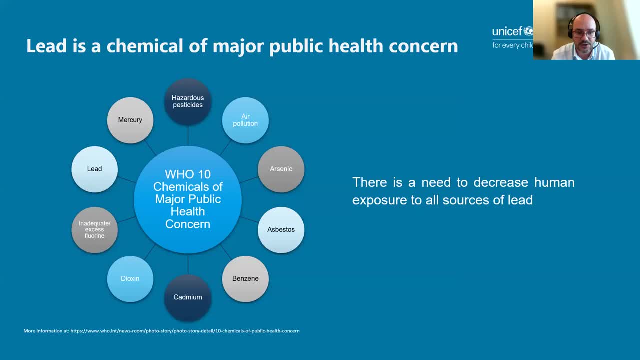 Next slide And, as I mentioned earlier, lead is one of the 10 chemicals of major public health concern and although arsenic and nitrates have been a key water quality parameter and those chemical contaminants are included in the JMP, in the joint monitoring program guidelines, Maybe at this time, 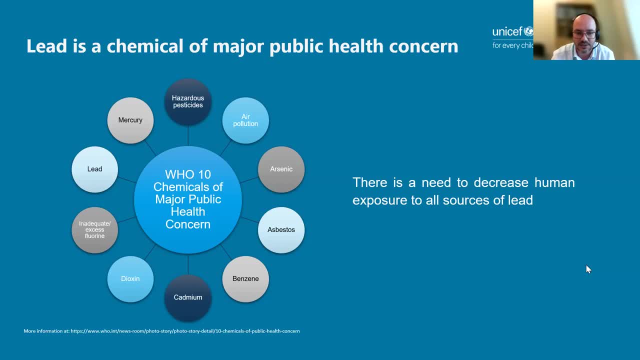 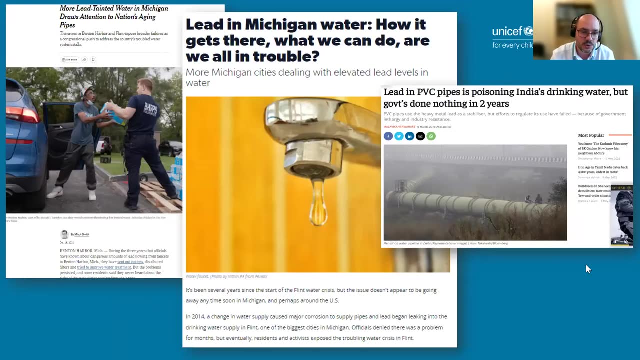 to increase surveillance and water quality testing of lead as well. Next slide: Water quality issues usually attract a lot of users and mass media attention, and for a reason, and here you can find some recent examples from Flint in Michigan, but also in other countries and contexts where lead has attracted interest from both consumers as well. 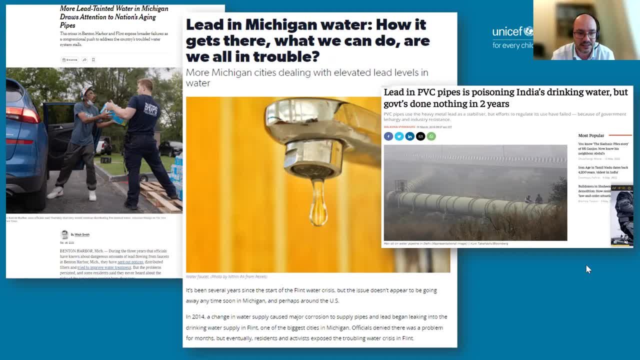 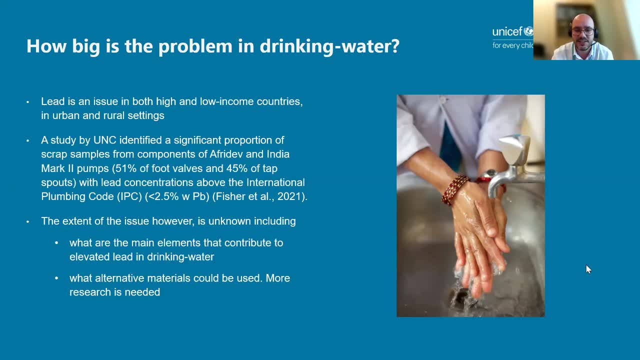 as media And the last slide Now. the key question that many of you may have is: how big is the problem in drinking water? Well, I'm afraid it's difficult to say now. There isn't sufficient evidence on how much of the lead in blood samples can be attributed to drinking water and, at the same time, there 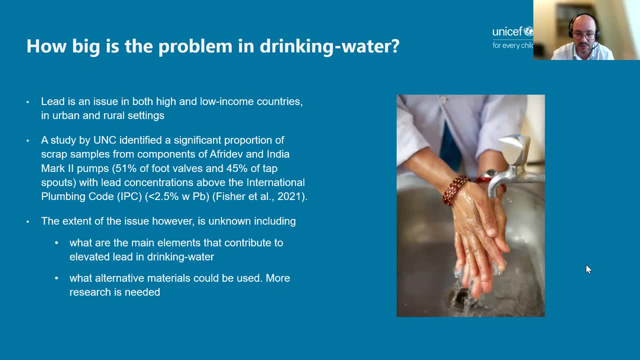 isn't insufficient information on the extension of the problem at global scale. However, lead seems to be a larger issue than initially thought. I think the example from the UNC research in west Africa shows that is a global issue affecting both low and high income countries and both rural and urban areas. 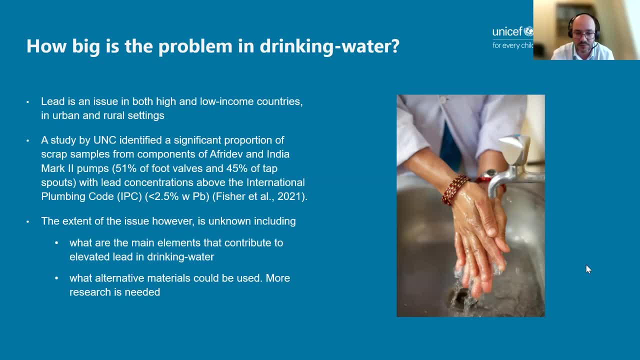 The extent of the issue in the water sector, however, is still unknown. what are the main elements that contribute to elevated lead in drinking water and, at the same time, what alternative materials? and, assuming that materials seem to be the main cause of lead contamination in water, what alternative materials could be used so in in those two areas? 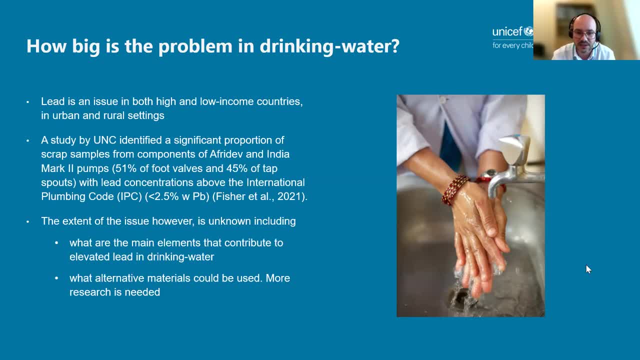 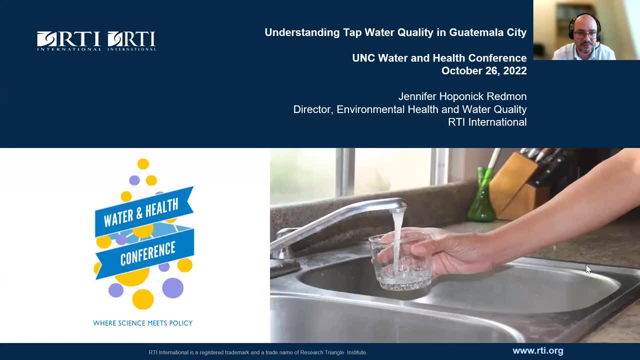 there is still some research needed. i will stop here and pass it over to jennifer. ok, thank you. my name is jennifer hovinnick redmond and i'm going to briefly esc stop review some of the water quality research we've done in guatemala city recently with 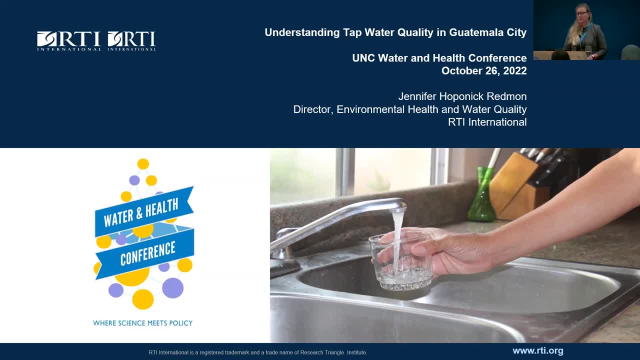 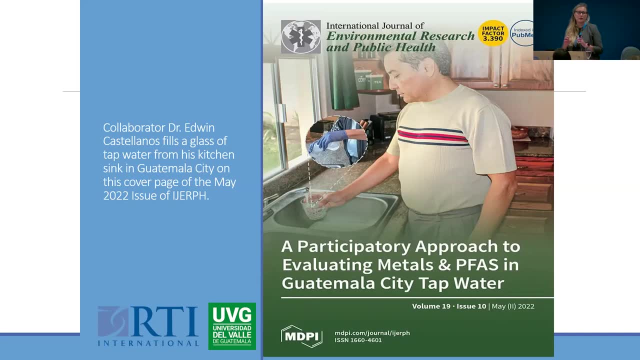 the water quality research we've done in guatemala city recently with property Sophie, a focus on metals including lead and PFAS. So this was the cover of the issue where we published this article, and I have a QR code at the end if you'd like to look at it. but this is actually 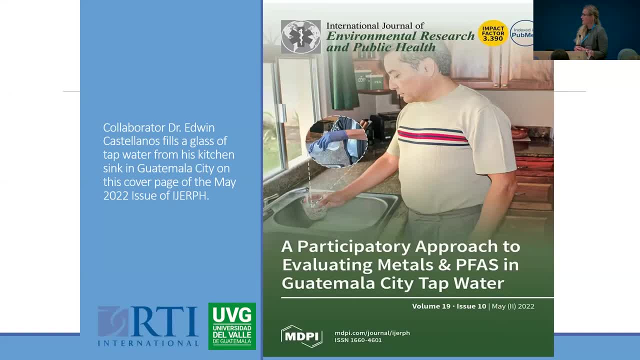 our collaborator, Dr Edwin Castellanos, and he is filling a glass of water in his home- and we used a participatory science approach to collect these water samples and analyze the data, which worked especially well because we started this the first month of COVID, So I was originally 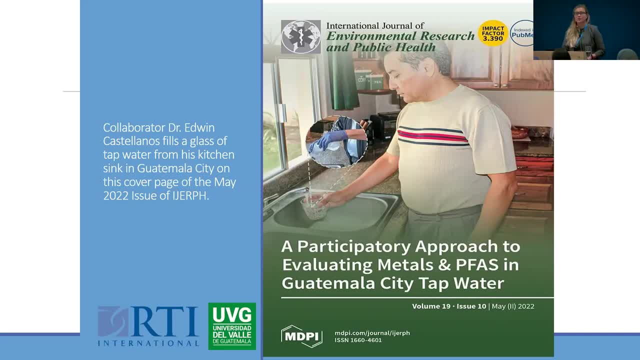 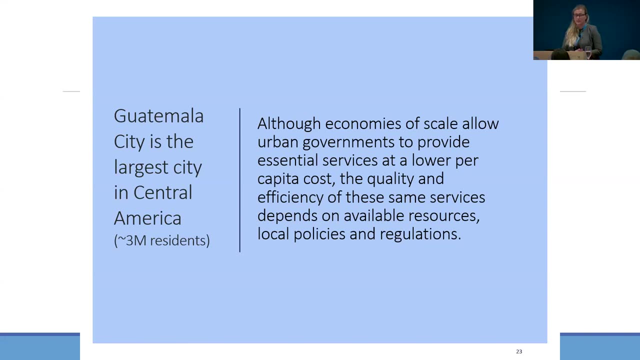 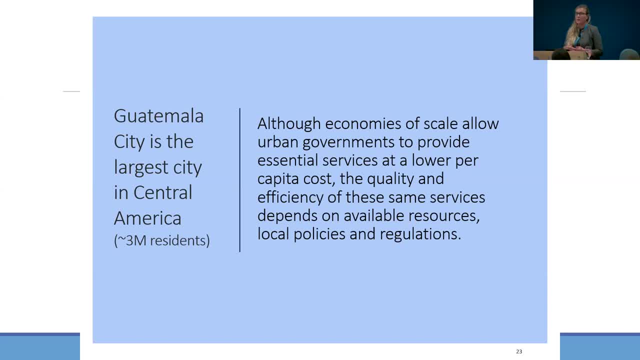 more urbanization continuing to occur. People are moving from rural areas to urban areas for better opportunities and for better infrastructure, and although economies of scale do allow urban governments to provide essential services at a lower overall per capita cost, there are still limited resources and the municipalities are subject to their cost limitations and regulations. 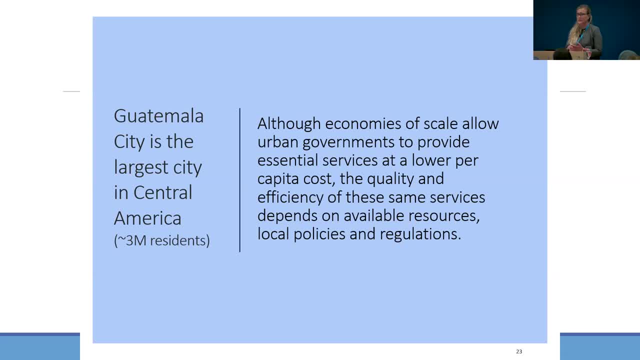 for how they can provide essential services. So I think it's a really important thing to think about in terms of how we can provide water quality to residents. So residents in Guatemala City do still often have issues with service throughout the day. Oftentimes they might need to. 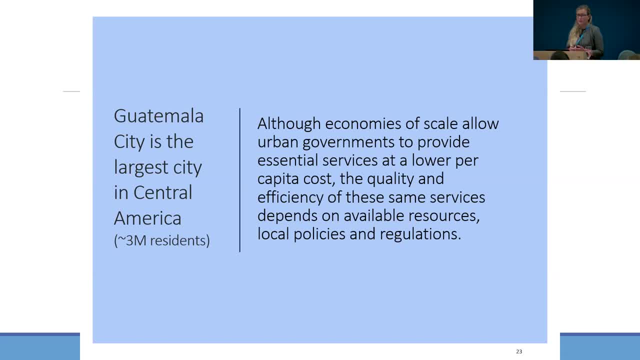 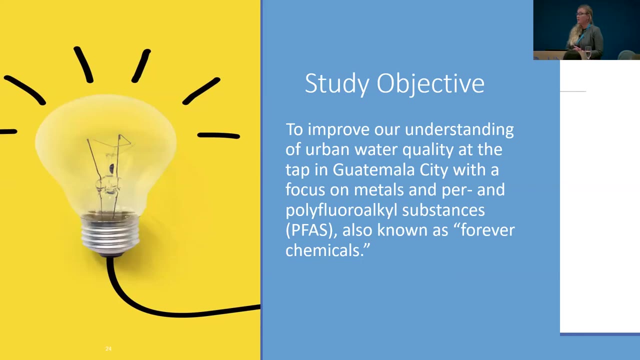 store water, to be able to access water throughout the day, and there's limited regulations in testing specifically on metals and PFAS, which has never been tested before. So our study objective was to improve our understanding of water quality at the TAP, with a focus on chemical water quality and. 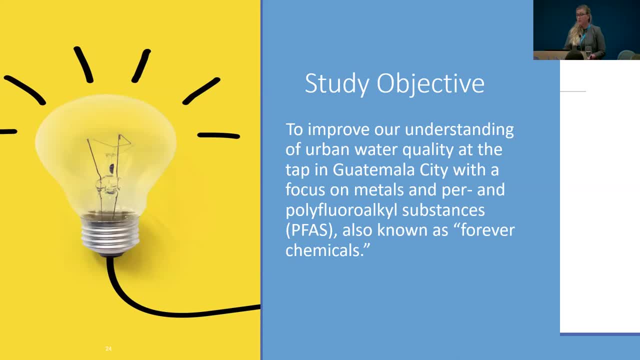 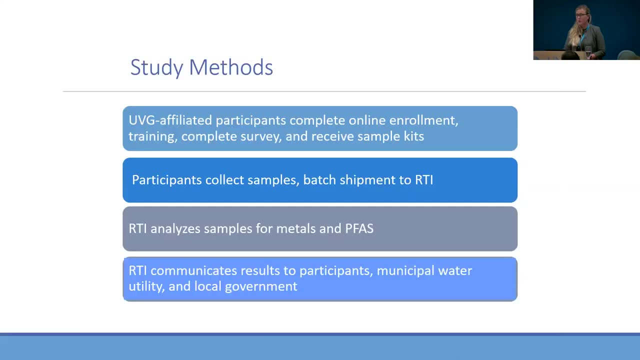 water quality metals and per and polyfluoroalkyl substances, which are also known as forever chemicals. Our methods were to: we worked in conjunction with UVG, the University de Valle, Guatemala, and there were affiliated participants of the university for participation. 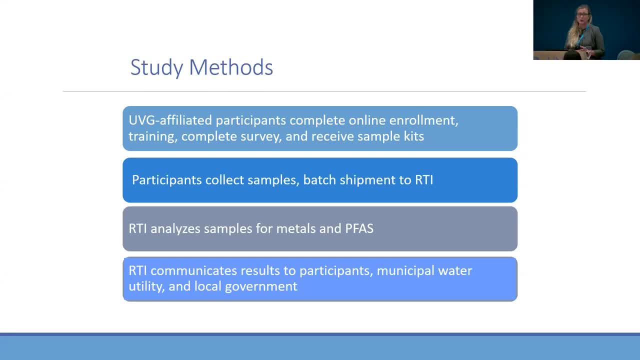 And so that meant students, staff administrators, maintenance staff or plumbers or former alumni were also allowed to enroll. We had online enrollment and then we did training online through a webinar, along with written instructions, and we had a video as well. 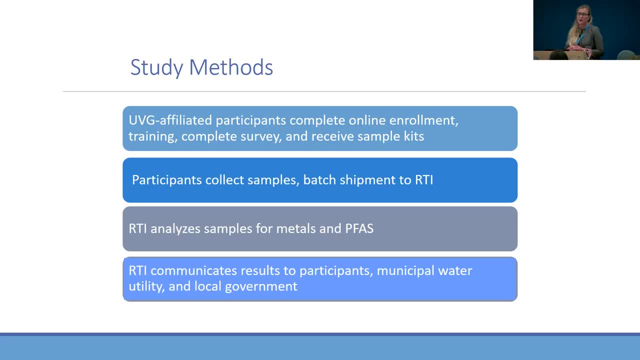 We shipped all of the samples down to Guatemala and there was an outside pickup or you could have a courier at your door with COVID. They completed an online survey and after receiving their sample kits, they collected first. draw water samples first for metals. 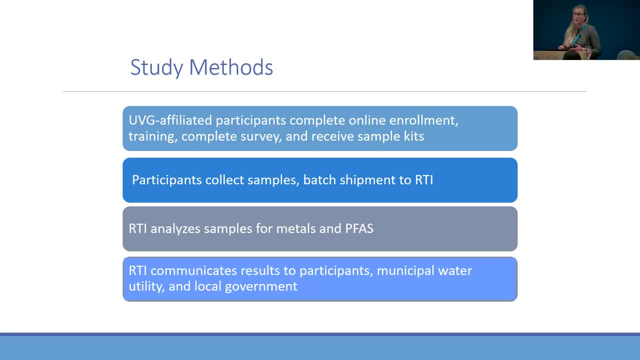 Followed by a sample kit, And then they collected the samples, and then they collected the samples, and then they followed by running the water and collecting the PFAS samples. We then batched all of those samples back and they went through FedEx internationally. 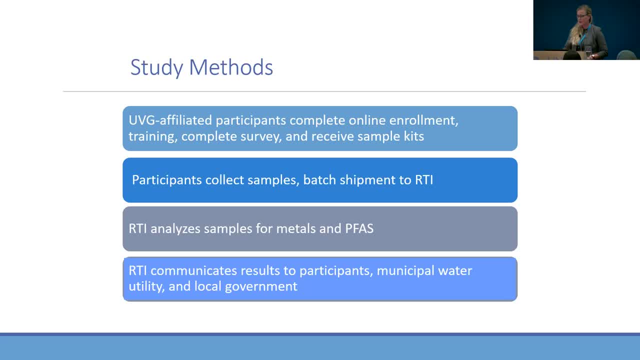 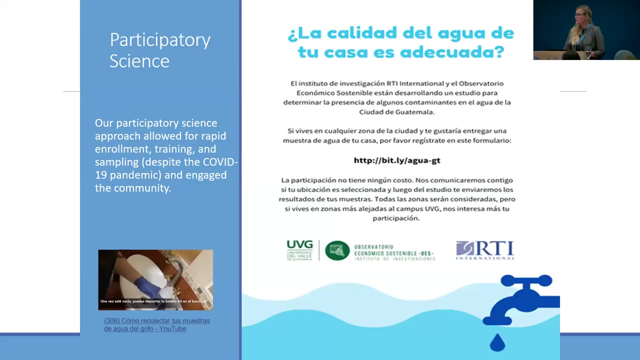 through customs with a cracked kind of ice pack- specialized ice packs- At RTI, we analyzed them and then we after- importantly- communicated the results to participants as well as the municipal water utility and local government. So here's an example of one of the study flyers that went around, and it went around on University. 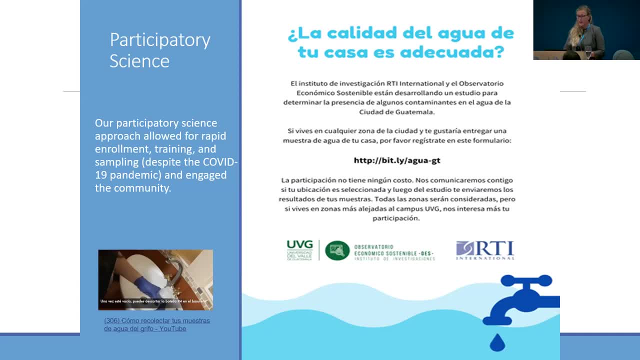 of California TX's list serves and also up around town And our participatory science approach overall all allowed for really rapid enrollment, training and sampling despite COVID-19, and it engaged the community, So it had that value added as well And we didn't need to scrap the project because this separate pandemic was going on. 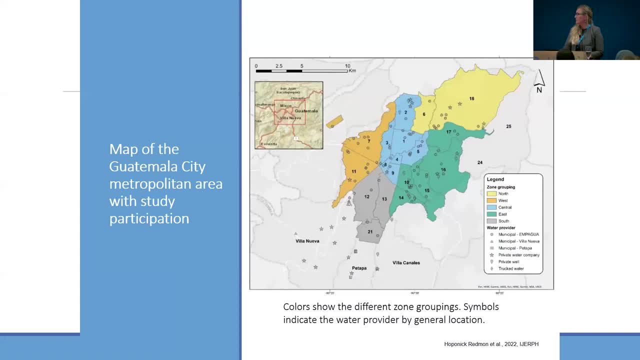 Here's a map of the Guatemala City Metropolitan Area And you can see study participation with the dots And there's a my map here And then we have a map of the Waldorf area. But there's different zones of Guatemala City and those are the numbers and the colors are. 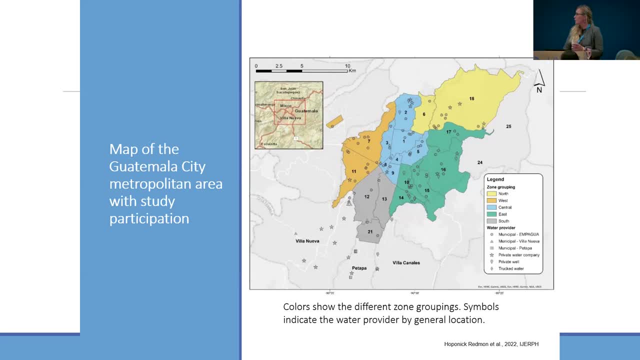 where we aggregated the zones, to be kind of north, south, east, west, for analysis, And we also looked at varying water providers, including municipal water supply, private well water, trucked water or private water companies. So what were our results overall? Well, we tested for 20 metals. 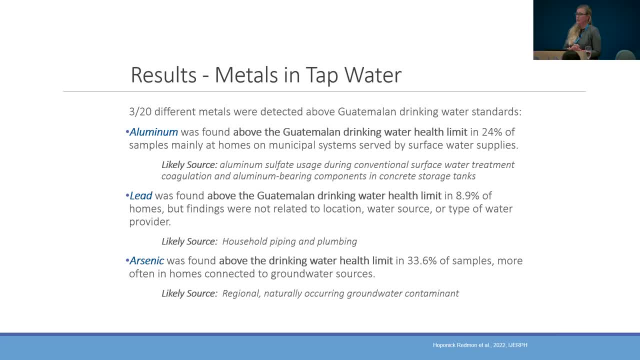 We found that three out of 20 metals were above Guatemalan drinking water standards, which for the most part, match with WHO standards. Interestingly, we found that aluminum was above the drinking water health limit and 24% of samples, and that that was mainly associated with the municipal 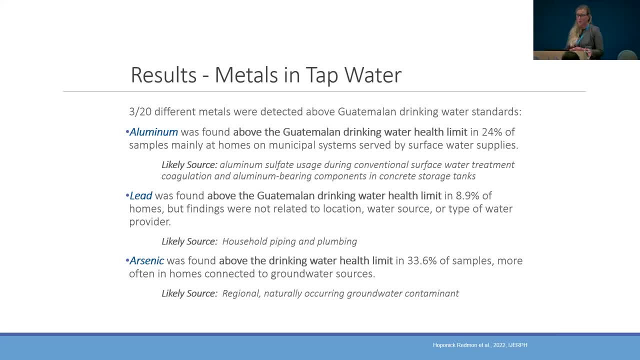 water suppliers using aluminum, So that's a pretty good estimate for coagulation, And it actually was more likely in households that had concrete storage tanks for storing their water during times of shortage. We also did find lead above the Guatemalan drinking water health limit in almost 9% of homes, but they weren't related. 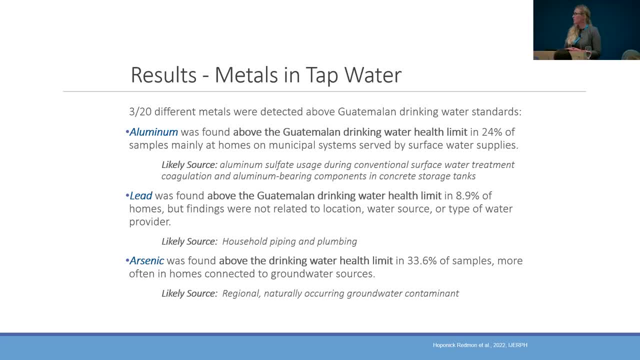 to location water source or type of water provider, telling us that it was likely from individual household piping and plumbing, which we see often in the United States. And so we did find that there was a significant increase in the number of water supply in the United States, and we did find that there was a significant increase in the number of 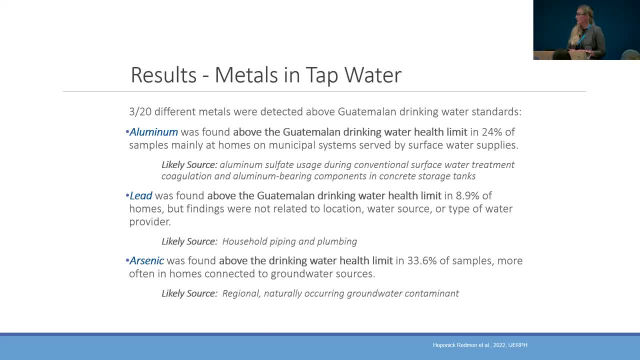 water supply in the United States as well. And we lastly found that arsenic was above the drinking water health limit and almost 34% of samples more often in homes connected to groundwater resources, And that also is not surprising, given the volcanic nature of the soils there and it being a common 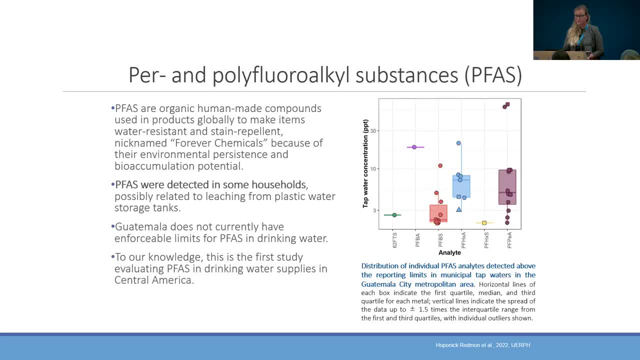 naturally occurring groundwater contaminant For PFAS. so PFAS, you know it's used in lots of products because it's stain and water repellent, But it's mentioned as a forever chemical because of its environmental persistence and bioaccumulation potential. 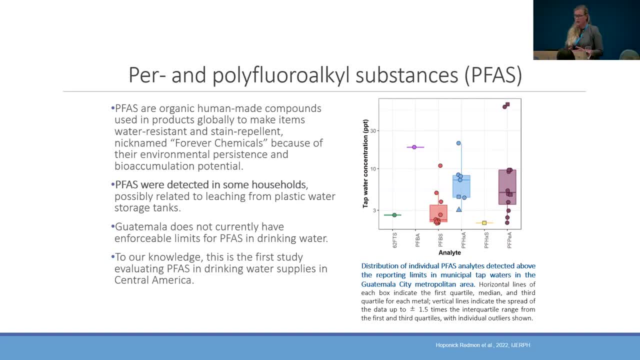 To our knowledge there was no industrial manufacturing or anything like that of PFAS in Guatemala City like we actually have in North Carolina and some areas of the United States. But we hypothesized that PFAS are in lots of things, so we might actually find them. 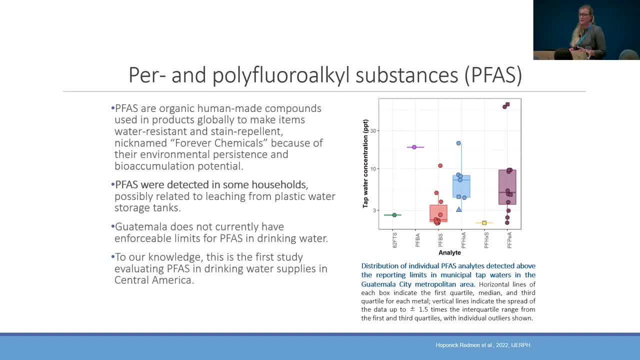 And what we found is that indeed they were detected in some households, likely due to the use of plastic waste. They were not tested in public water storage tanks and it was more prevalent when tanks were stored on roofs outside, So they were getting kind of hot and leaching from the sun. 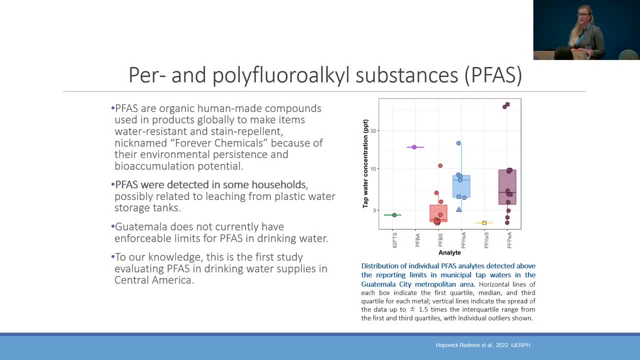 Guatemala doesn't currently have any standards for PFAS, though, And to our knowledge, this was the first study testing PFAS in Central America. You can see on the right some of the PFAS analytes and the levels that we were seeing them at. 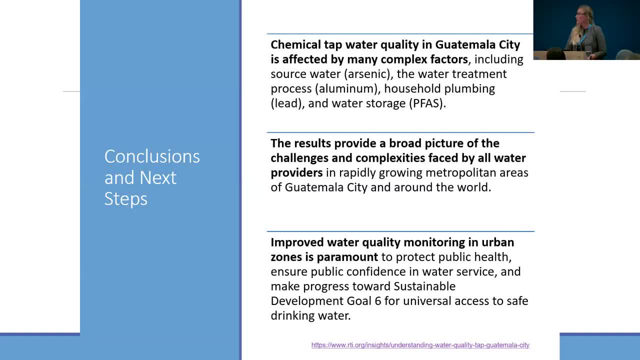 So our overall conclusions are that chemical tasks water quality in Guatemala. you know it's affected by many complex factors, from the water treatment to naturally occurring groundwater contamination, household plumbing and water storage, And the results provided a broad picture of the complexities and challenges faced by water providers, not just in Guatemala City or in Central America, but across the world. 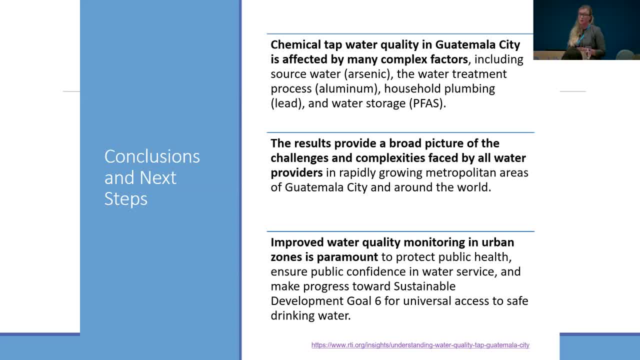 And that improved water quality monitoring and specifically chemical water quality monitoring, Other sites, leftover tillage areas. So all of these things that could possibly土lay the fact that they're for metals and chemicals and emerging contaminants like PFAS, is necessary to help achieve the sustainable development goal six for universal access to safe drinking water. 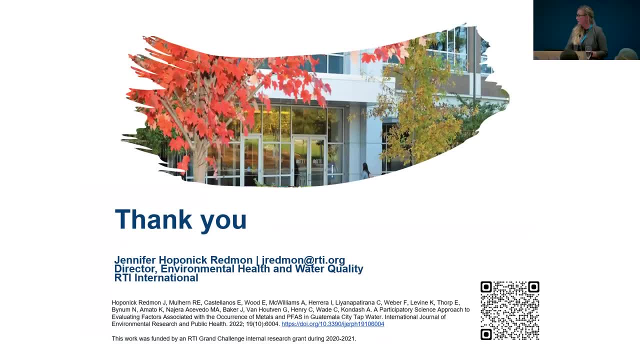 So the last thing I have here is the QR code If you're interested in that article- and that's the name of it on the left there- And you might know some of the folks there, including Riley Mulhern, who came out of UNC and is a co-author. 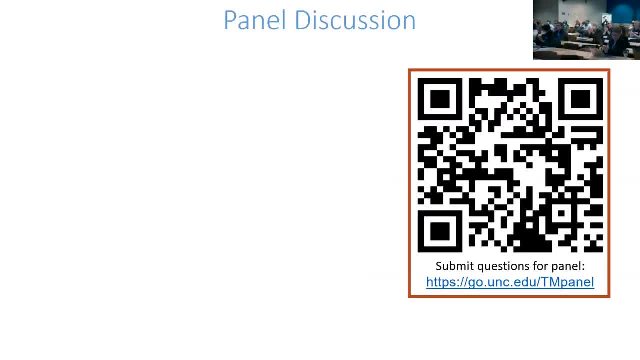 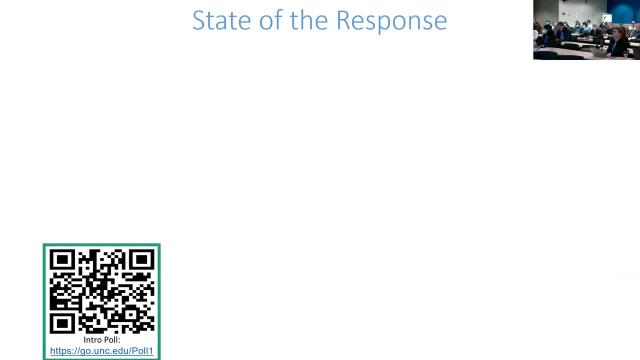 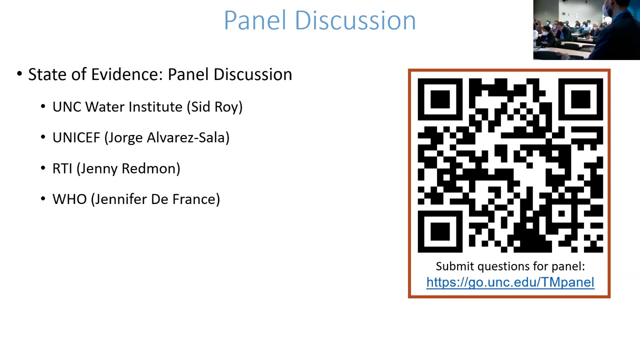 So thank you for watching this first video. Thank you, I think, Jennifer. Yes, it up on the panel and all the panelists want to come up and join the front so we can ask a few questions of everybody and- and we're going to be the speakers that give a presentation so far- and also Jennifer to France, from who is online. 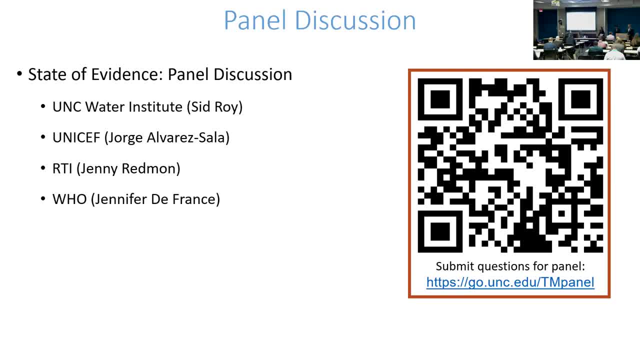 And again the QR code to ask panelists questions here, If you want to be able to get them in the queue. And or Hey, are you still there? Yes, I am Okay, We'll move you over here. so you're hovering above everybody's head. 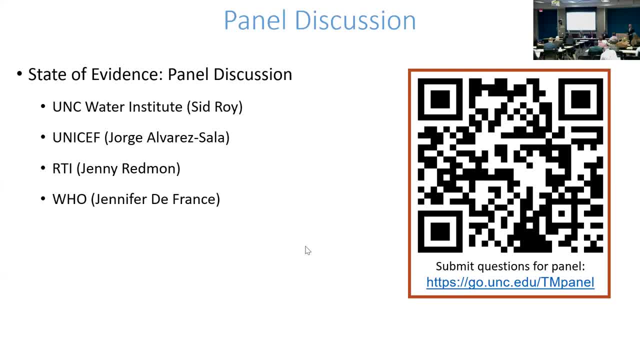 Yeah, Make sure we go to the mic. Yeah, so we'll start, you know, I guess, maybe before we start, you know, maybe I think it'd be really helpful to hear a little bit from Jennifer, who has done a lot of work on this and recently released a technical brief. 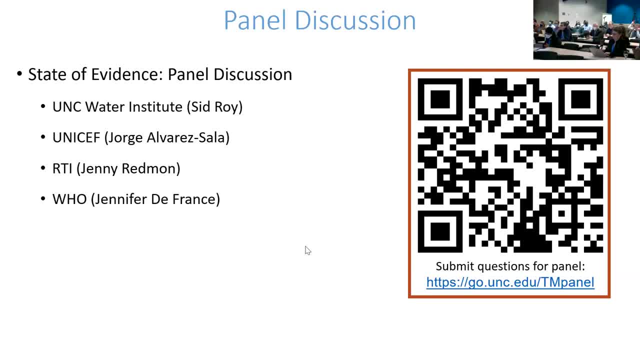 And maybe to kick things off, maybe hear about a little bit of the work that you've done, Okay, And then we can move into some questions. Thanks very much, Dean. so I'm actually supposed to present them the technical brief in the next part of the session, so keep that very brief. but we develop some guidance to support the assessment and management of Latin drinking water, recognizing that it's a complex issue. 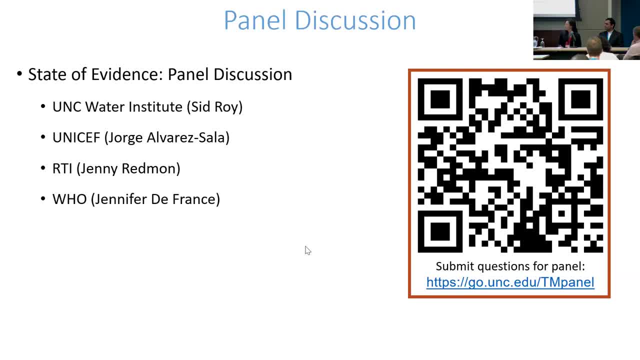 In terms of just what actions need to be done. I mean thinking about This part of the present Part of the session. we're looking at the state of evidence. What do we know? what do we not know? Maybe from who perspective, it's worth highlighting that, yeah, a lot is included in who is drinking water guidelines, as we've heard, and we do recommend that there is some monitoring of lead and drinking water. 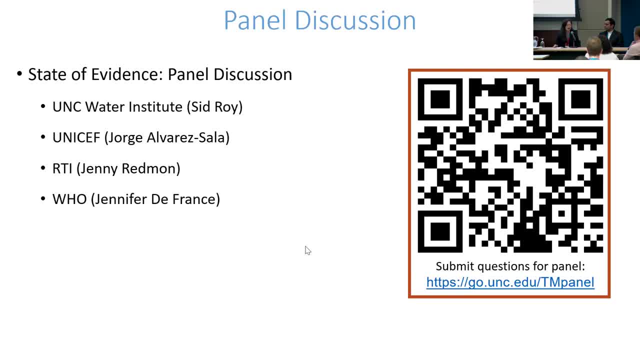 Also, though, as you've heard it from, Often from the material in water supply system and the pipes and household plumbing. So, as part of investigation, we need to look to see, you know, our supply chains, you know resulting in using approved material. 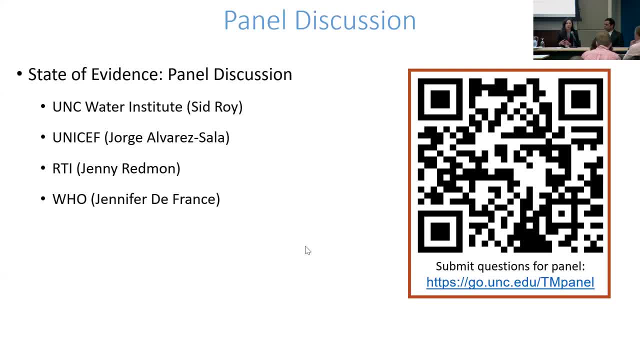 So it's not just about monitoring the actual lead content in water, but it's monitoring the supply chains and making sure right materials are used and installed properly. Thank you for that kind of sneak peek and kind of give some context this discussion. We have anyone in the room who wants to kick off a question and there's a microphone. 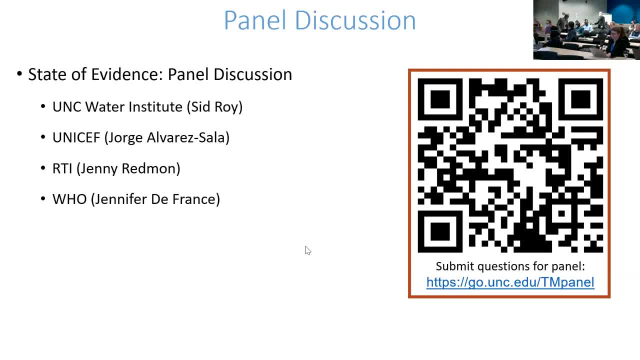 One in the back here and then we can come up next. Thank you. Thank you for the presentations And I have a question for our Jenny from RTI. so, And what challenges? by the way, that's some awesome work, right. what challenges did you face and implementing participatory science internationally and how did you overcome them? 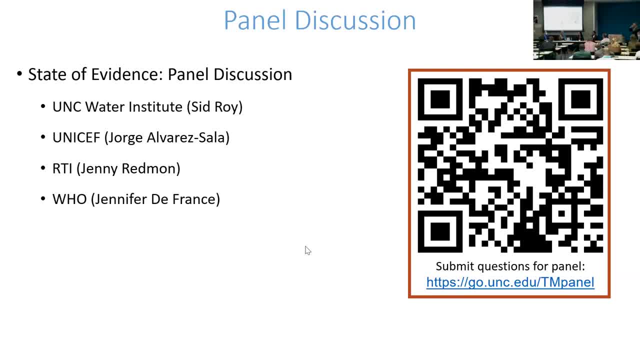 Well, I think the biggest factor is to have collaborators on this. Well, I think the biggest factor is to have collaborators on this. Well, I think the biggest factor is to have collaborators on the ground that want to work and collaborate with you especially. we were actually unable to fly into the country during this period, you know, we could not even fly in, and so we were fortunate. RTI is a nonprofit research institute and actually our collaborator, Edwin, had come to RTI several years previously as an RTI scholar. 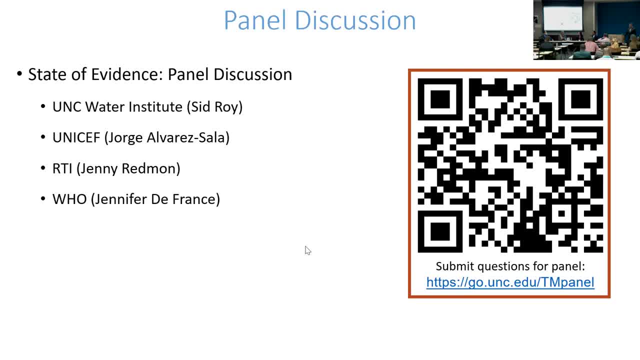 And so we kind of started that networking and collaboration and ethos of what could we do. And so we kind of started that networking and collaboration and ethos of what could we do. And so we kind of started that networking and collaboration and ethos of what could we do together. 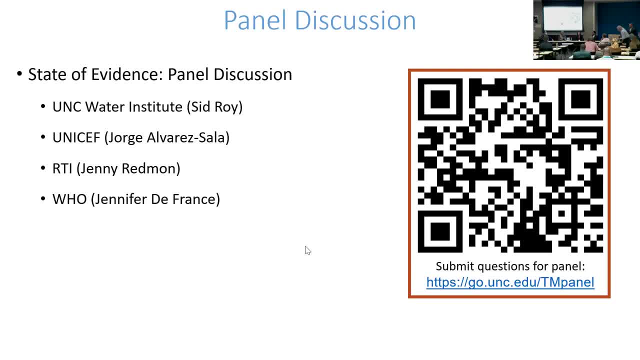 So when we originally had the project idea, we were already going to be doing this when we needed to pivot to relying more on them for actually, you know, receiving the shipment, sending the shipment back, It was easy to do that within the timeframe. Thank you, We had another question. Yeah, Thank you. Thank you very much. Thank you. Thank you very much, and you can introduce yourself or circle you're from and what he was earliest. Thank you very much. And you can introduce yourself or circle you were substitute your project partner, who was artist and what he was earliest: Right. Well, thank you so much for the discussion. 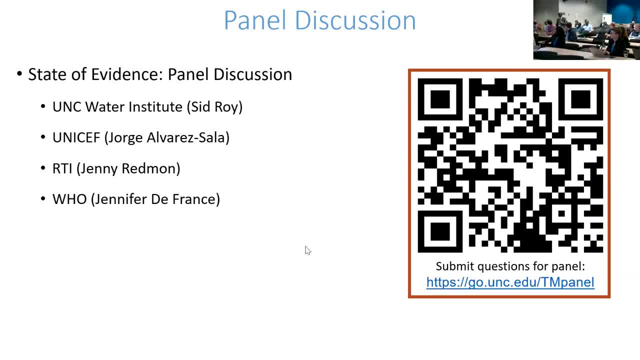 who you're from and who you're with when you're in task. great, i'm bismarck. i'm coming from ghana. i work with one of the public universities, which is amstead, i think, my. it's just a matter of clarification, maybe for context for those that work on bohu and taps in ghana. uh, i wanted to. 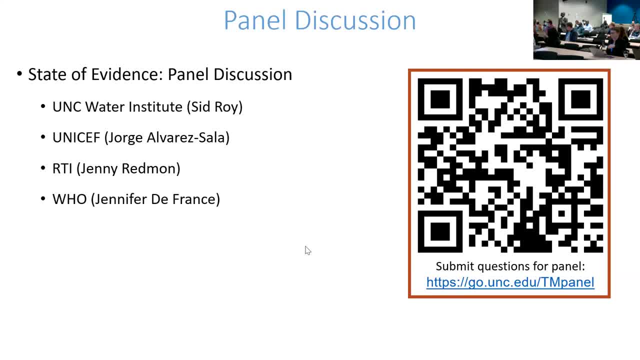 maybe get understanding the taps. when you say the taps, is it from small towns or from utility, which is ghana water maybe predominantly, or from cwc systems or your own reticulated systems? and then i also saw- i think in one of the slides you had india mark two and then, after they've probably 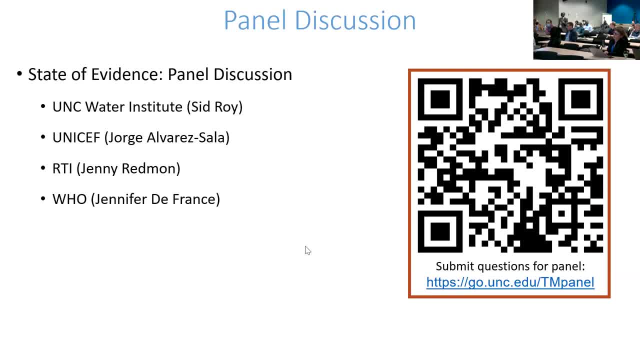 been the main corporates. but uh, did you check with respect to the age, or it was coming from maybe the geology, hydrogeology, always with the parts, which is because of the pumps and therefore the age of the pumps? thank you, yeah, i'll uh respond to that briefly if i can and then if my panels have anything to add. 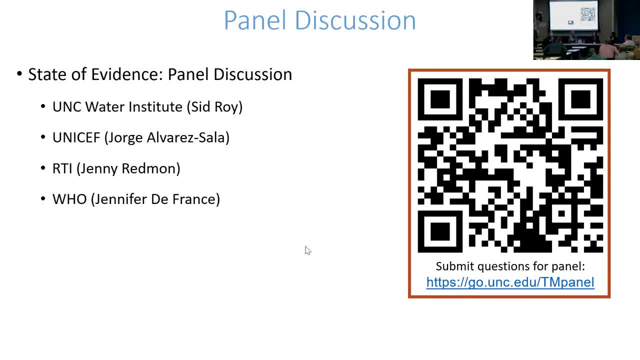 uh the first question. um, these were primarily systems in the north uh in uh four districts around uh tamale right uh, so so in the uh northern region. so these would have been uh under cwsa rather than uh um uh ghana water company and um, i'll mention that um and i think uh uh, my colleague. 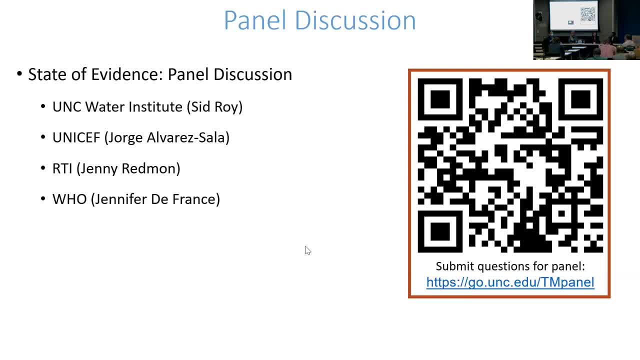 sid mentioned earlier that, in fact, um, when the data were analyzed with respect to the system age, there was no significant effect of system age and also, you know, sid didn't have time to uh uh present all of the results, but when they were analyzed with respect to uh uh geographic details there 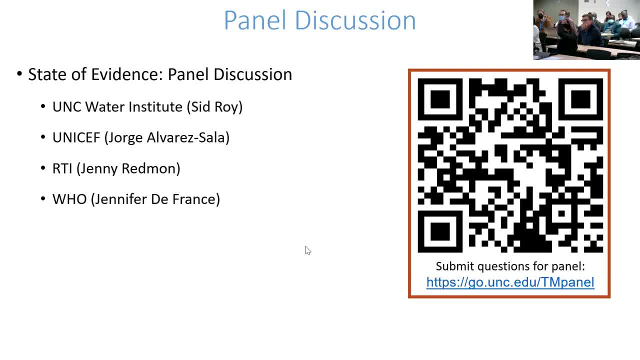 was no significant effect, uh, no significant geographic clustering and, in fact, when the fully flushed samples were analyzed, the occurrence of lead was greatly reduced. so that, combined with the fact that there was a significant association with brass parts and brass parts containing lead above uh current uh iatmo international standards, that certainly was suggestive of an 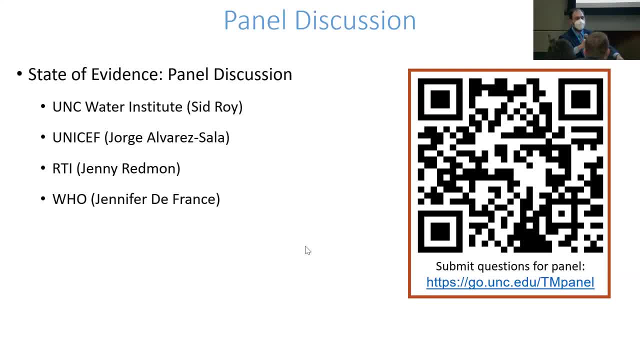 association with unsuitable materials as compared to geogenic sources. if that answers your question, all right. that was a long answer. another question over here. yeah, thanks very much for your presentations. i'm saskinovitsky. i'm a researcher at the university of oxford. my question is for jenny redmond. i was curious. you mentioned 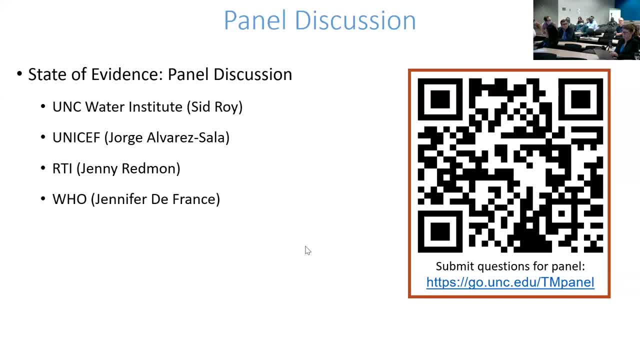 that you shared the results back to communities of your work. could you just say a bit about how people responded, and was there any information about what they might do to protect themselves? sure, that's a great question. so we took a lot of care to provide the results with context. 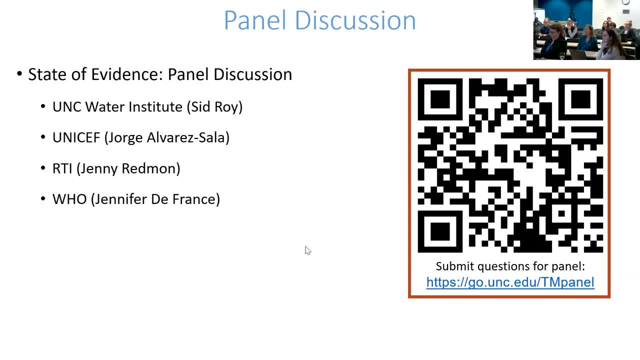 for, first of all, what are these contaminants? what does this mean in terms of any health benchmark? so we used guatemalan standards and international standards, and for pfas, because there weren't standards for guatemala and they're rapidly changing in the us. we took that into account while trying to not overburden individuals, and then we also shared. 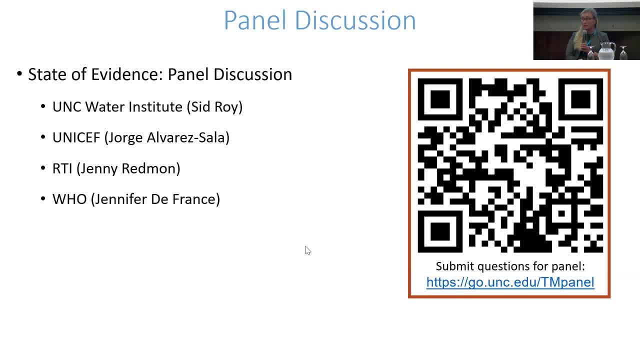 potential actions that you could individually take, which, unfortunately, in guatemala, a lot of the the easiest actions relate to filtering or replacing faucet fixtures for metals, and they had some limited access for purchasing some of these. So we were thinking about: OK, could you purchase a filter from the US that you can't access in Guatemala and would it ship there? 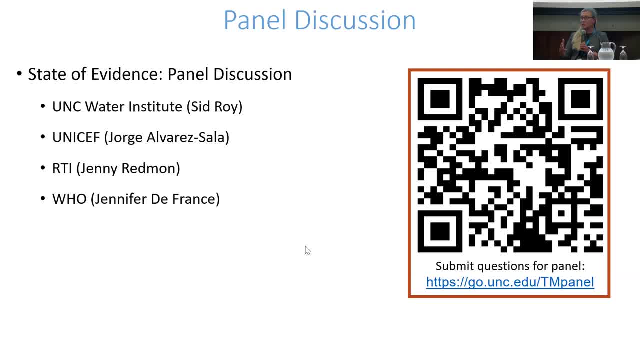 People had those sorts of questions And then, lastly, we also did connect them with how they would put in a response for the government to further look into it. But we also connected with the municipal water supply and the local government. So they knew this study was coming out and we had we held several, several webinars, and then our in-country collaborators were here, you know, in person, in a room like this. 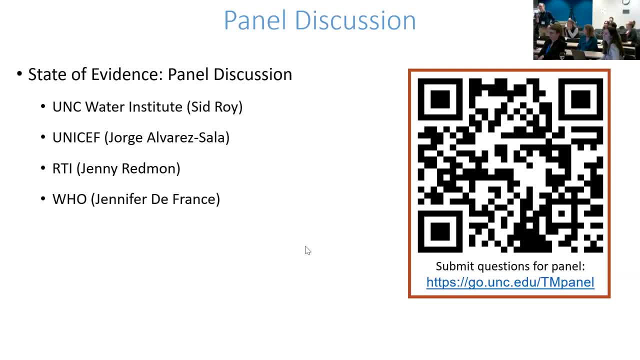 One here and then another over here. Hi, Matt Bentley from USAID Bureau for Humanitarian Assistance. I have a question for all of the panelists, if you're willing to respond. I just want to know, given that we know that lead doesn't have a safe level, 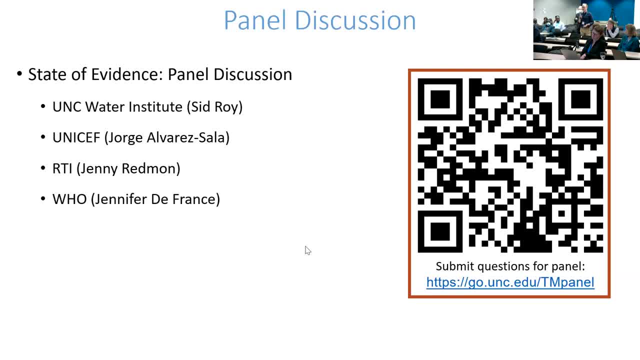 Should we? should we think about Including lead or or any other toxins in the definition of safe water from the perspective of the SDGs? SDGs: I think that's a good question And one thing to point out is SDGs, you know it's for global comparison. There's some limitations with that right. It's looking at arsenic, looking at fluoride, microbial parameters. 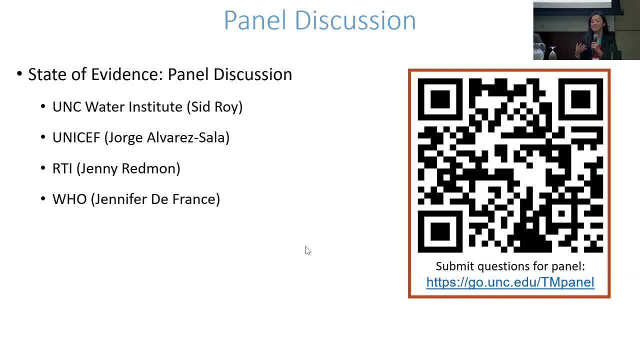 You know, I think for WHO, the biggest thing for ensuring safe drinking water is risk management. you know, to prevent contamination and making sure you address the priority risk, and that's not covered as well, And so I think we need to be pragmatic, in that you can't cover everything. 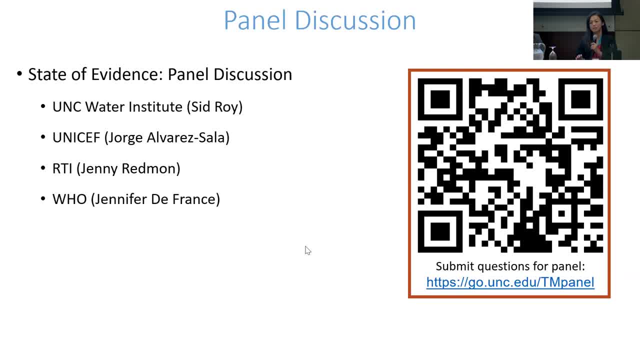 So there are certain things and the SDGs also. they're supposed to be tailored for the national context, of course. for nationally, Countries should make sure All priority contaminants are considered in a prioritized manner. but for global monitoring, I think I'm not sure about the resources with that. with with lead, I mean it is priority but that's a lot of resource implications for requiring lead. 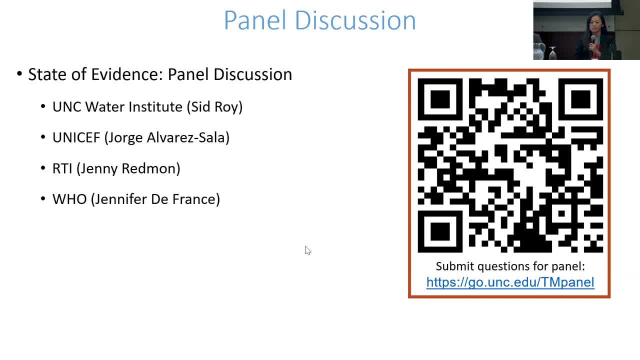 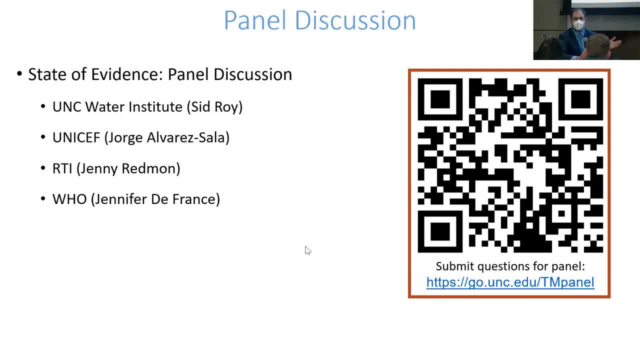 Yeah, in fact, I'm going to take the host's privilege for a second and just add to that. Anyway, there is JMPS active to track globally, going forward based on data availability, And so I think you rightly made a distinction between those two in terms of. 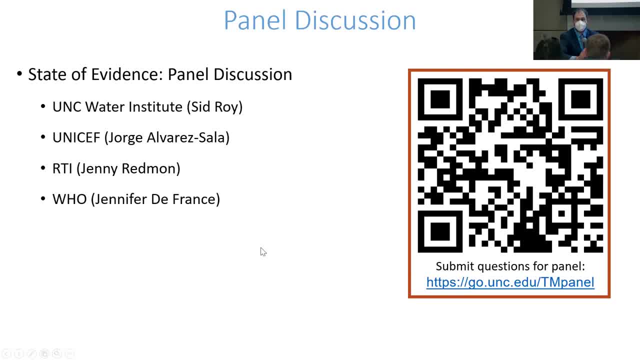 hey, were their opportunities for prevention right now to have massive benefits to populations separately? where do we have data to monitor things globally now versus in the future? But knocks back to your question One of the things: so there's some wonderful students doing a systematic review of 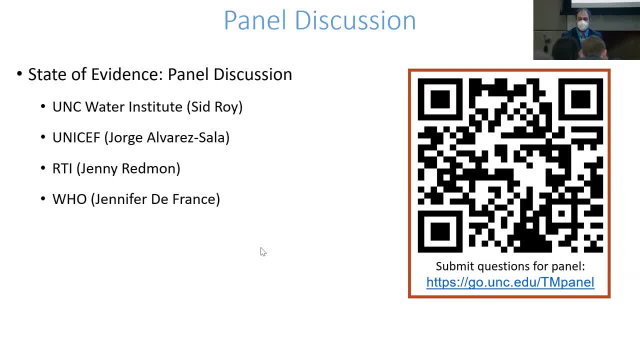 lead toxic metals in drinking water in low and middle income countries, And one of the things they're doing is taking a look at the methods that are used, And these are overwhelmingly currently laboratory methods in high quality studies, primarily ICP-MS and others, for 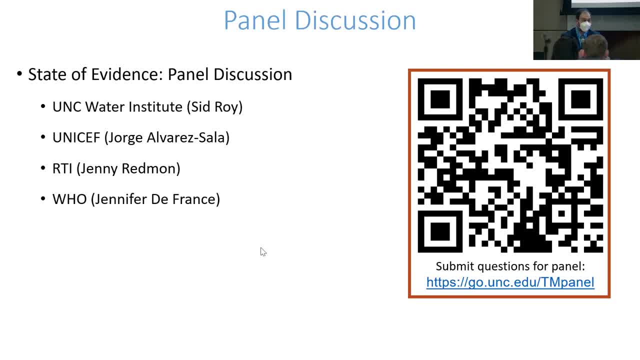 you know if we want to know about part per billion concentrations. That said, shameless plug. some wonderful students have developed a free, open source app that takes those presence absence LFIA test strips and gives you a semi-quantitative interpretation for screening, And that's nice. 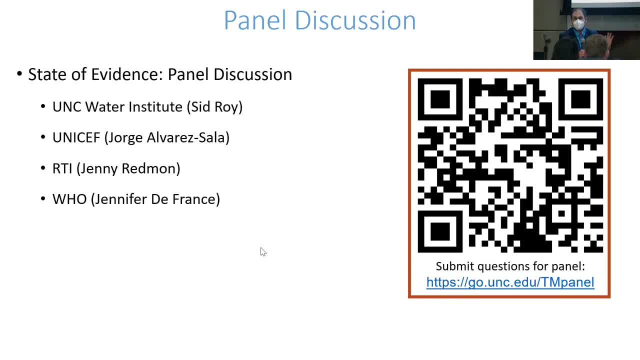 because those test strips are 10 bucks each give or take, And so, to the extent that you get good enough field-based screening data, it answers a different question than robust ICP-MS data, But in terms of field-capable methods, that's one thing we're very interested in And 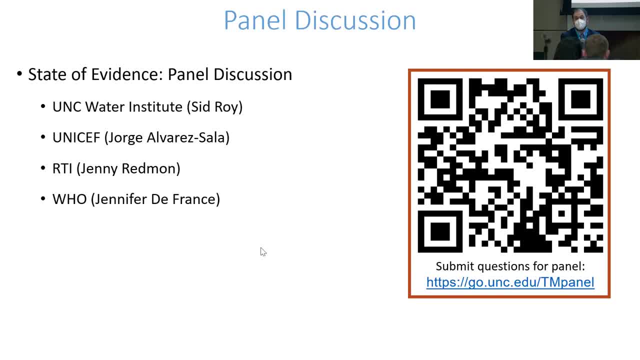 I'd love to give you some of those strips and the QR code to download the app and see if that's useful. There's a question over here. Oh, yeah, her. and then over there. Okay, Hi, my name is Katya Cherikomeli and I'm a researcher from UC Berkeley. 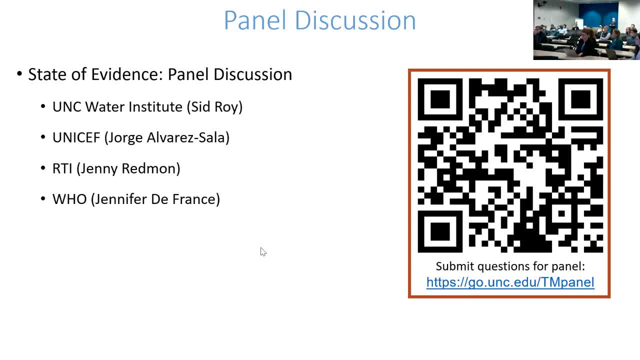 I have a question for Jenny from RTI. So in your talk I was really happy to see how comprehensively you thought about the RTI And I think that's a really good question. I thought about the chemical risks from not just the source but the actual treatment process. 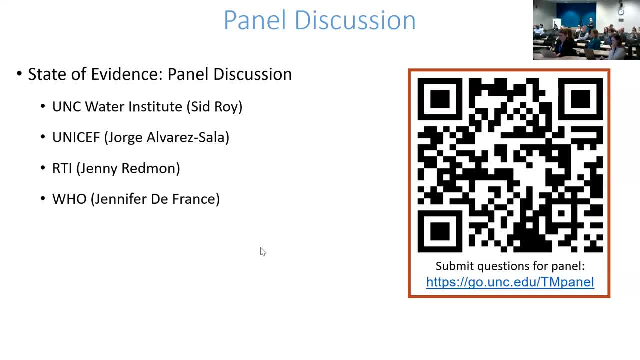 the piping and, at the end of the day, the storage, which is very common all over the world. So I wanted to hear your thoughts on thinking about the chemical risks associated with concrete tanks versus metal tanks versus plastic tanks, which are all so common. Which ones would you? 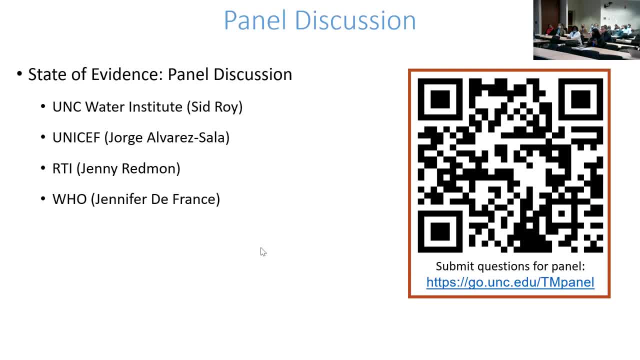 prioritize in terms of thinking about spreading the message or worrying about the concerns of the risk exposure? Sure, That's a good question. Well, first of all, so we found that PFAS was related to plastic tanks and arsenic related to concrete tanks. We found that tanks that were outside were more likely to contain. 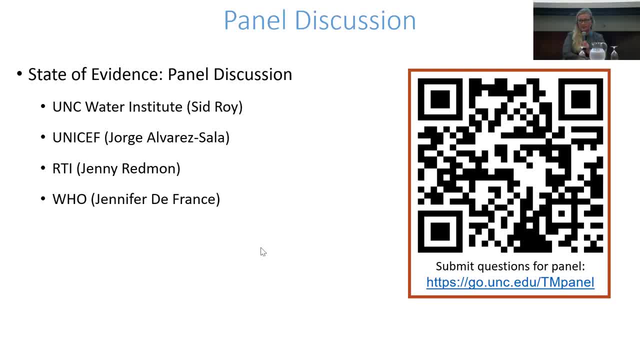 contaminants And that makes sense from a temperature, sun kind of bleaching perspective. So I guess if you were going to recommend something, trying to store it in a shadier or a cooler area, That is better. There were individuals that had tanks on the ground compared to on a roof, or if 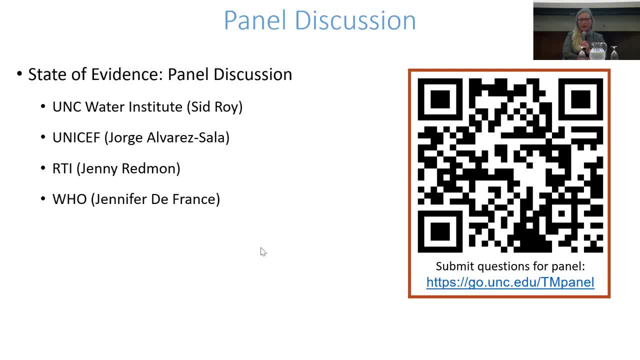 it's on the ground, under a tree or something like that. But then the plastic tanks. they're not technically supposed to have PFAS in them, but it's likely. from hardening the tanks, that fluorination process is inadvertently probably creating PFAS. So that's something that's a. 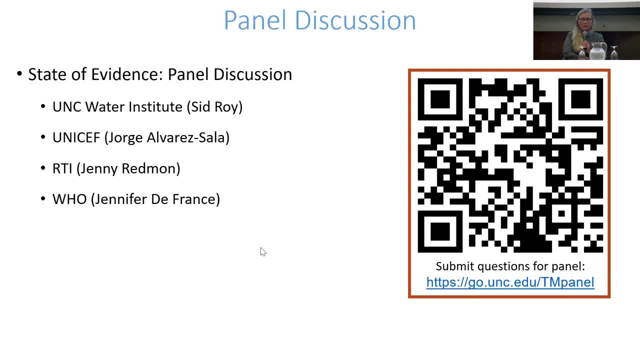 future area of research For metals. what we would love to know more about is how often the concrete tanks were cleaned, Because in general it appears that they're not clean very often And probably you're continuing to kind of use the water off the top and you're getting the sediment, but there's some mixing happening And our hypothesis 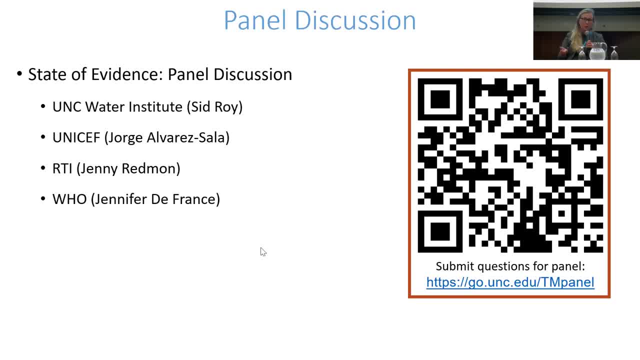 is: maybe if you clean those tanks out more frequently, maybe there would be lower arsenic, because the water for the same water source without a tank was lower arsenic levels than households that had a tank. Just to add to that, really quickly, I think it's important to point out that not all materials 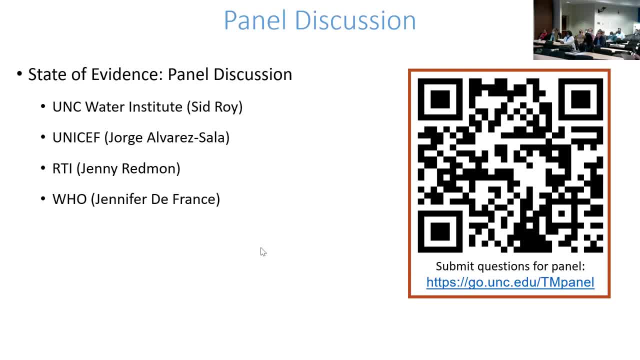 not all plastics are the same right And not all materials are the same, And I think the critical point is you need to make sure that you use materials that are appropriately certified. you know that are considered appropriate to use with drinking water. 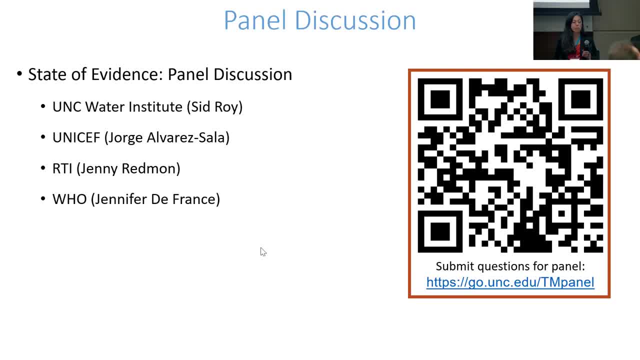 Thank you. My name is Diana Kesiga. I'm working with the Uganda Sanitation for Health Activity funded by USAID. My first question has been answered. It was around the PFAS leaching into the water because of the plastic tanks I was looking out for. 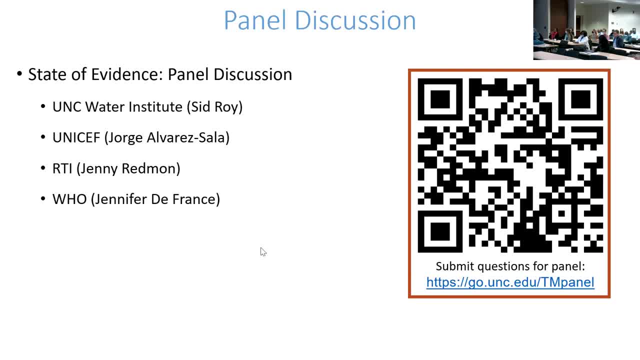 recommendations on where best these can be installed from an implementer's perspective. And then on the aspect of aluminium: is it because the concentration at treatment point is not accurate, Or is the storage of the water contributing to the higher concentrations? Thank you. 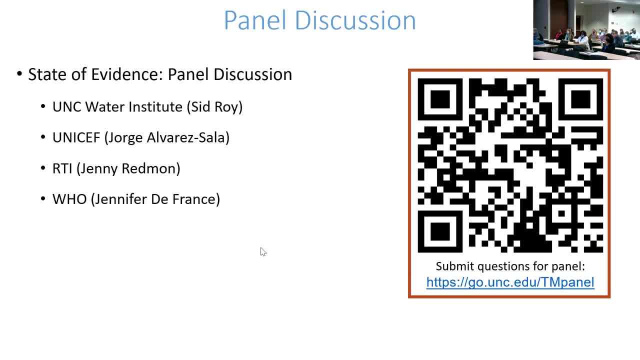 Just regarding aluminium from, I think, the WHO guidelines perspective. So just to say that WHO has a health-based value for aluminium, but we don't consider a guideline value because for operations for coagulation you should be able to go below it, So I wouldn't be surprised. 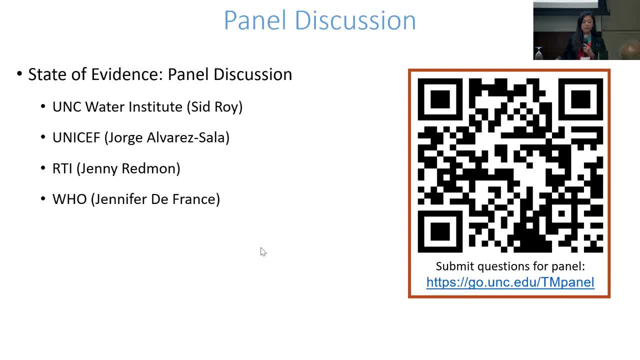 then if higher levels are being used in the treatment. But I think it's important to note that the higher levels are being used in the treatment plant and that's what's causing the higher levels, And what we surmise is that there were higher levels than necessary at the treatment plant. 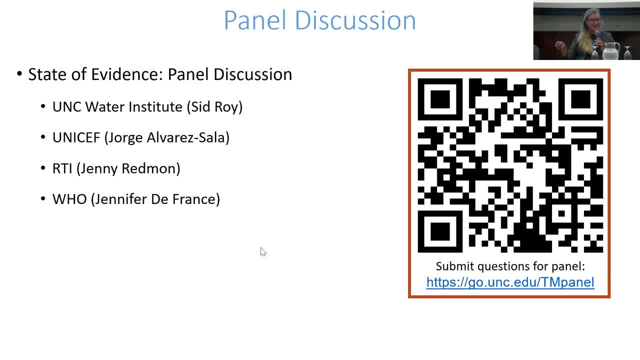 and the treatment plant didn't have funding to test at the tap, And so they'd actually never known that they were actually probably overdosing at the treatment plant. So this was the first time for them to be able to get that information, And I assume they're taking that into account, and 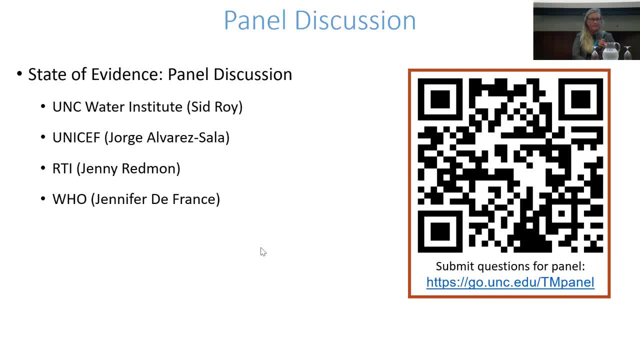 potentially changing what they're doing. So that's a good question. Thank you For the plastics you asked. honestly, there needs to be more done on that to try to identify it, because similar to there being limited filters available that are certified in Guatemala City. 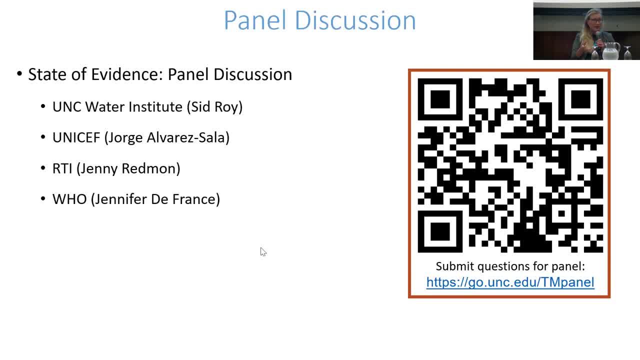 people are just getting tanks that they have, that are available to them, So they might not be understanding what their risks are. Thank you, We have one more question Then we'll close out with a wrap-up question and then we'll move on to the panel. 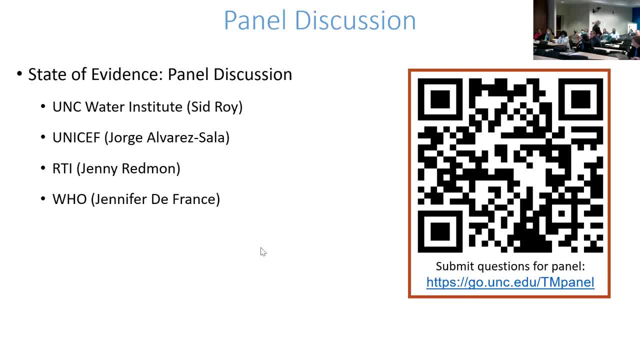 Hi, thank you. I actually have a follow-up comment to the last question about aluminum. So my background for my dissertation work was on fluoride removal, So I studied a lot about aluminum chemistry And one of the things I wanted to bring to your attention when you're. 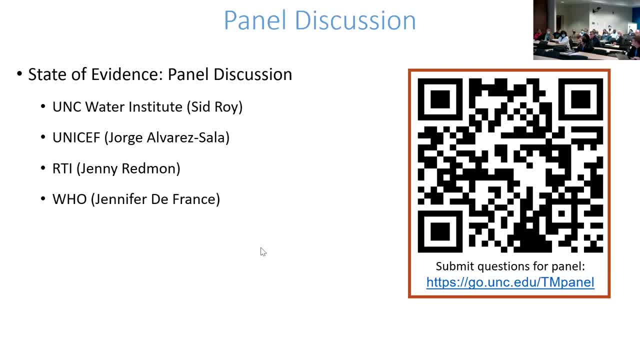 doing future surveys? is that also to look at the use of activated alumina as a water treatment method, Because in my experience it's actually quite soluble and we're using it all over the place to target particular chemical contaminants and also as use of the? 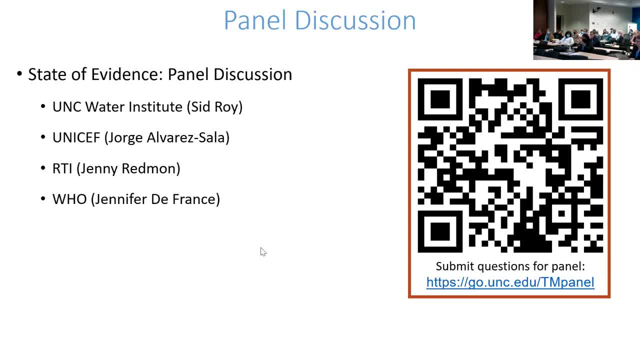 tässä it as a desiccant, And this material is definitely above WHO guidelines in many of the experiments I did, even at low dosing. so that's an alternate potential cause. Well, thank you for all your questions. I have one closeout question that maybe 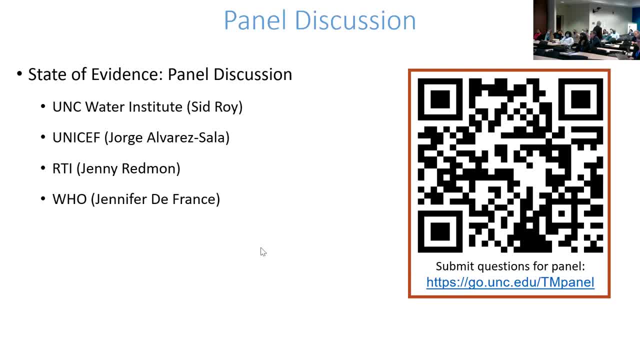 if you walk your answer now or maybe to World Vision to talk specifically about hand pumps. But one of the questions that just says can you discuss more about This is from an online submission. It says: can you discuss more about the hand pumps? that where lead was found, were they the? 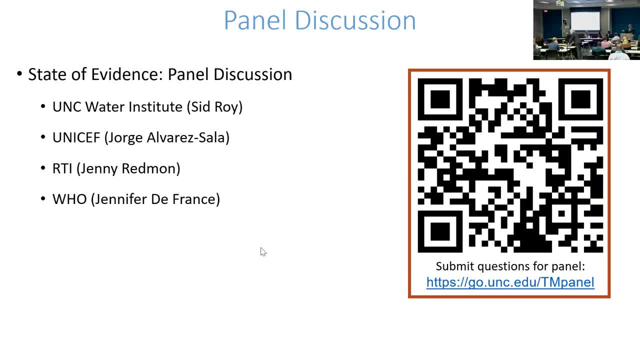 original pieces, replacement parts, etc. so if anyone wants to talk to that now- and i know world vision would have something as well- yeah, that's a great question and uh ray has more to add to that. what i will say is my recollection is we didn't have the data to disaggregate that. um, that said, the 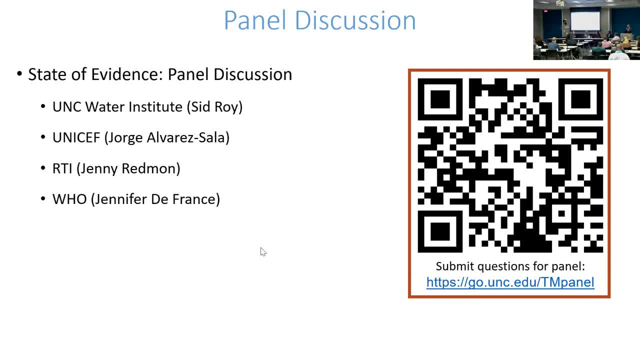 lack of correlation with aid. it would seem to suggest that, uh, it would be surprising for it to be just original parts or just replacement parts and for there to be no association with age. but we didn't have, i don't recall that we had sufficient data to disaggregate. 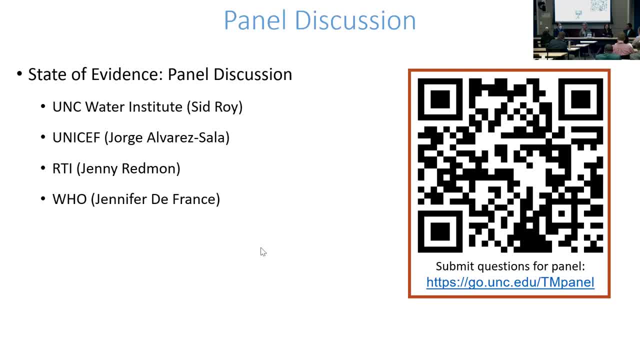 um, but we may know more and separately, um, you know, world vision can speak for themselves, obviously, but are continuing to uh, uh invest in generating more evidence to better understand uh occurrence and prevention stuff that we'll hear more about. well, thank you all the panels. we can give a round of applause. we will now move into the next. 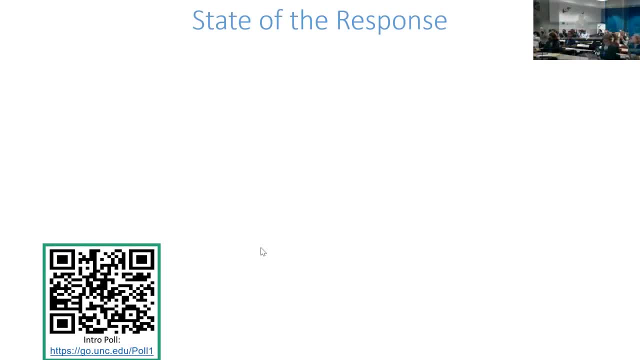 portion. the next portion of today is: we're going to have the state of response, so we're going to hear from these some- some of the same organizations and some additional ones- on how they've responded to these findings. you know where this is an issue and what. what are people doing about it, and so we 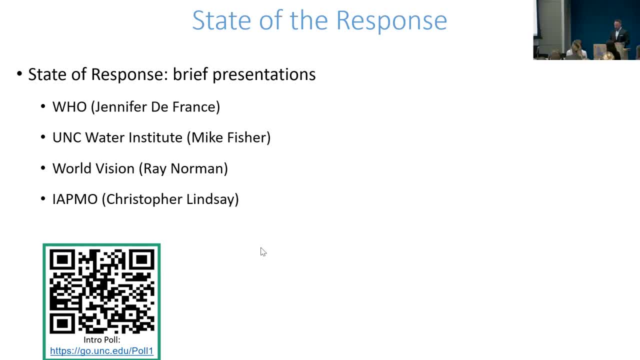 will go down- start with uh, jennifer, and we will work our way through the presentation slides and we will go down and then we'll talk about some of the things that we've heard from you and then we'll move on to the next slide deck. there we go. 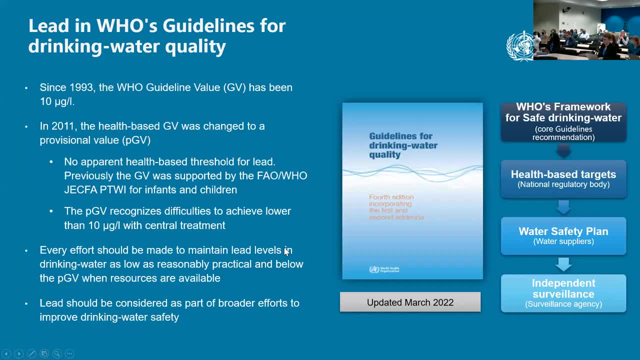 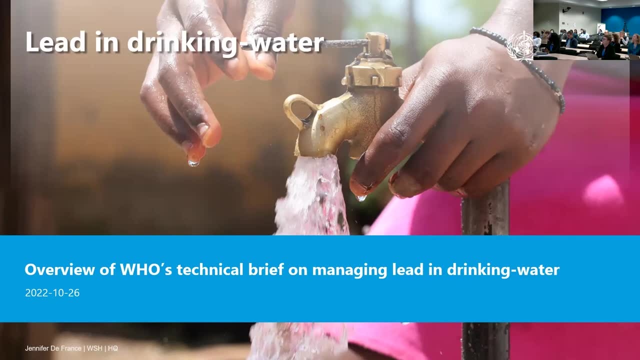 whoops, should i get him out right in the middle of your slides? thank you so much, dane. so now i'm going to give the overview of this technical brief on managing lead and drinking water that wac has shown us will be coming up in the next few weeks. 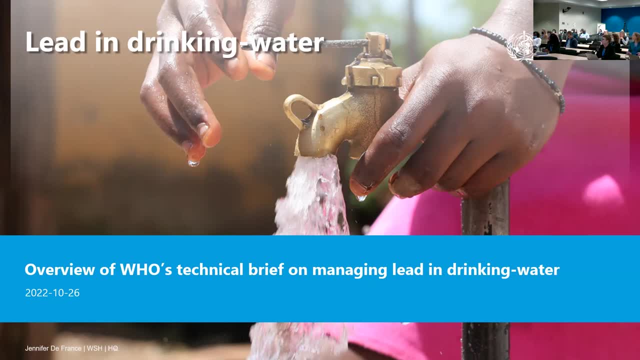 so now i'm going to give the overview of this technical brief on managing lead and drinking water that wac has shown us will be coming up in the next few weeks. WHO recently published- I have just a few copies. I'll just show you guys what it is. 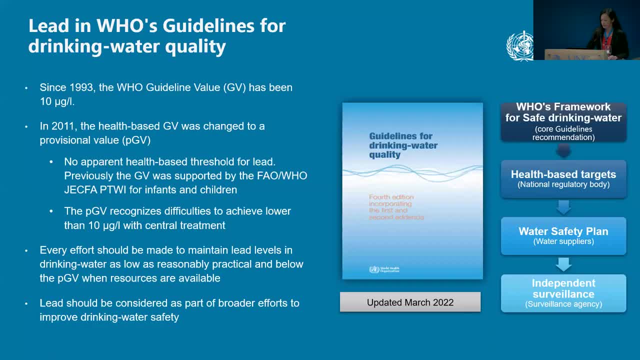 So before I actually get into the overview, I wanted to give a little bit of context, but we've gone through quite a few points already related to the background, So I'll just go through it really quickly. But one: I just wanted to remind people here that right now it's International. 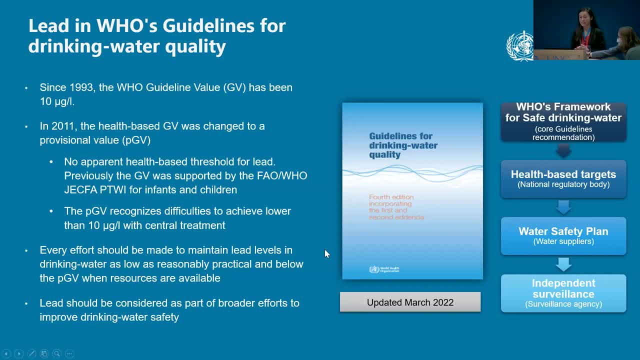 Lead Poisoning Prevention Week. That's the 10th year for this event And so WHO, more broadly, is doing a lot of stuff on lead with campaign materials and really reminding people that we need to address lead to protect public health. So we heard a lot about the guideline value. It's 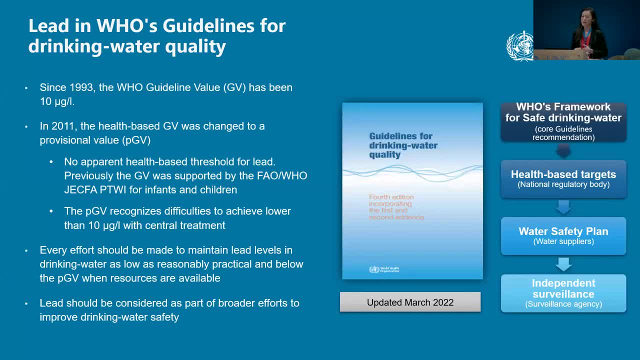 not health-based. I'm not really going to get into that, but just to say that this level of 10 micrograms per liter, it used to be health-based but it was retained and considered provisional, recognizing it's very difficult to get below this level where lead materials are used in water. 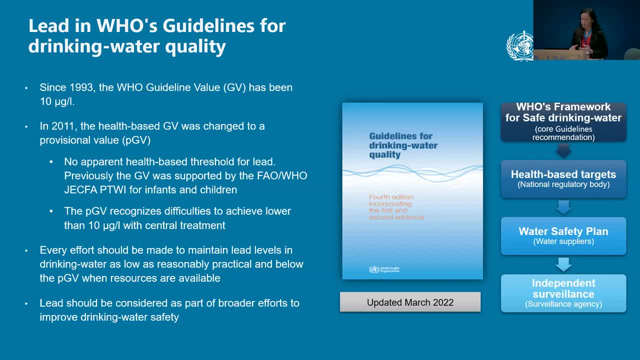 supplies. And so with that, because Sorry, Sorry, what was that? No, I don't have it on the right side. Okay, no, No problem. So with that, if countries can go lower than 10 micrograms per liter, they should. 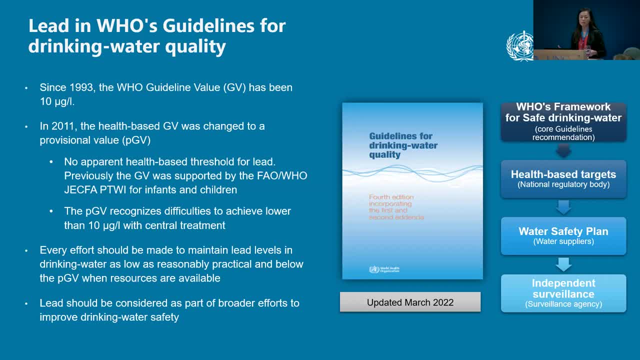 But also we need to keep in mind, as we mentioned, lead is one of several priority chemicals, So we need to consider lead within the context of all risks within a water supply system, using a preventive risk management approach to identify the most important parameters and to manage those. 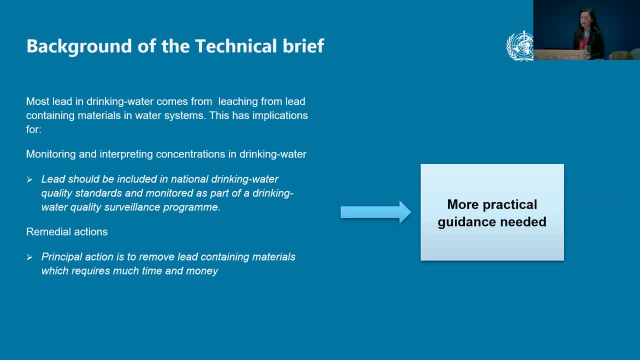 priority parameters, Because lead is mainly found, you know, in the transducer. So if we're talking about three-to-four milliliters, but if there is a sign of lead, then we have to monitor what's in the water. So I will say that 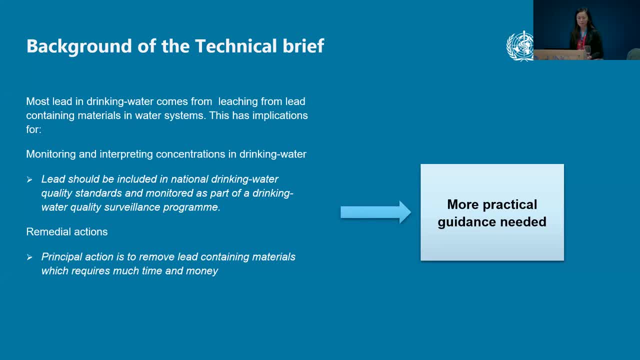 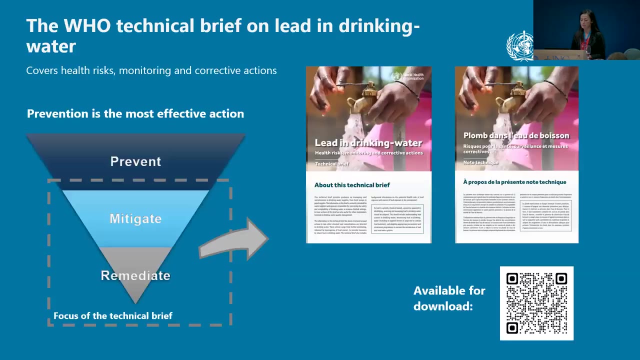 the most dominant source of lead in drinking water is from lead-containing materials. This introduces service lines from lead-containing materials, So this really has implications for the management And because of this, because of this complexity, WHO developed some guidance to support the assessment and management of risks. So this is the technical brief I mentioned Just this week. 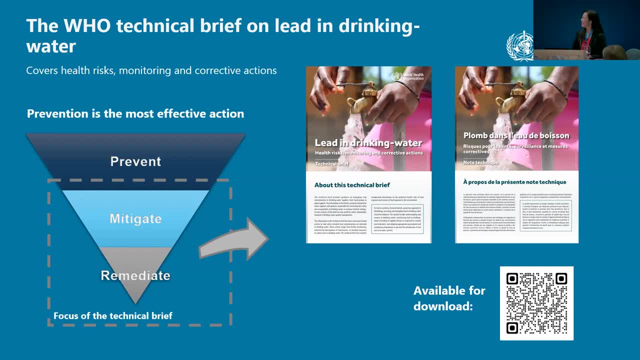 we published the French version of the guideline, So yet another QR code for you guys to download this technical brief, And on this website there's also information and materials from the International Lead Poisoning Prevention Week, And so I encourage you to look at those materials. 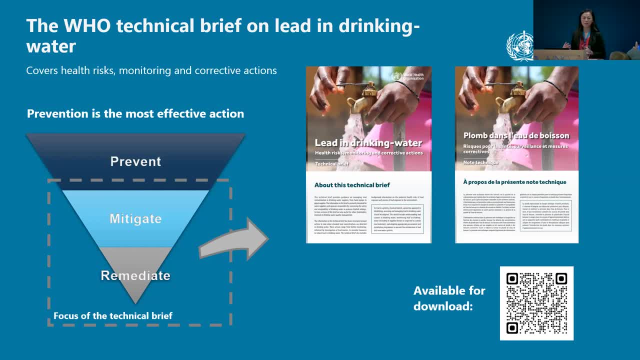 So this guidance was really developed when we got questions from member states asking: what do I do when there's lead in water? What actions do I need to take? So it's really structured around: what actions do you take when you find lead in water? But having said that, 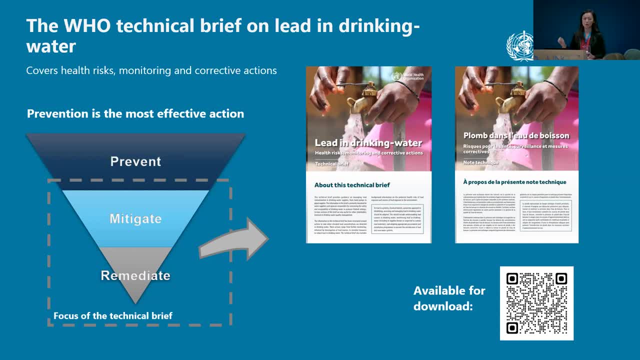 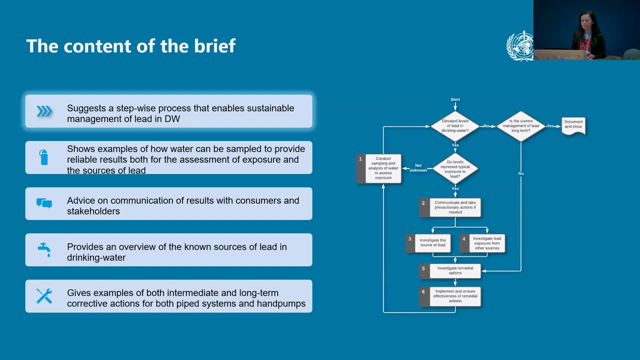 prevention is the most effective action. So it's not to try to de-emphasize it. It was just the angle we were taking With trying to provide practical guidance, But clearly we need to ensure prevention moving forward. So, just very quickly, here's an overview of the contents of the brief. As I mentioned, 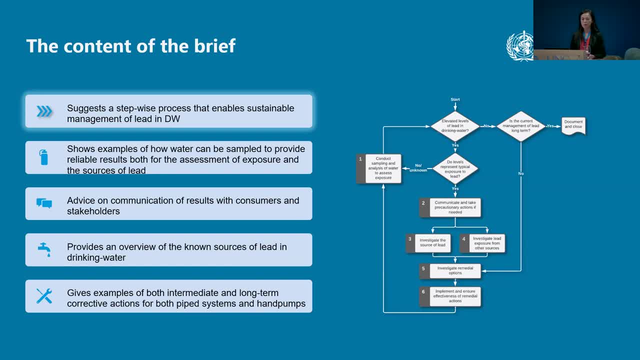 it's really aiming to provide practical guidance when you identify lead in water, And it proposes six key steps to undertake. when you identify lead in water, The key message is: you shouldn't just panic. What you need to do is you need to take a systematic approach to really understand what 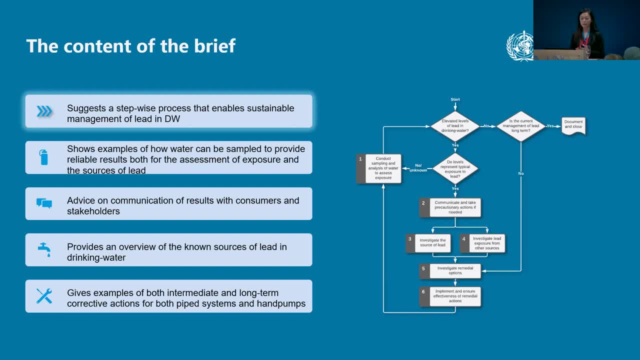 that lead concentration in water means to better understand that in terms of exposure for the populations, in terms of the sources, and then take actions to address progressively the lead issue in water. There's also information about the sampling and considerations for monitoring lead in water, because of the complexities I had mentioned before about what does lead in water. 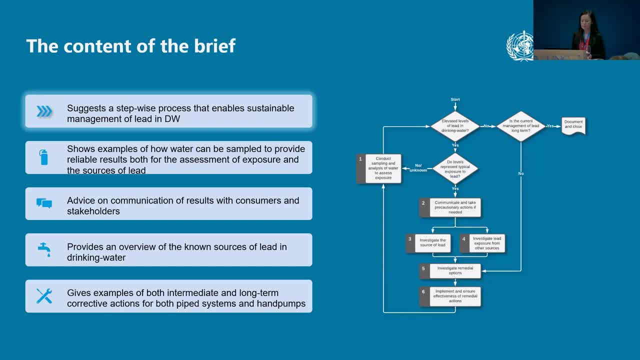 actually mean. There's a lot of stuff around communication, There's information about the different sources of lead from the different types of materials that contain lead, And then it gives many examples of what actions can be taken to address lead in water, from short-term measures to more longer-term measures. So I'm just going to briefly go over. 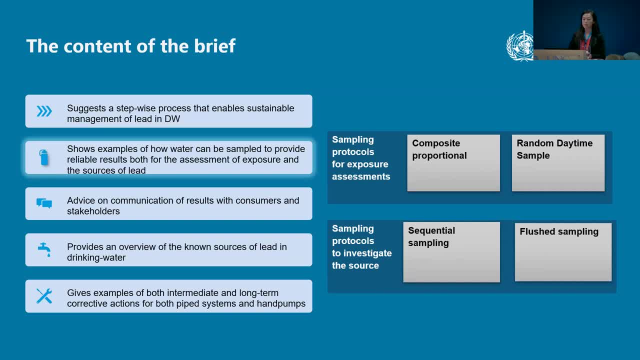 some of these. In terms of the methods, I just want to highlight that we saw in the first presentation just about different sampling protocols that you can take, And so there's an overview of the different protocols that you can take, And so there's an overview of the different. 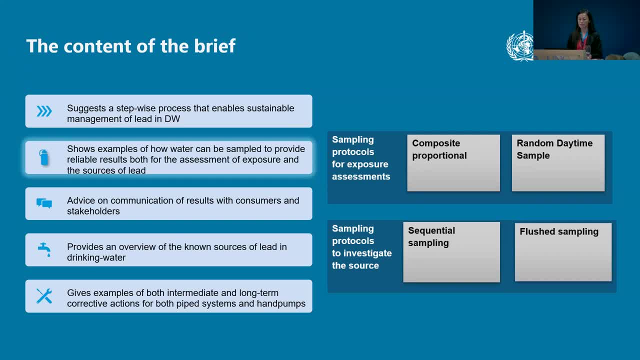 protocols that you can take, And so there's an overview of the different protocols that you can reach for exposure and understanding source and source in there. but also you need to consider when do you take the samples, How many samples do you take, How do you take the samples, et cetera. 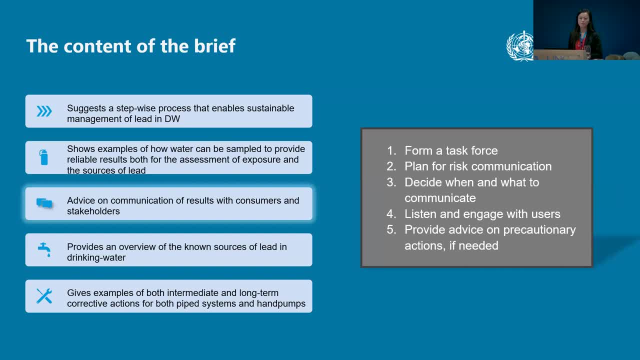 And so there's guidance around that In terms of communication. it's a very critical part of this lead issue in water And I think that really the key message is that we need to communicate on lead in drinking water, need to take a proactive approach addressing –, talking. 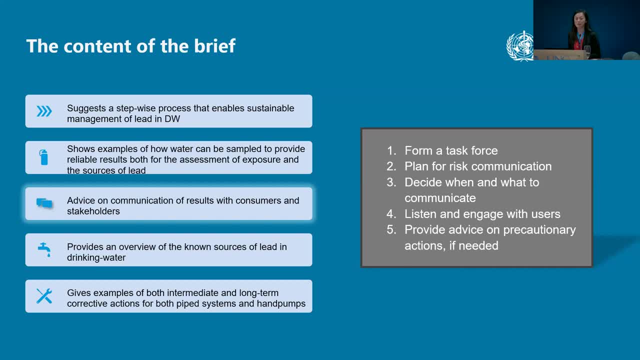 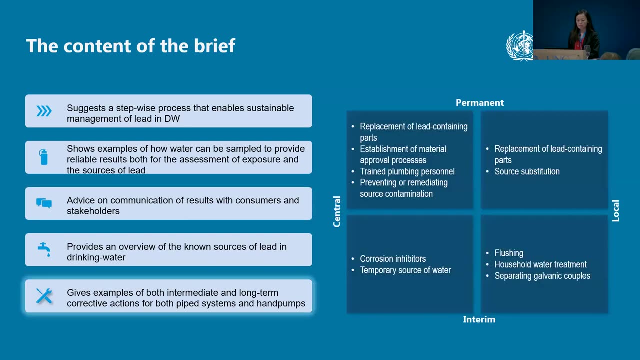 We're talking about it with the government counterparts, talking about it with communities that may be potentially affected, being transparent about the results, being proactive about what actions can be taken. So it's really great to hear the example from Jenny with the with the communities in terms of action. 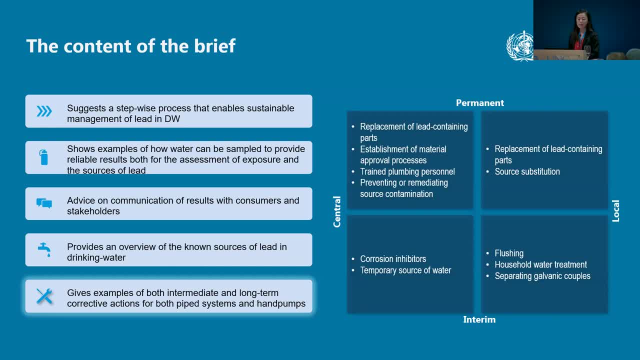 So we heard already a little bit about certain actions to be taken. Ultimately, as I mentioned, we really want prevention. We're talking about using low lead materials. we're recognizing that that can be a very expensive and long-term process. That doesn't mean that you should not be taking action, and there are many actions that can be taken to mitigate Latin drinking water. 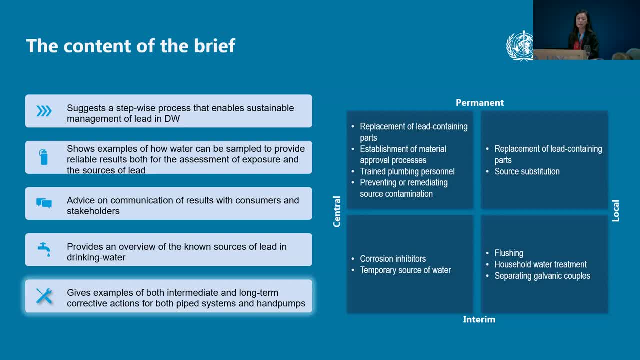 Maybe not to below 10 micrograms per liter because of issues with reducing it lower than that when it's in the materials. But you can. you can do several things. that again we heard from the others about flushing, about using filters, etc. So just to flag that: 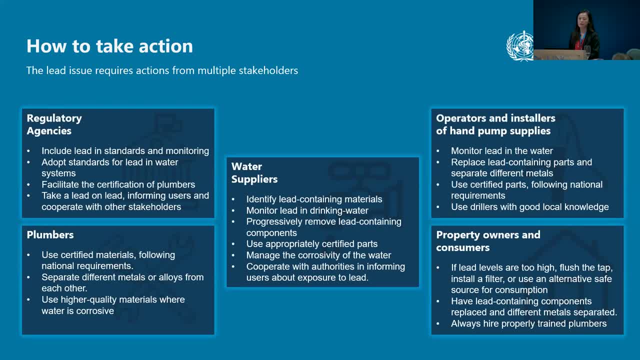 There are different actions that we can be taken. We also present in the technical brief based on what actions different stakeholders can take And this really wanted to flag this, mainly because I think lead is unique compared to other contaminants and that it involves a wider variety of stakeholders. 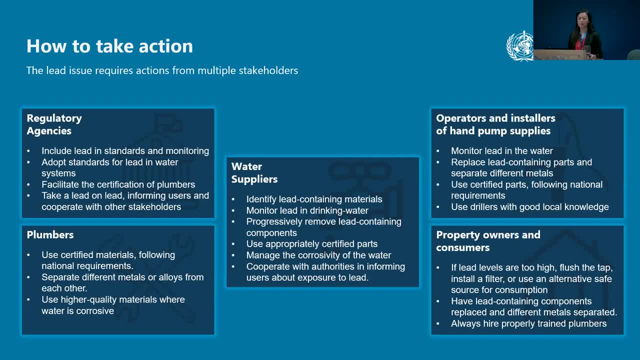 We're often, for example, lead could be in the building. so you need to involve the building authorities, You need to involve plumbing authorities and plumbers, as well as the health authorities. Hearing from from Jorge Ertz, Jorge, earlier, how you know, ultimately comes down to health, and so we need to think about all those exposure sources of lead. 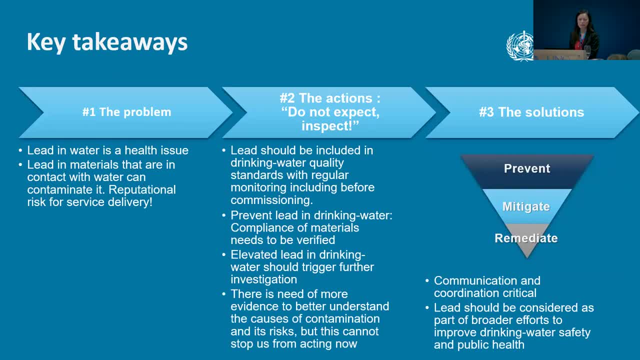 So just a few key takeaways. Actually, the really the key message I want to make is again, when there's lead in water, We really are advocating to take a systematic approach, to understand what the samples mean, to understand the exposure and source. So this whole thing about this is data You're collecting. 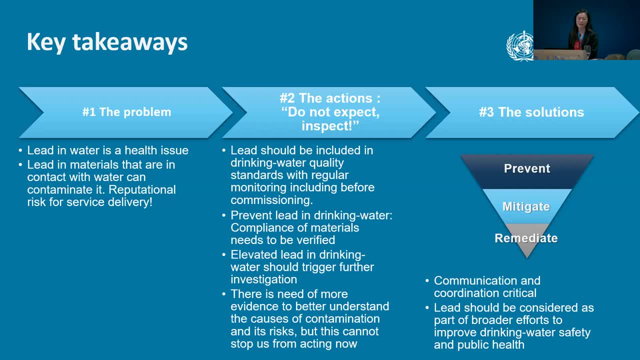 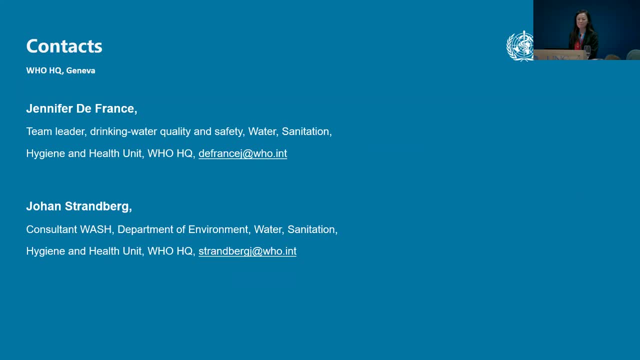 And that will better inform the management action. So taking this stepwise approach is really critical. Just to add, I just wanted to mention my colleague actually, So I'm presenting here to you, but it's actually my colleague Johann Strandberg who who led the presentation of this brief. 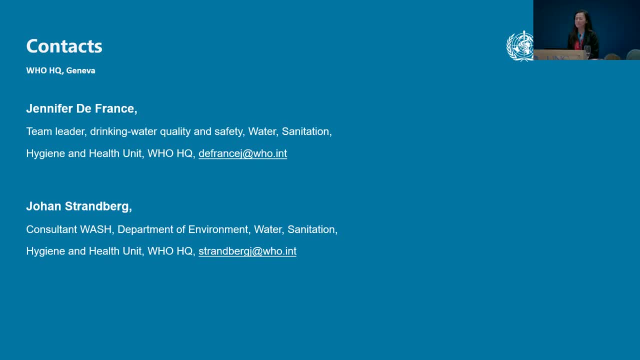 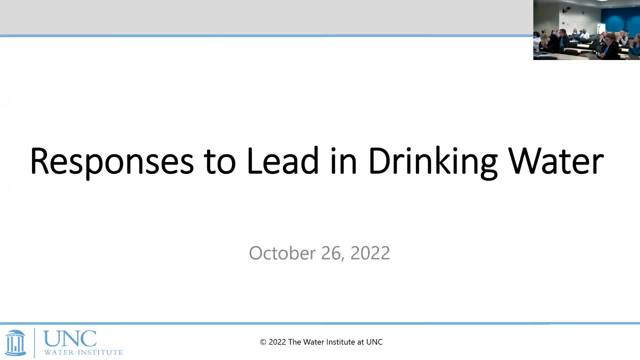 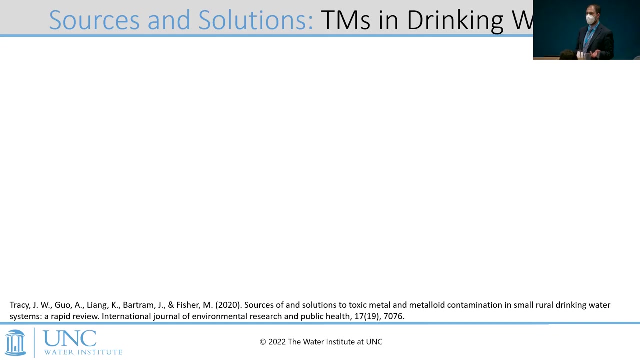 So he couldn't be here- but really thanking him for for working on this. So, with that, thank you for your attention. Thank you, All right, i'll go quickly because I know we're short on time, But I just wanted to sort of draw a few links between some of the examples we're gonna have and some recent work that unc students did as a rapid review on sources and solutions. 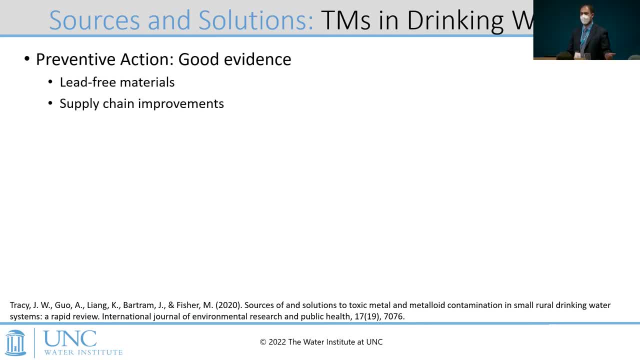 Of lead and toxic metals and drinking water, And so, as as Jennifer said, there's great evidence around effectiveness of primary prevention right. So I mean blessing and a curse if a lot of lead occurrence is due to the use of lead containing materials in water systems. 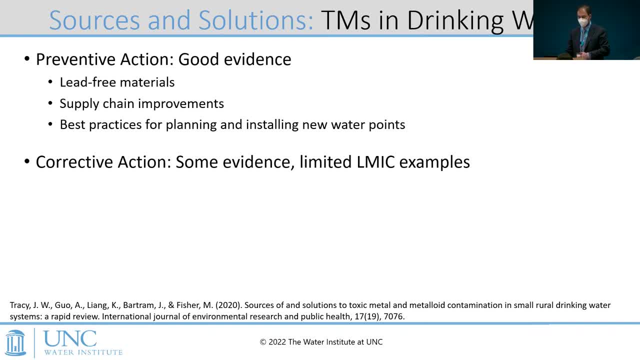 Well, that is something that's highly preventable and so there's great evidence around primary prevention, around corrective actions. You know sort of in that continuum that the who brief explains there's good evidence from high income, country and urban settings. But there are opportunities to generate good evidence around adaptation to small systems, rural systems, systems and different contexts. 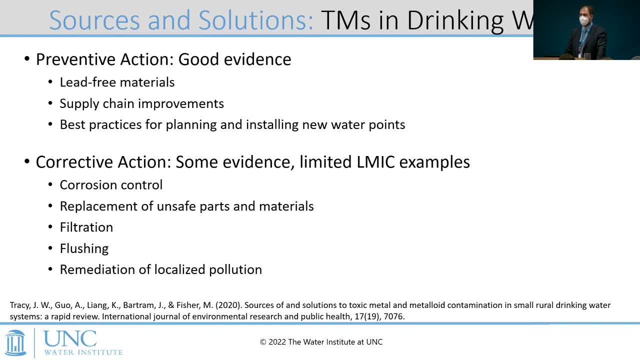 And so that sort of gives us some window into where evidence can help support Next steps potentially, and also links to some of the evidence around implementation Opportunities to find out not just why to act on lead and what to do, but also how to implement it. 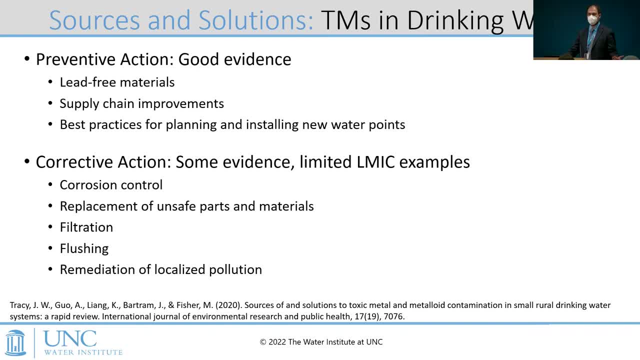 What challenges and what stakeholders need to be engaged, etc. And so I think this is really a fertile area of opportunity for generating evidence, to support action by different stakeholders To successfully Implement some of the priorities that who is outlined and others will be discussing. 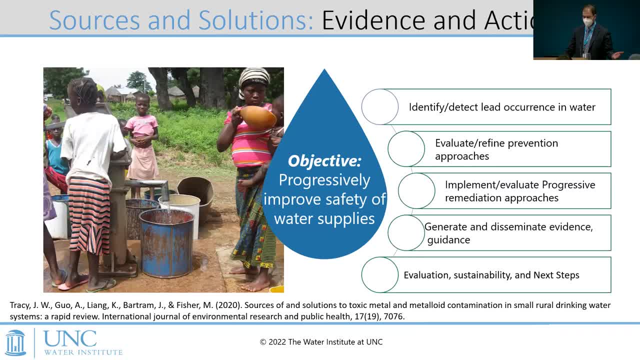 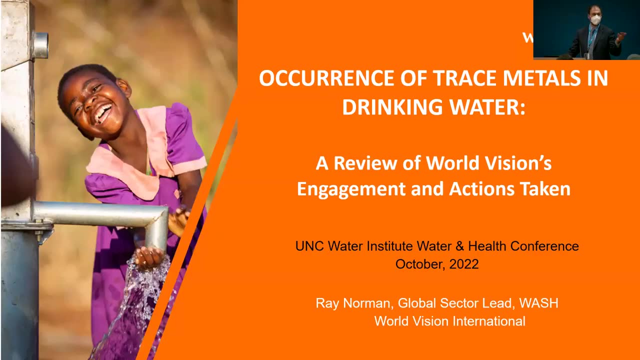 And so i'll move quickly through this. but you know, we we sort of took a took an attempt at framing some of the different categories of opportunities to generate evidence, to improve implementation outcomes, And i'll turn it over to our colleagues from World Vision. 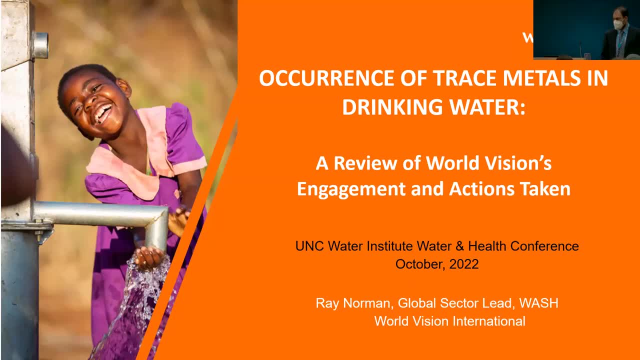 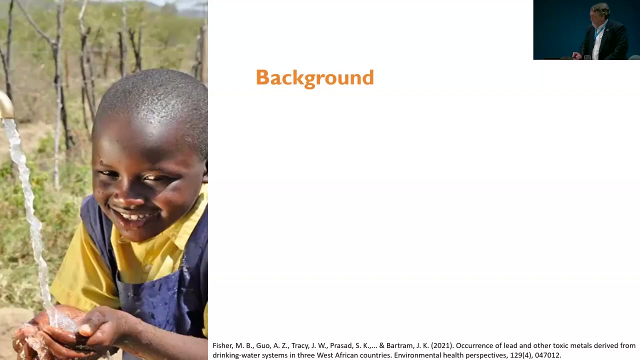 Next. Okay, Thank you, Mike. My name is Ray Norman. I serve as the global sector lead for World Vision's wash program. I want to talk a little bit about what we have done as a major water implementer in some 40 to 50 countries around the world. by way of background, 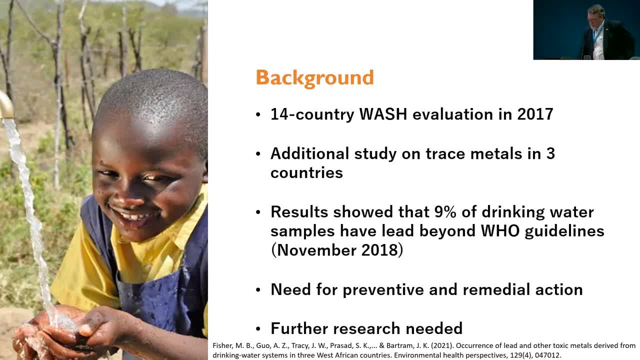 We make sure i've got everything. Yeah, by way of background, The first step we initiated was some years ago. we funded a 14 country wash evaluation that was conducted by Unc. The results of that evaluation have been presented here at a number of conferences. 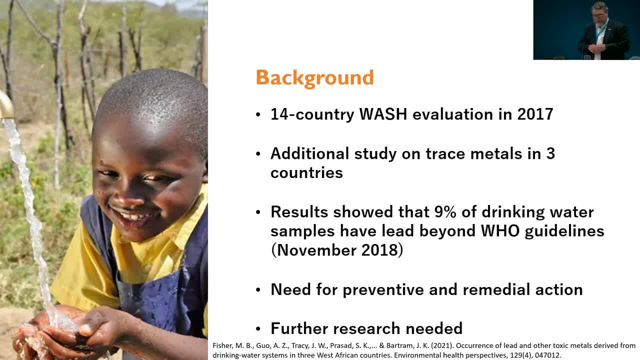 But as we were doing that, we- as as Mike mentioned- We also added a additional study on trace metals in in three years And those results, of course, have been published. You had the reference there a little bit earlier. Those results showed that 9% of drinking water samples in those 3 countries have led beyond Who guidelines. 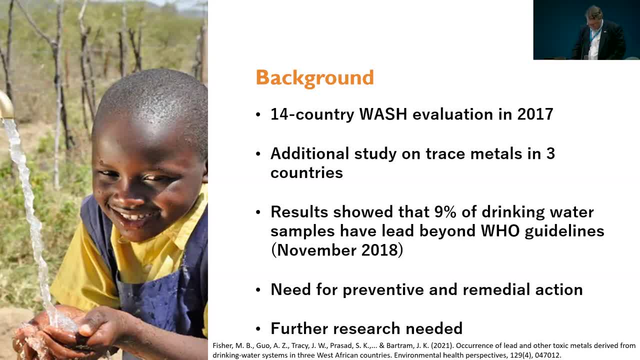 That was published. Well, we we got those results- around 2,018, and as a major implementer of water systems, you know we realize that we need to take action. We need to take preventive and and remedial action. as a water implement. 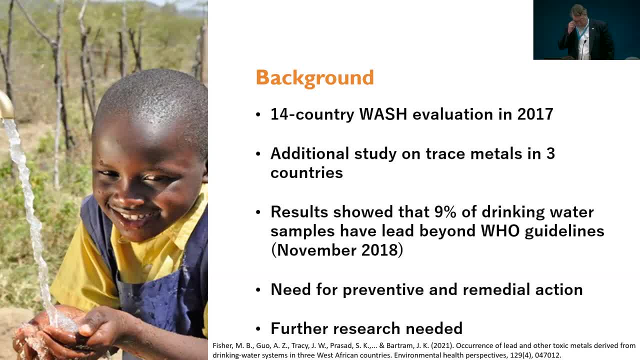 We began immediately asking the question: What can, What can we do, What is our role? And, of course, the first issue was that, as with the way research progresses, you realize that you need more research and before we could really nail down precise preventive and remedial actions. 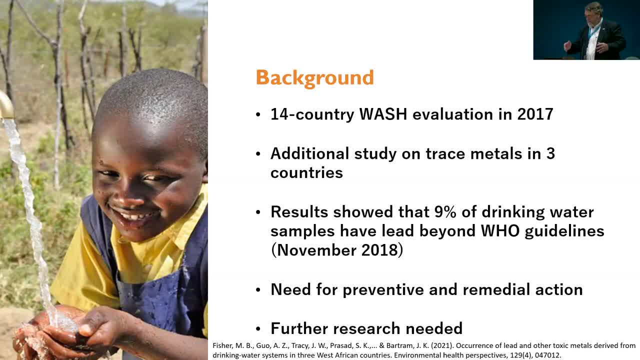 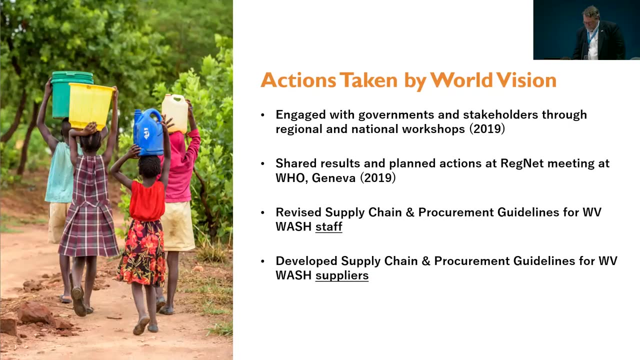 I really appreciated Jennifer's comment here. She said: First thing you do is: don't panic. Adopt a systematic, a systematic approach to in planning your action. So the first thing we did was we decided to engage national governments as a major implementer. 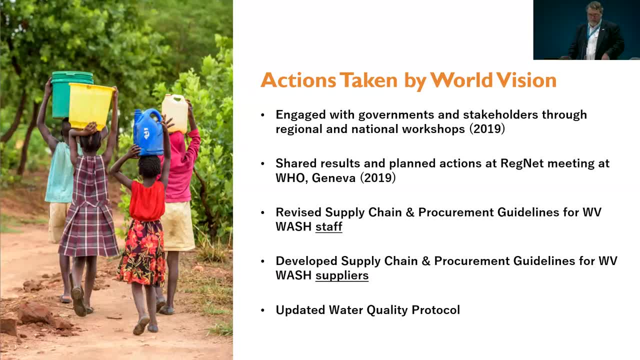 We work very closely with our national government counterparts, usually in the Ministry of Water and the Ministry of Health, because we believe that governments need to own The responsibility of taking action for lid. as a, as an implementer, As a guest of the country, we will follow suit. 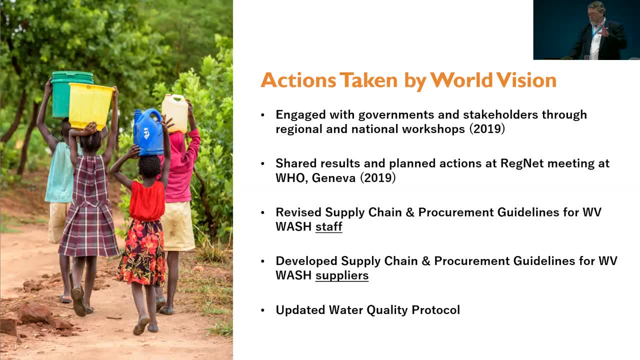 We will take their leadership. So we saw, the first thing that we could do while we're still waiting for more data is to engage with governments and stakeholders at various at various levels. The first thing we did is we organized a, a, a regional workshop in Africa. 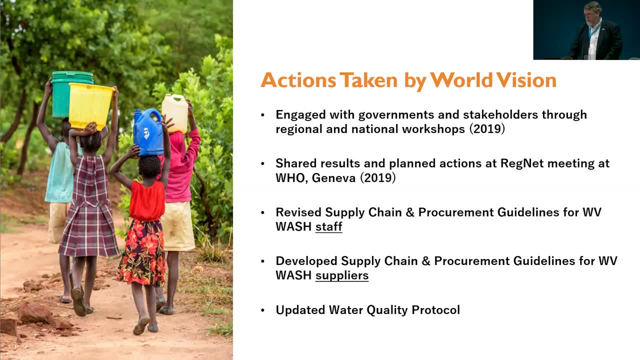 We invited. We had representatives from from. We had representatives from from 4 different countries from the Ministry of Water. We brought them together. We let them develop action plans. They took them back to the their countries. We had at least 2 countries that then hosted stakeholder workshops to present the data and to develop action plans for their around the issue of lead in their national programs. 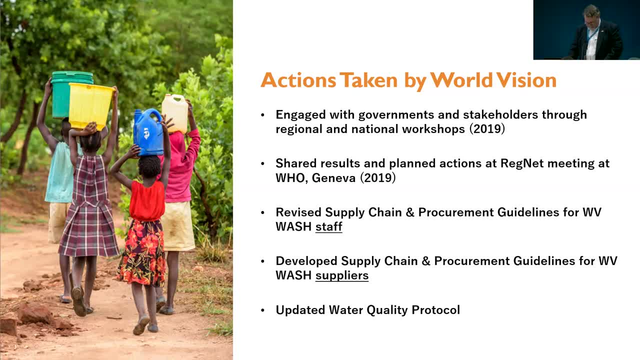 We also were invited by Jennifer and her colleagues at W H O To participate in the regnet- the right water regulator- a network meeting in 2,019.. You and C Shared the results. We were there as well to talk about these issues. 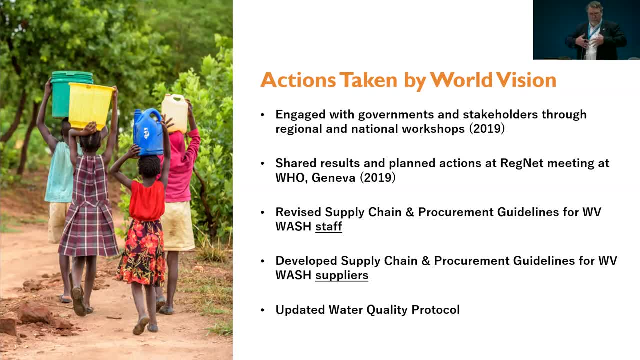 So our we were trying to be completely transparent, to inform as broad an audience as we as we could. Then, turning to our internally, to our organization, To World Vision, One of the first and most important steps we took is we immediately revised and updated our supply chain and procurement guidelines. 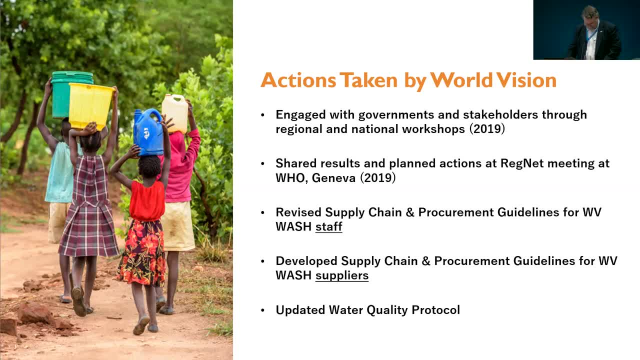 We worked with a number of different organizations to to develop that. Of course, the goal is to assure lead free, certified materials and parts in our systems, and that took several months. We at the same time, We also developed a supply chain and procurement guidelines. 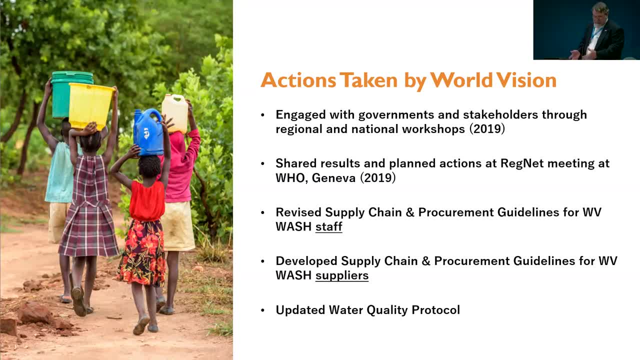 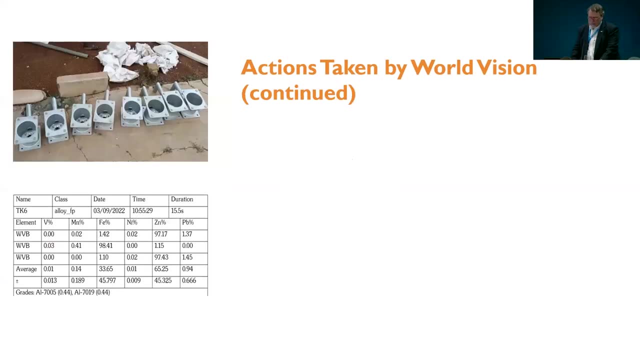 For our suppliers and we sat down with our suppliers and worked through that as well. We also updated our water quality protocol. This was for our field wash teams and with the, with the, the updated supply chain and procurement guidelines, We also began having regional meetings where we took those guidelines. 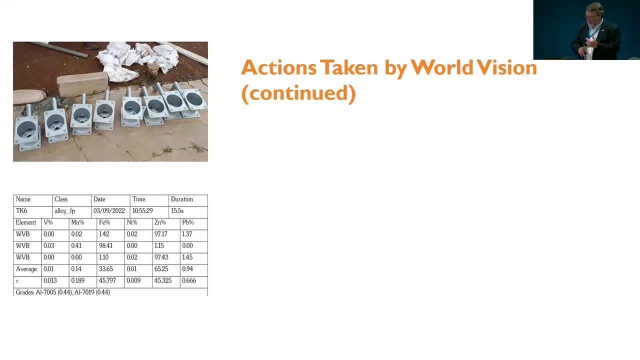 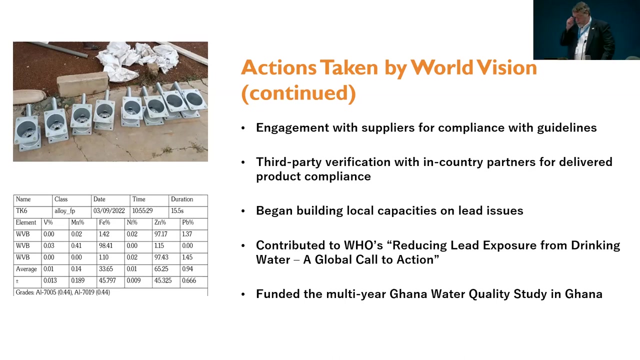 To our field people- not just our wash staff, but to our supply chain and procurement staff and to our auditing staff- and worked through those revised guidelines at regional meetings across across Africa. We also directly engage suppliers- and we are- We continue to do that- around compliance and guidelines. 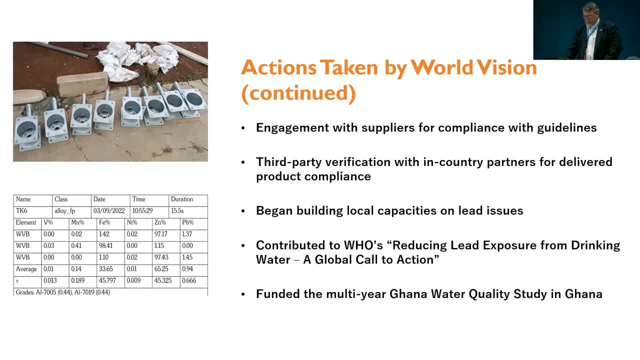 We We purchase a lot of wash related material and so we're very engaged with with suppliers. So that is an ongoing, very active conversation that we continue to have and we'll continue to have. We also took up third party verification within country partners for the products that had been delivered to be to assure that they were in compliance. 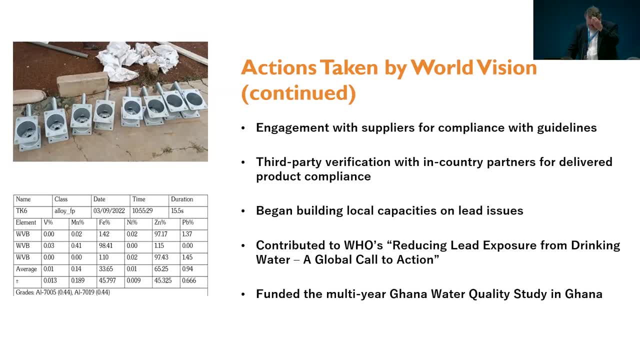 We worked in, for example, in Ghana with the University of Mines and Technology, Using an Xrf spectrometer, and we worked on that with them to scan materials that had been procured. Some very interesting learnings came out of that. You can actually see a table there that, on the far right column, shows some of the lead and different different components of a pump, a pump system. 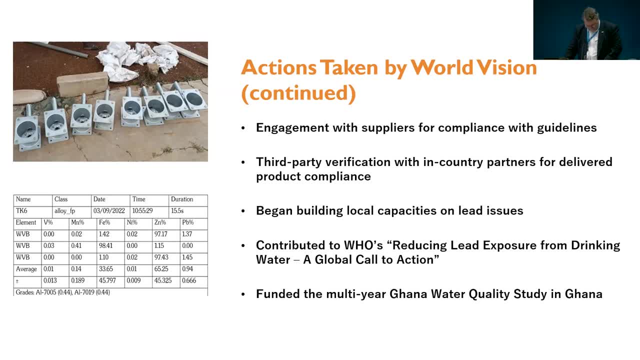 But third party verification we felt was very, very important. We've also begun building local capacity on lead issues. We've engaged with the national water ministries. for example, in Ghana We work with the community water and sanitation agency. We also work down to district assemblies in in building their capacity and understanding the challenges around lead. 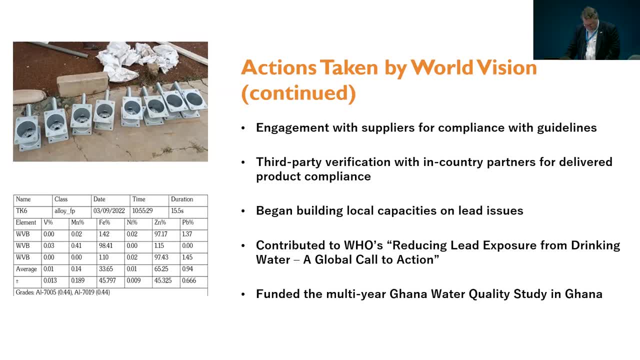 We've also been working with the national standards boards in both Ghana and Niger to improve their standards And since we have worked for many, many years with major pump manufacturers, we are engaged with them. We've also been on the use of standards to improve their product quality. 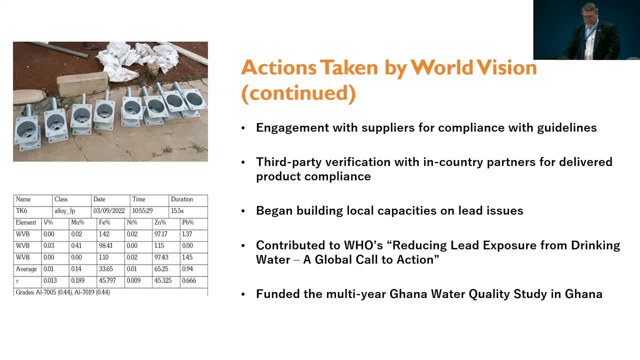 Jennifer mentioned the technical brief. We had the privilege of being involved with W H O in preparing, contributing to the preparation of that brief. and perhaps most importantly, most relevant as we speak is we have just world vision has just funded a new study to take the lead research to another level in Ghana. 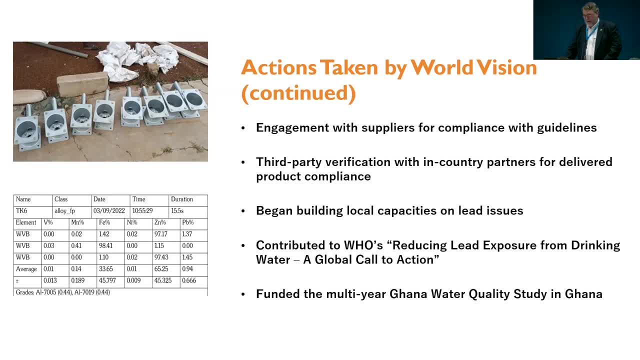 We've launched- We're funded- a multi, a multi-year study in Ghana. It's a collaboration between the water Institute at Unc, World vision and the community water and sanitation agency in Ghana to really try to get to the next level of evidence, especially trying to really understand where the source of lead is coming from and develop, of course, preventative and remedial. 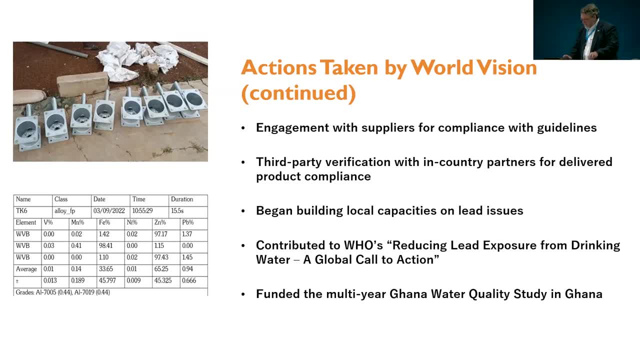 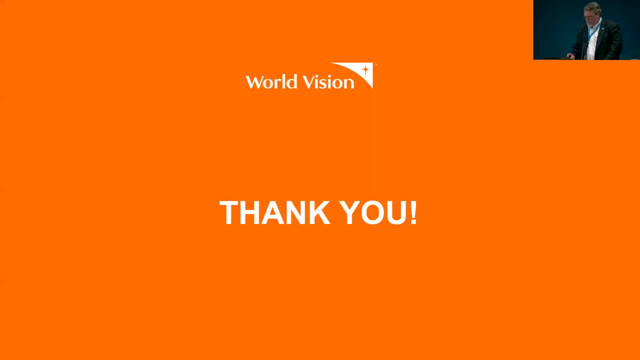 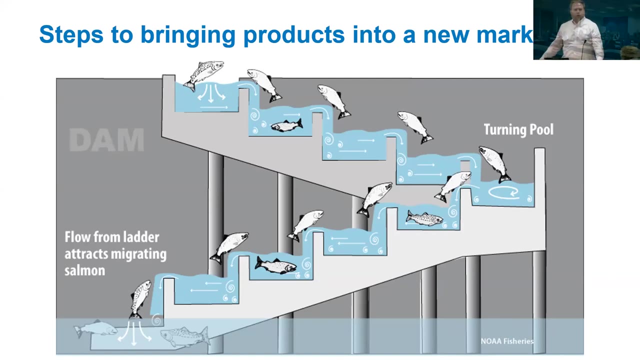 measures from that. I will stop there, But those are a few items of what an Ngo, A water implementer, can do as we tackle this, this lead issue. So my name is Christopher Lindsay. I am a vice president of government relations for Iamo. 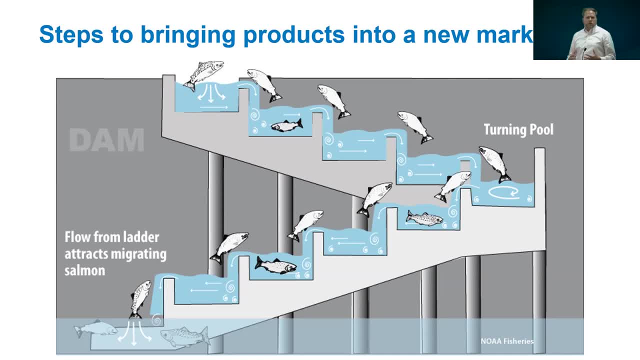 And, as Dane was saying earlier, we're an international trade association That's an important voice for the plumbing and broader water And sanitation sector. So our key stakeholders include manufacturers, regulators and those on the front lines of installing these types of systems. 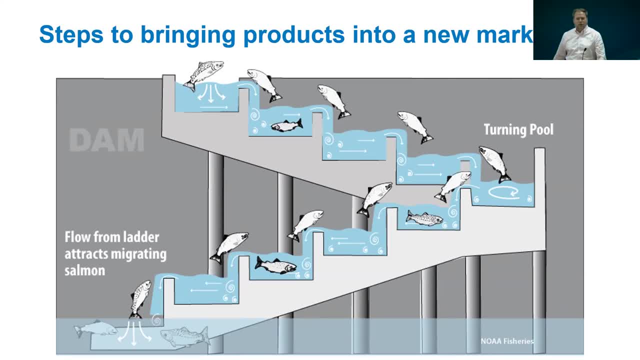 Now I brought 2 slides with me, and one is more kind of a water analogy, because I love water analogies. I grew up in the, the Western United States, and so dams and rivers are something fairly common that we have to, or fairly common in our environment. 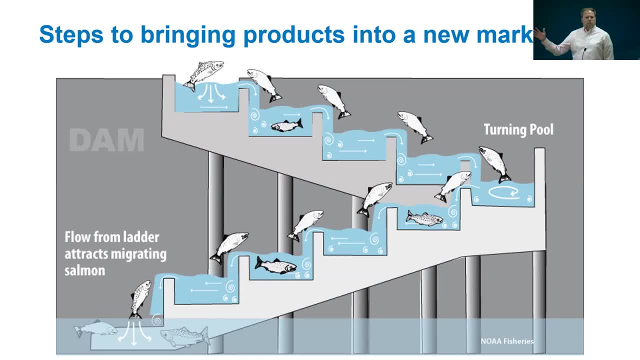 And one thing we've learned is that you know, when you put up a dam, You create a pathway for migratory fish to be able to get back upstream to, you know, to the headwaters, And essentially you know this where it relates to kind of the work we're talking about now. is you know one of the things that W? 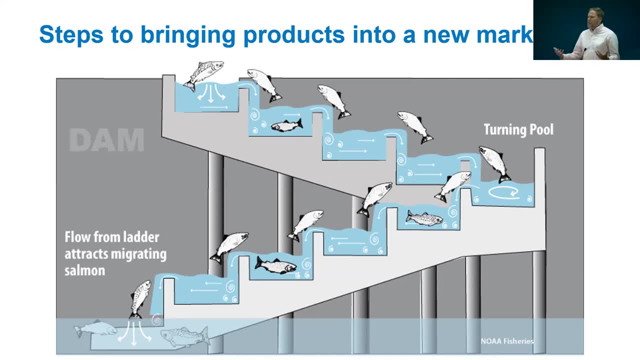 H O has pointed out is one of the key steps we can take is just to prevent the flow of lead materials, you know, into these, into local markets, If so much of our- you know- wash projects are based on locally sourced materials. 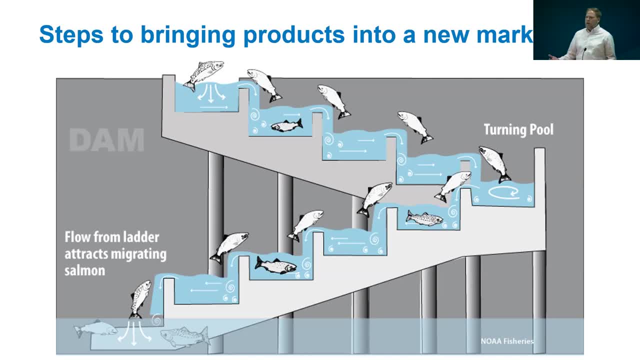 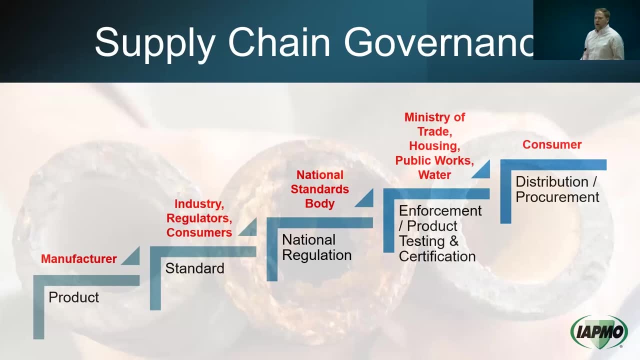 How do we prevent the materials that are available From containing lead in them? How do we influence that process? And so I wanted to speak to a couple of those, those points today As we begin. I think it's helpful to understand really supply chain governance, and i've kind of outlined some basic steps here to and understand. 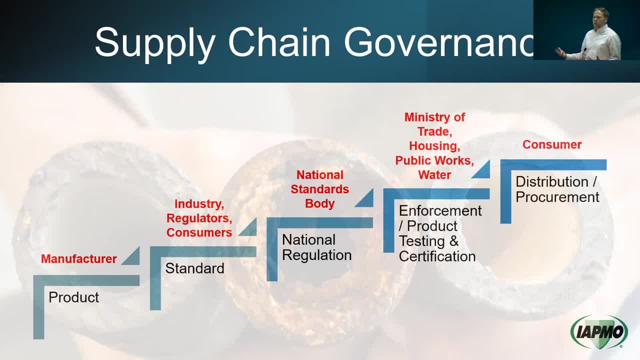 So help illustrate where we're trying to influence the process. As you can see in the very, the first step is a manufacturer comes up with a product. Usually at that point, if it's a established industry, If we're not assuming, like a new technology, you know 5g or something like that, or you know we're guessing in beyond 5g. 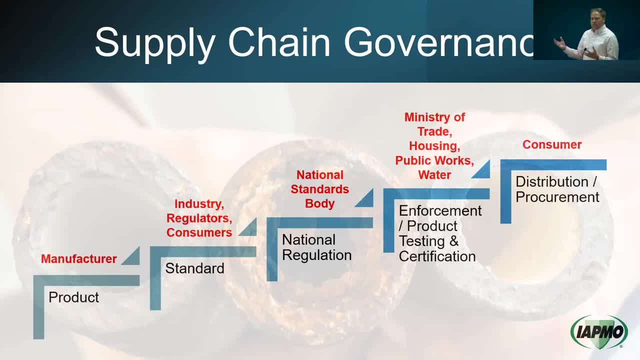 But you know, if we're not dealing with the latest thing on the market, you're coming into an established industry, And so industry partners then gather together from you know, manufacturers, regulators, experts, and they decide to give a basic standard for how that particular product is going to fit into the broader ecosystem. 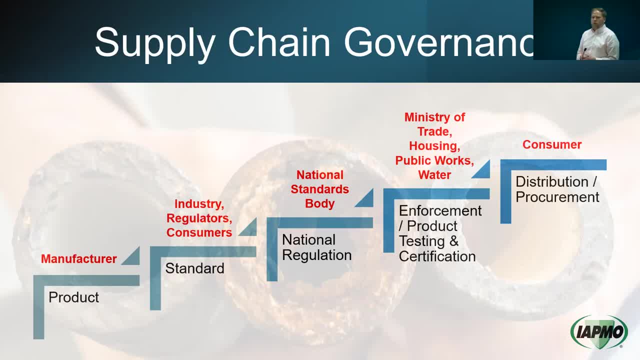 And what are the safety and what are the efficiency requirements that should be required for that product, That all, the class, All, And the products in that class of goods you know we'll, we'll kind of be characterized by Then? you know, these standards are adopted either by national law or in technical regulations, you know, by a national government. 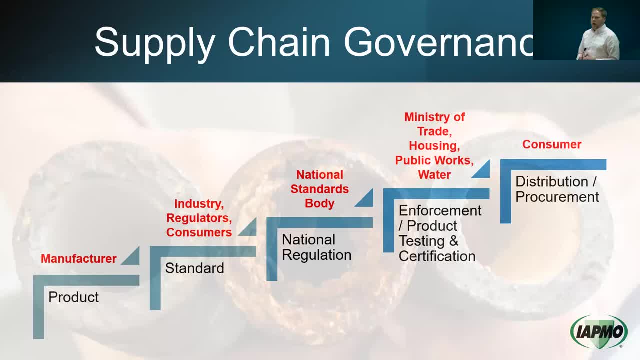 And that's really where it begins- becomes the force of law you know behind it And the key step usually in that process is the national standards body As we go into the next step of how do we implement or mandate that, that particular standard or that new national regulation. 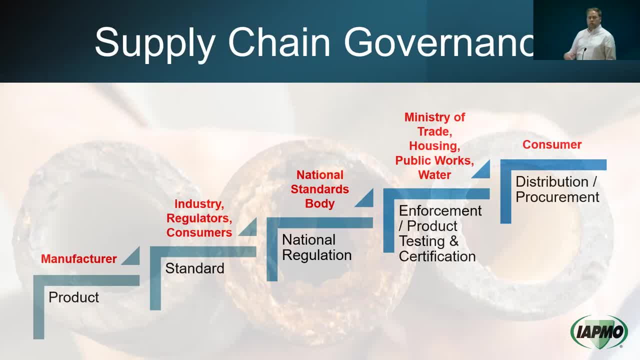 It falls into the hands of different ministries. You know, ministry of trade is what regulates what products can come into the borders. Ministry of housing or public works or water, The ones who actually mandate that these products have to be used within our systems. And then, beyond that, the next step, it comes down to individual consumers. 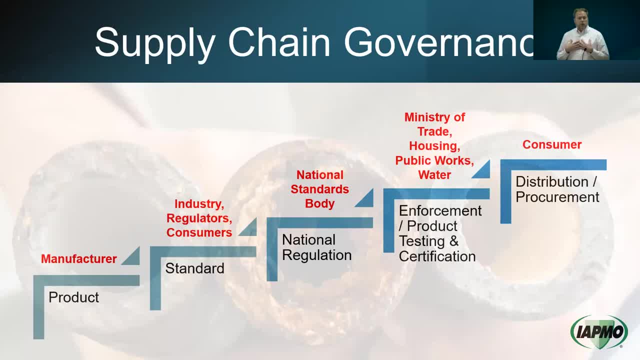 Now the average consumer cannot tell the difference between which pipe has led and which pipe does not, And so by influencing what products are coming into it, Make some to some extent make that decision easier for them, and certainly large purchasers. I guess world vision was just you know, Ray was just saying you know they can dictate what products are used in their supply chains, and so they can influence the process through through their own programs. 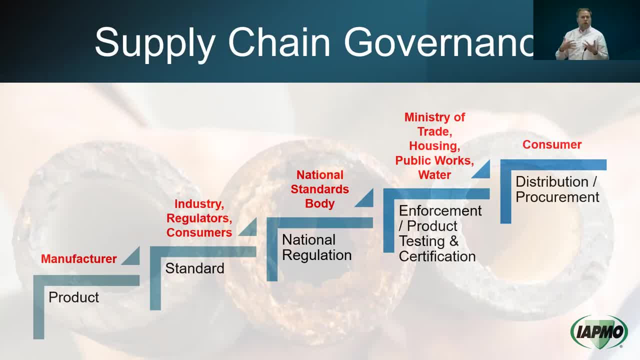 And certainly, as you know, for many of you who are implementing partners, that's something, that step that you can take as well. A couple of key points as you look at this: these, these steps here. for the supply chain, Governance is, first off, that step where you take the standard to the national regulation. 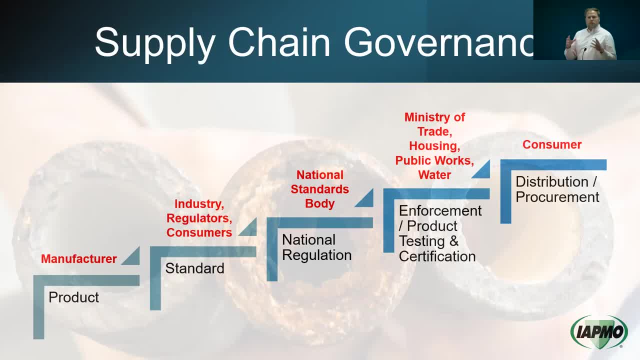 This is often where you know, we take an international standard and we tailor it towards the local use. by what? but still keeping the foundation of of the of the standard. So, for example, we worked on a regulation this past summer in Indonesia. They were looking to update the standards for faucets. 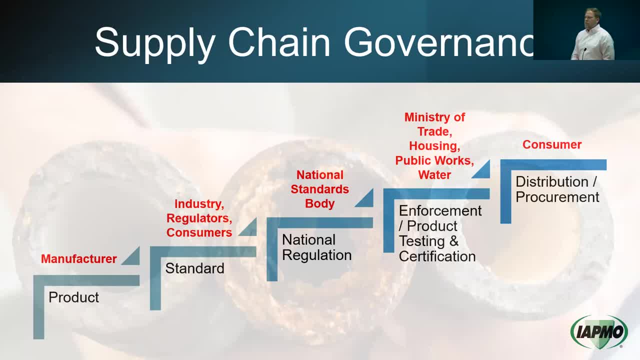 It's all taps in their country and one of the things we heard from local manufacturers was that, hey, we cannot meet the performance requirements Of international standards. you know we can. you know we can't do the. we can't beat the life cycle. you know parameters that have been set. 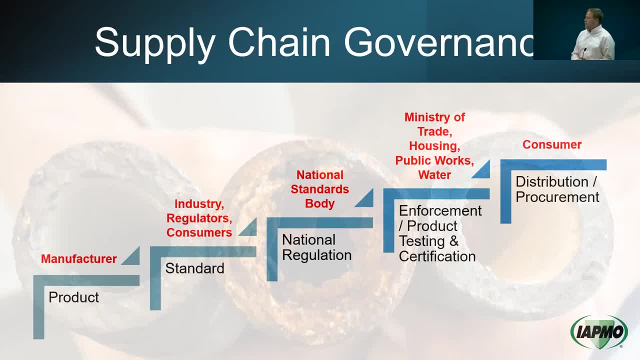 However, we can meet the safety, achieve the parameters, And so we worked with them to say, Well, okay, we can adjust the some of the performance requirements. Well, they may not be quite as high performing, but at least they already. they will address the lead issue. 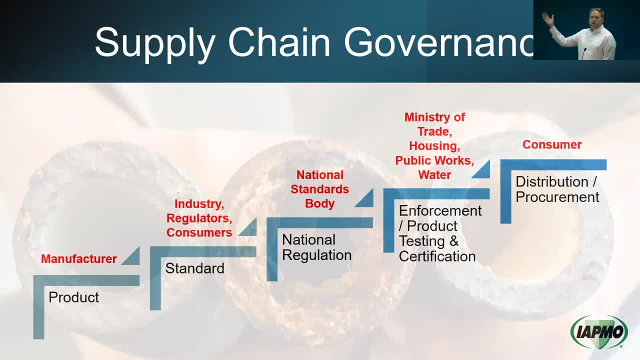 So that products coming into the market, if they exceed it great, you know, performance wise, But at a bare minimum The products being sold, you know, as that gets mandated and implemented, will no longer have lead in it. And so that's where that kind of that negotiation, that tailoring, takes place between local industry and international industry. 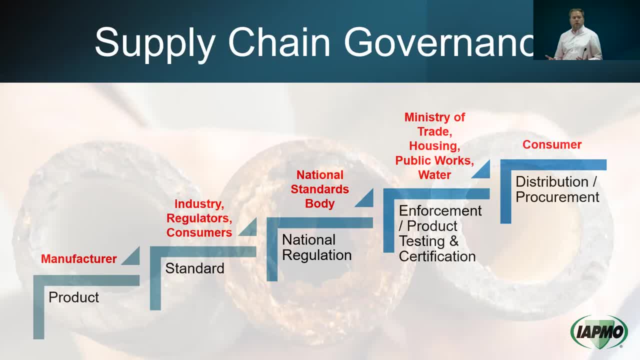 The other piece that we've heard about today is that testing and certification off times for products that require, you know, deal with public health and safety. One of the best practices you know worldwide is to require independent or third party testing and certification. 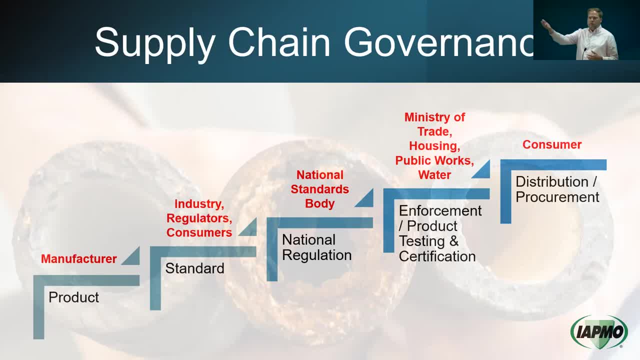 So you don't have to take a individual manufacturer from another- The other side of the world's- word on it that their product doesn't contain lead. You know it's independently verified to do so, And so that's one of the things that you certainly can impact. you know, as you're looking at your own supply chain and procurement processes is requiring that you know products being supplied, you know do have that independent verification. 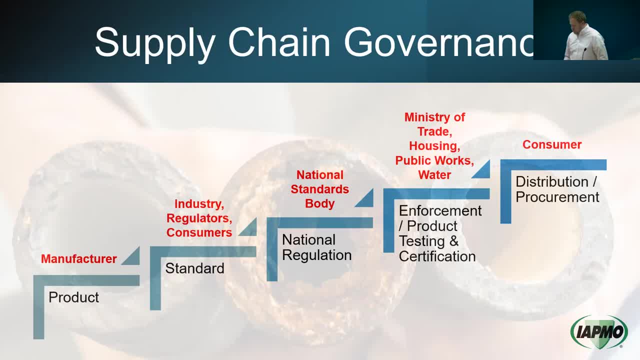 The other thing, kind of maybe looking more now at a couple of examples from the United States of where this has been actually implemented in real life In September 2018.. EPA finished finalized their lead free rule, where they actually said as part of our national regulation that all products being sold in the United States can contain no more than 0.25% of the weighted average wetted surface of that product can contain. lead. 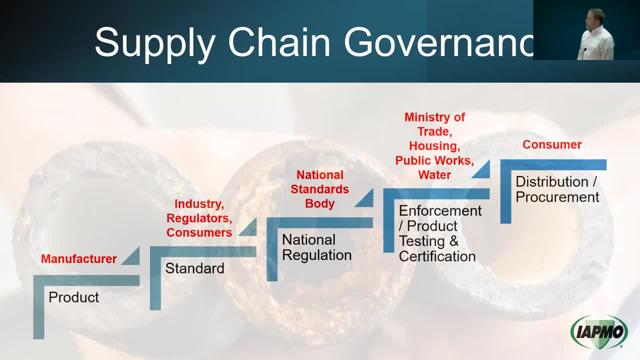 Later, two years later, actually just this past winter, California took it a step further and said: we're not going to look at the prescriptive requirements anymore, We want to look at the performance of the product And so, from now on, all products being sold in California starting- and I think- 2024.. 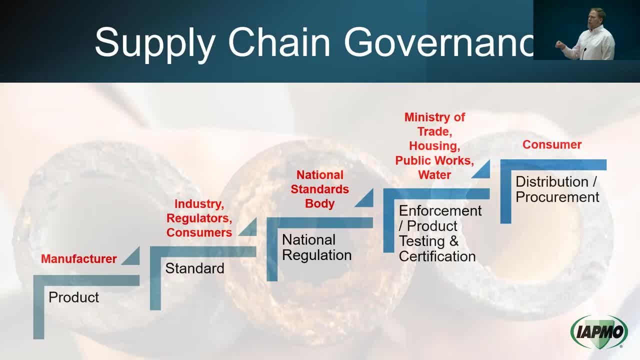 They can no longer leach lead more than one microgram per liter. And so- and that's these kind of steps like these by national economies have ripple effects across the entire industry, because multinational manufacturers aren't going to create one lead product and one not. 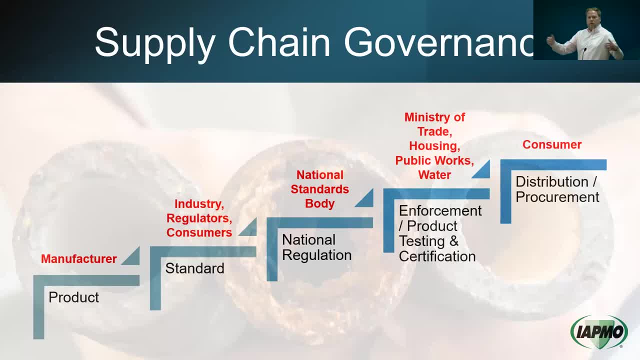 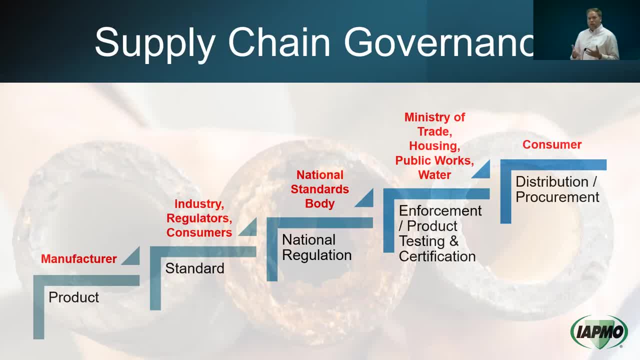 However, there are still steps to be taken, particularly with more dealing with products that aren't necessarily sold in high, high income countries, or that you're dealing with manufacturers that are only sell locally or regionally, And for us, this is where, you know, being able to influence this process at every you know with each national government is become an important you know- priority for our industry. 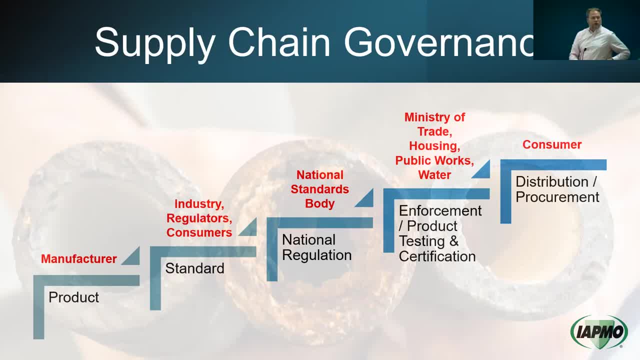 For example, when hand pumps have been a big part of our discussion, the after dev and the Indian mark to pump. There really is beyond hand pump specifications. There really is beyond hand pump specifications. There really is beyond hand pump specifications. So you know, when hand pumps have been a big part of our discussion, the after dev and the Indian mark to pump specifications have been developed by Scott Foundation. there really is no standard, you know, for those. 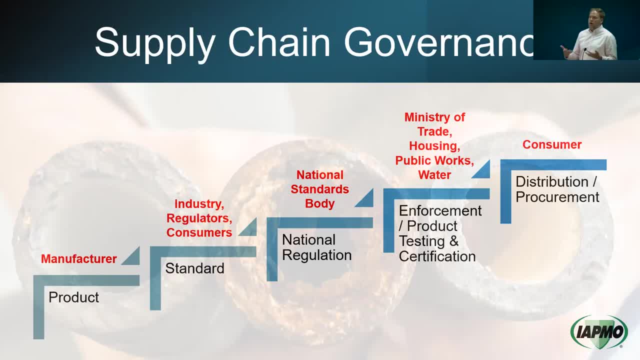 So there is no requirement that those products don't contain lead or the brass parts in those not have lead in it. So industry is working actually to develop an international standard with us and the key partners there. that then can become, you know, a part of national regulations and have the force of law so that you know products can be stopped at the borders or manufacturers. 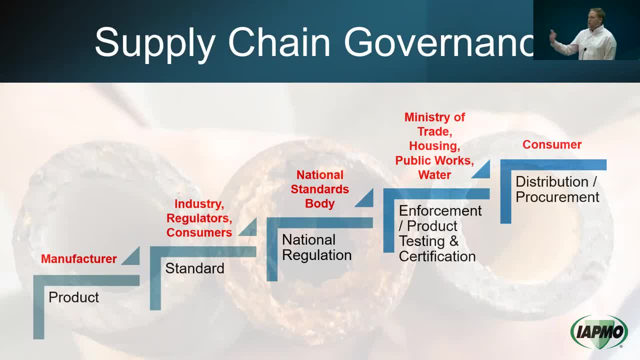 your retailers can actually require certain things. you know when they go as part of their product. they go if it's part of their procurement processes. um, you know, as we look more broadly, what needs to be done in this education. certainly you all coming here today and becoming better. 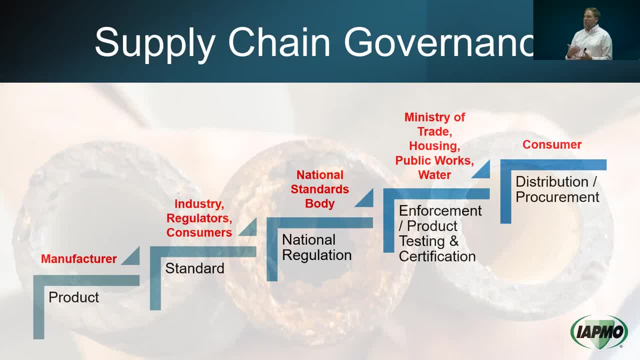 informed about this and as, hopefully, taking that knowledge and being able to apply it in your work uh is an important part of what we're hoping to do. data: we've heard we we'd love more data. you can see that there are some keystone uh. uh research that has been conducted to show the 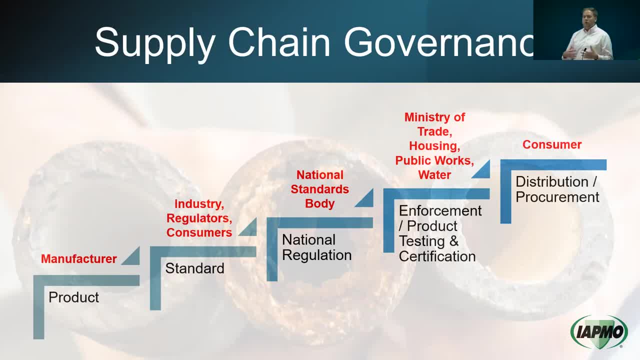 prevalence of lead and pfas and other contaminants. we welcome more, and so, as you think about potential or future research opportunities, uh, we'd love to take advantage of that for our, our, uh, in our work as well. um, and then you know, we'd love to partner with you. yeah, that's what kind of? 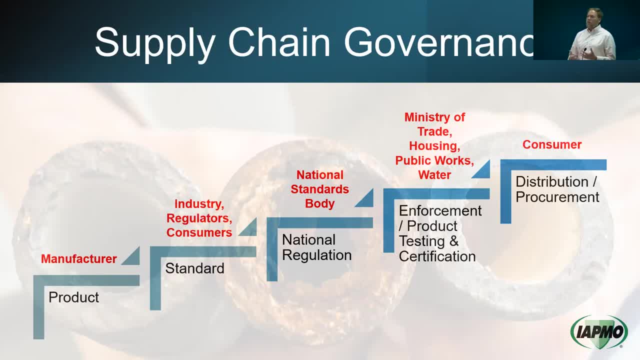 my final thought. i mean as, particularly as you work with water governance, we see addressing issues like this as an industry as an easy add-on to some of the broader, you know- governance themes that need to be addressed that we're working on as a sector, um, and so we'd love to work with you. 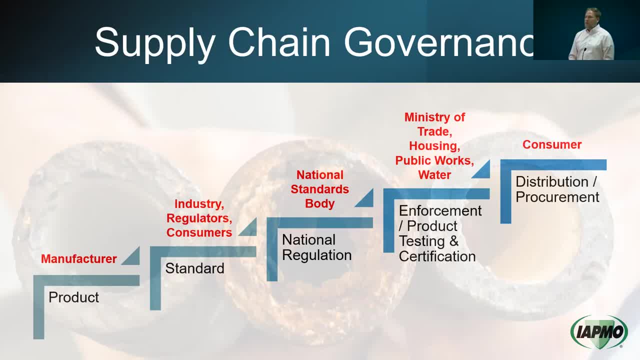 as you're making some of those investments just to include a couple of the you know these processes that are important to industry and we'd love to partner with you as you're making some of those investments just to include a couple of the you know these processes that are important to industry. 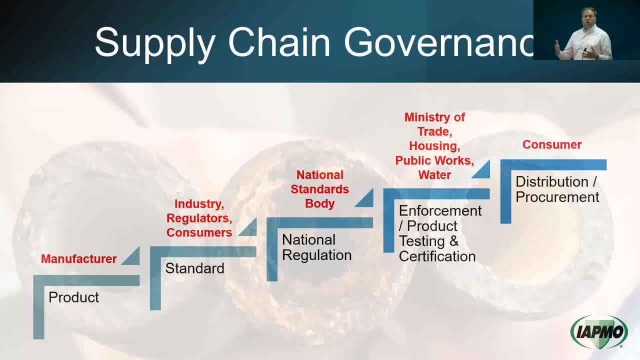 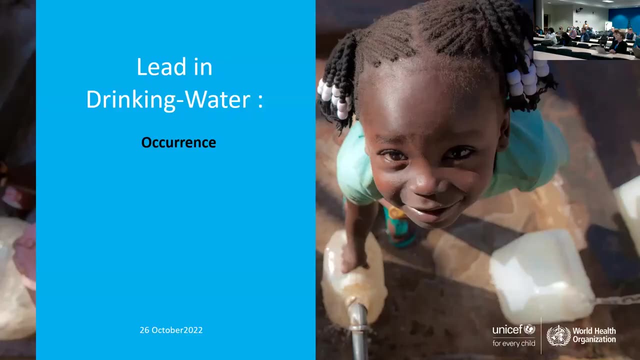 that will help to increase the flow of safe products while preventing- uh, you know, lead, lead contaminated products from entering the market. so thank you for your time. so we will turn it over to jorge to talk. yes, okay, we are almost there. um, allow me, in the next slide, to 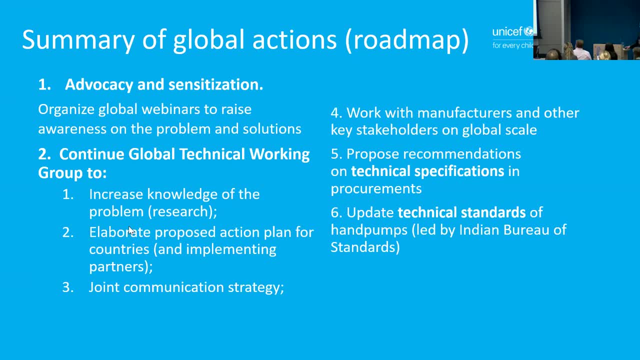 quickly introduce a summary of some actions taken by the informal toxic metals group. that includes several organizations such as unc, who, world vision, iapmo, water aid, the rural water supply network, leeds university and the organization i represent today, unicef. our group is open to more members and our 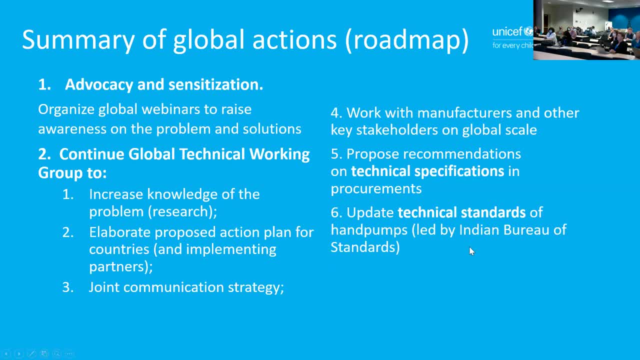 focus is now on advocacy and sensitization and also continuing- uh i will represent the university- our ongoing work on increasing knowledge of the problem, so doing some research, elaborating some proposed action plans for countries and implementing partners and doing a joint communication strategy. given the sensitiveness of the issue, we also work with 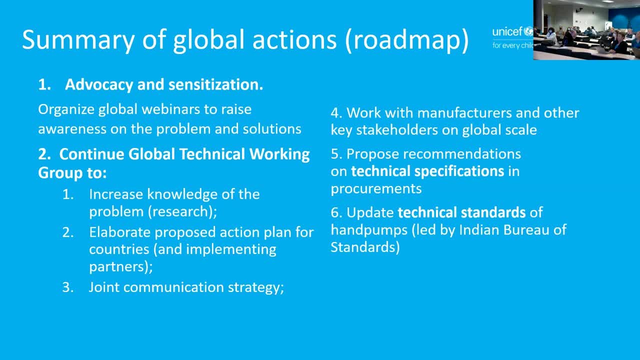 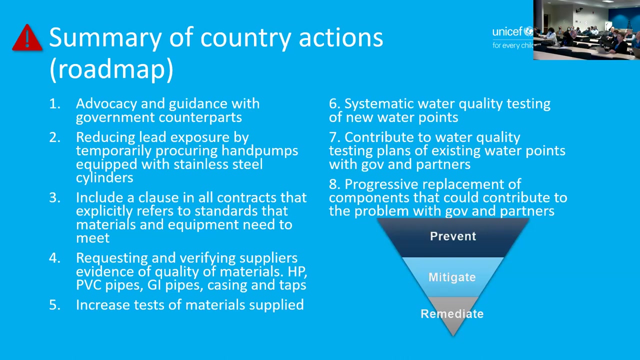 manufacturers and others- key stakeholders on a global scale- and propose recommendations on technical specifications in procurements, and we're working with them, with organizations like the indian bureau of standards, to update technical standards. and next slide includes a summary of country actions, proposed actions that governments and other stakeholders can do in your home countries. 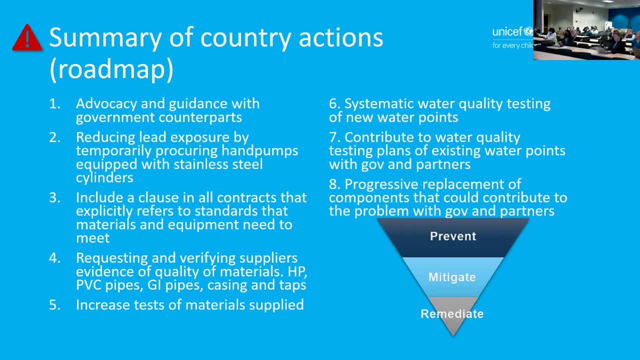 so one of the proposed actions is to help us to spread the voice and to contribute to advocate for for this topic and, to you know, to to have discussions in your own countries. Reducing lead exposure can be done in the case of hand pumps in rural areas. 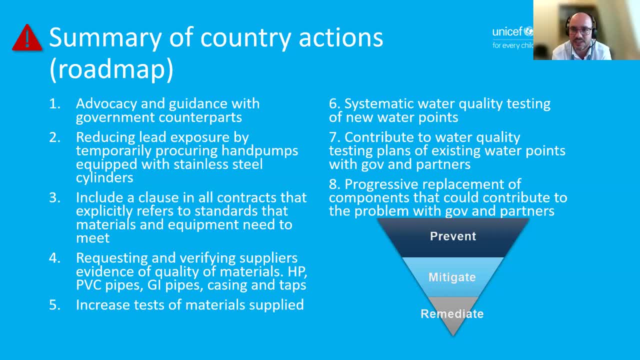 by procuring, for instance, stainless steel cylinders. It's a no regret, immediate option that can be done in many countries. For service providers, for organizations supporting the provision of services, we are recommending to include a clause in all contracts that explicitly refers to standards. 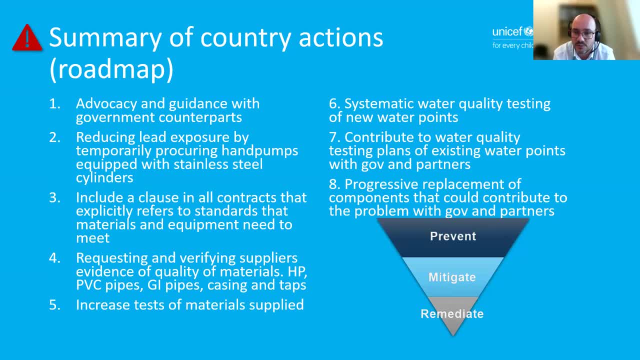 that materials and equipment need to meet And, as Ray mentioned, one of the recommendations and one of the actions that organizations like World Vision is taking is requesting and verifying suppliers evidence for quality of materials, in particular, on hand pumps, PVC pipes, galvanized iron pipes, casing stubs. 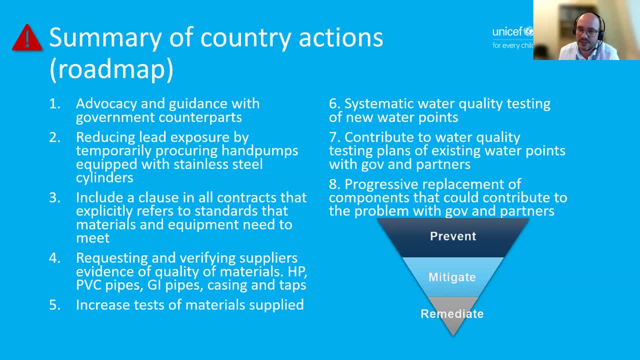 It is also recommended to increase tests of material supplied, as well as to systematically contribute to quality testing of new water points. And answering the question from a participant from USAID, we are not at this stage- not at this stage- recommending to include lead in the JMP data testing. 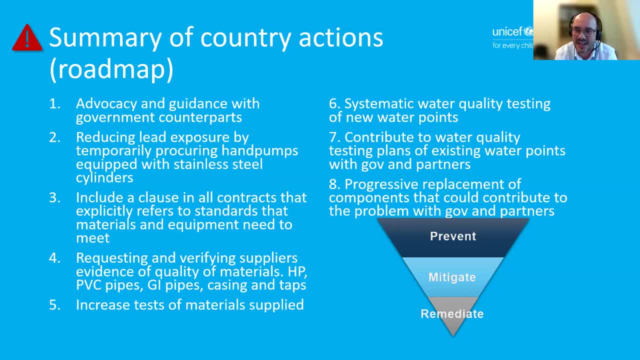 Maybe I misinterpreted. I can explain myself, but definitely we are recommending partners and governments to start considering collecting some information about lead concentration in systems, So contributing to water quality testing plans for existing water points and the progressive replacement of components that could contribute to the problem. 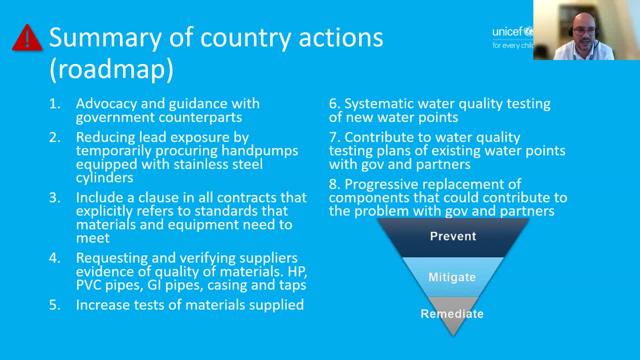 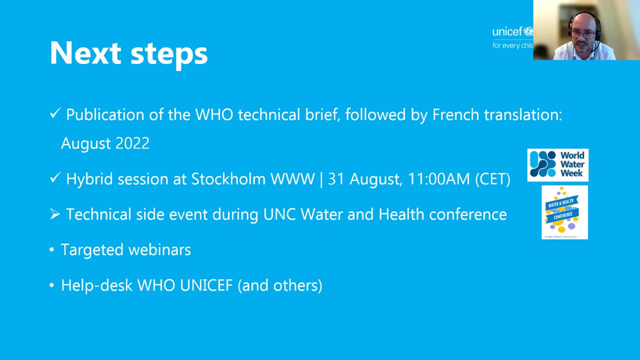 together with government and partners. And my last slide is is on the next steps. So Jennifer from WHO just presented the WHO technical brief that has been recently translated. It was launched a few weeks ago at the Stockholm World Water Week. It's being presented today at UNC Water and Health Conference. 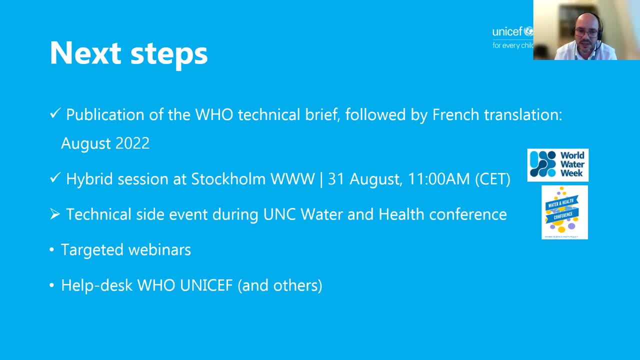 And we are open to support to some targeted webinars and to support countries interested and countries and partners interested in being part of the solution. I thank you all for listening to me And I think we are moving to the last part of the session. 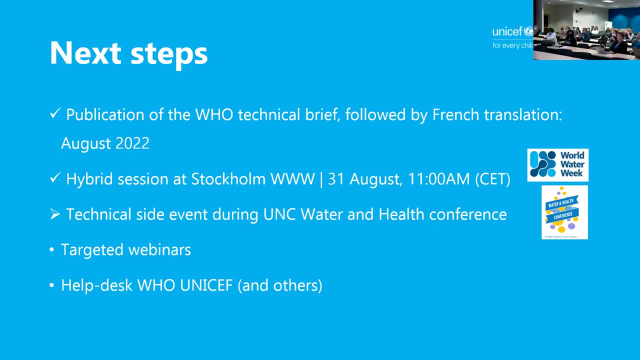 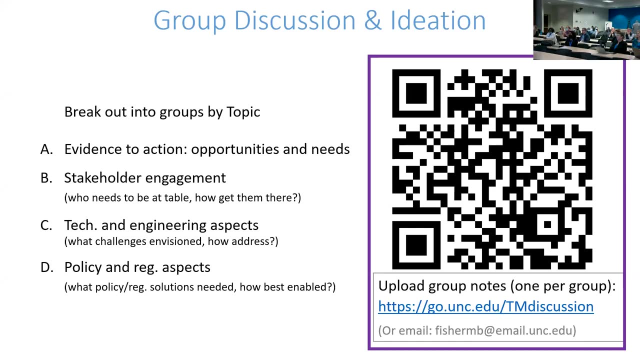 I don't know who is facilitating this. Thank you, Jorge, Appreciate it. So the goal here was to actually break in a small group, break into four groups here and talk about these items. We're running out of time, So we don't have the ability to break in a group. 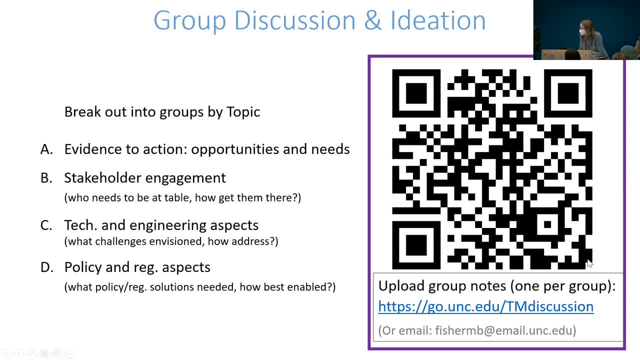 but we do want to hear from you. We want to hear and have this discussion So in your mind, A look at the evidence to action and opportunities that are needed. What stakeholder engagement? Who needs to be at the table for this? 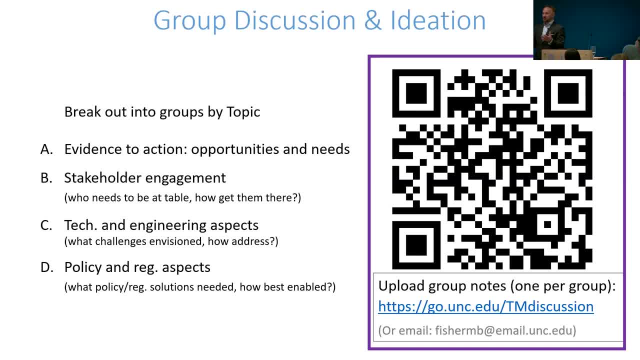 Like. we want to hear from you. This is your opportunity to have some of the best experts in this field on these issues here in the room. Who needs to be involved here? Also, you know what technology, what sort of engineering aspects do we need to look at? 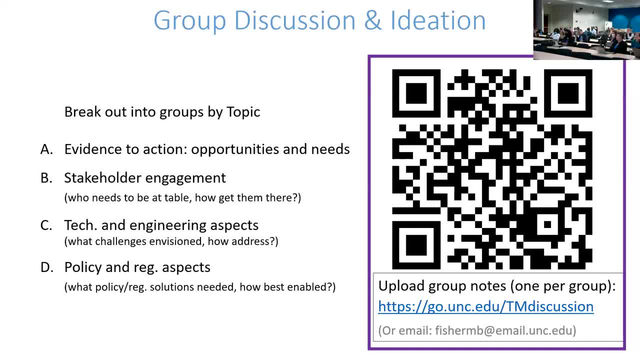 when we engage on these types of activities, to make this. this is a preventable issue. We've talked about this many times. like some of the bacteria and pathogen other areas we've talked about is a difficult hurdle, but this one is completely fixable and preventable. 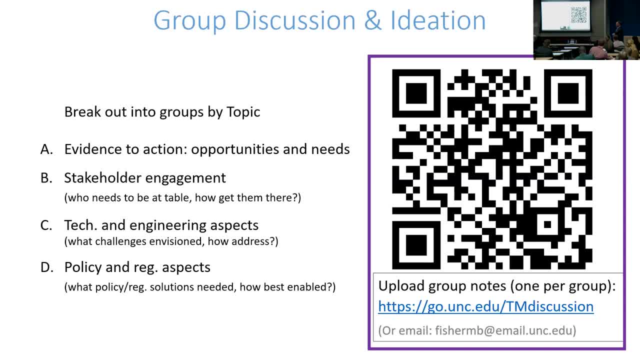 if we address it right. So what else is needed? And also, you touched on the policy. What policy or regulations need to be changed or impacted or implemented into projects to make sure that we stop from doing that? So there's a QR code. 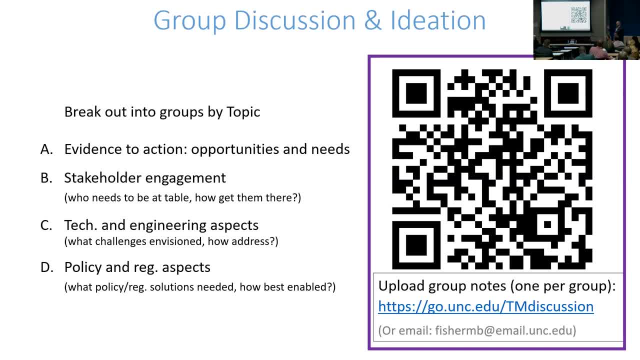 If you want to upload anything of any ideas that you have, that where we can start discussing this today. but we'd love to have a little bit of discussion for the next two or three minutes to hear from you What, what, what. who else needs to be at the table? 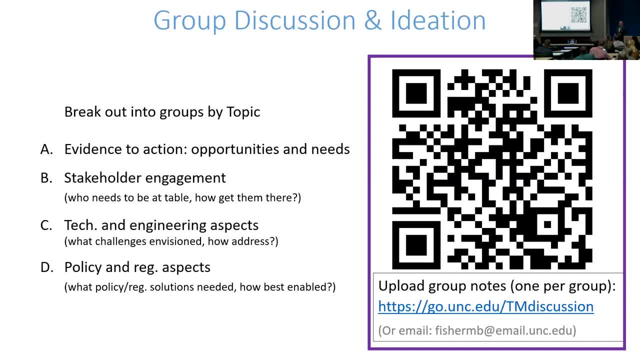 Who wants, what technologies do we need to impact, What policies need to be changed And who else should be at the table here. So do you have anyone to say? we can hear from Who's worked in this area? What who? who feels we need to make some adjustments here? 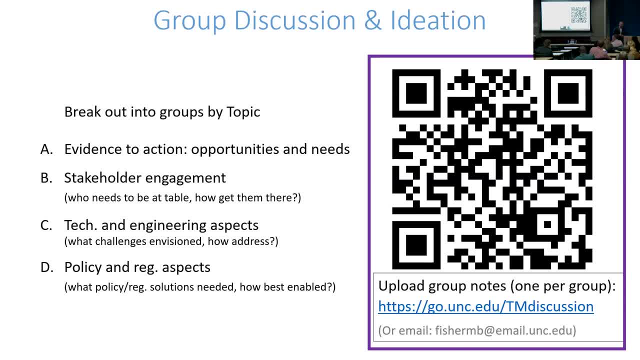 Yeah, and we'll grab the microphone if we can. so we can, so we can get you on the recording. And please do submit responses to this as well. We'll be collating and sharing those back with those who want. Hi, Yep. 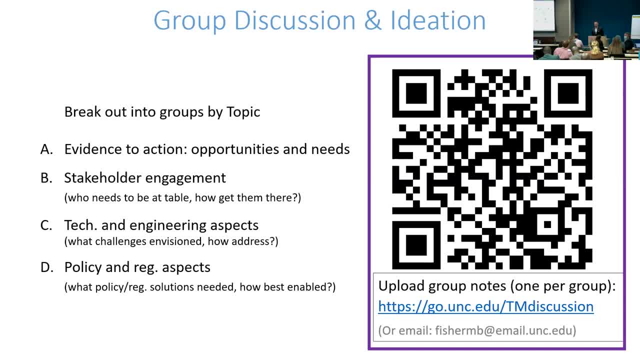 Okay, I was thinking about a little bit about the what can be done section that we just talked about, And a lot that was shared was really good And the whole thing about prevention being key is amazing and it was, but it was very high level for about like. 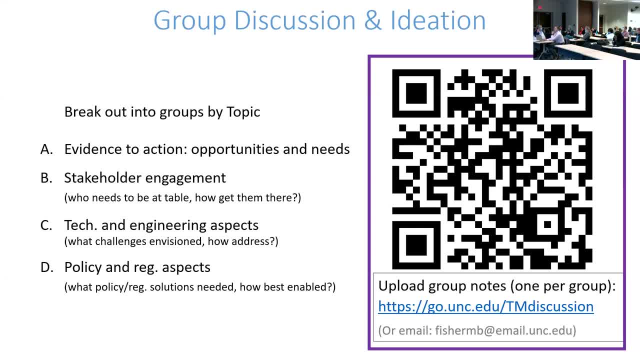 what can be done by countries, bigger groups of people, And I was wondering if there was any thought put to what could be done at a household level. Jen mentioned that cost is a big issue, like there's filtration, but what if you can't get certified filters? 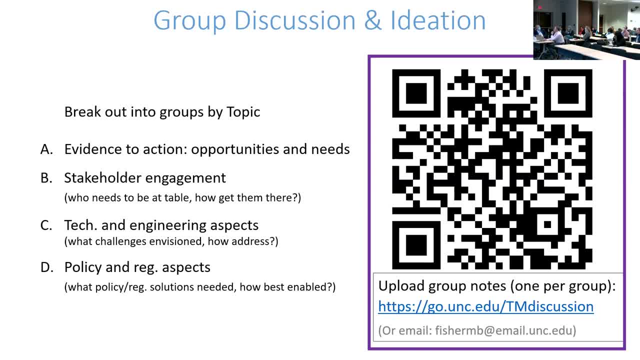 in the MIC setting. is there certain technology or solutions that are existing or could be thought of that you know might be applied? and by giving a little bit more power to the household, because you can't move or like, change your house or change all your fixtures or all the pipe, a lot is out of the hands of people who are being 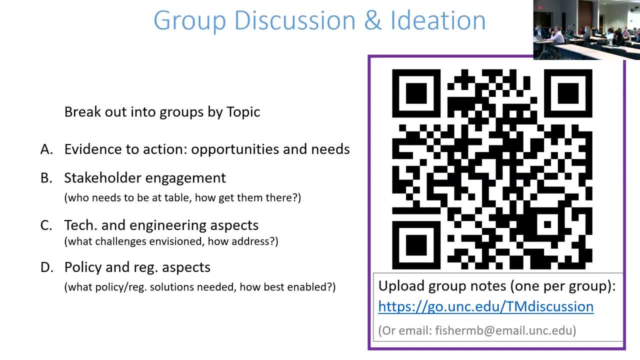 affected. so that's a great point. i think you know what is the educational campaign that needs to be taken on for this because, like you said, you can go and talk to a government, have them instituted, but a local home homeowner may not be able to do that, so what? so i think that's a great component is the 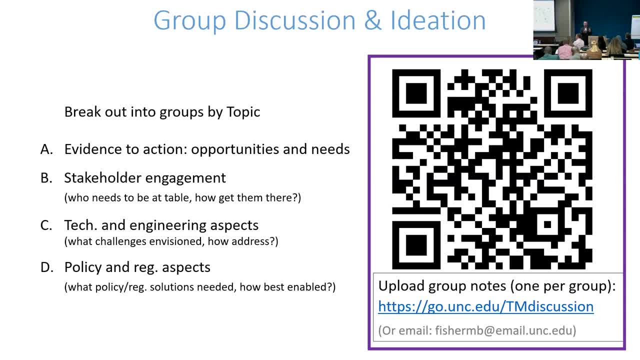 preventative, the remediation, but also the education, because there are solutions out there for individual homeowners and and usually pretty cost effectively too, to be able to address lead in drinking water in a home, whether it be point of use, point of entry, filtration. there's several different areas that you can't address this but, to your point, the average homeowner doesn't know that. 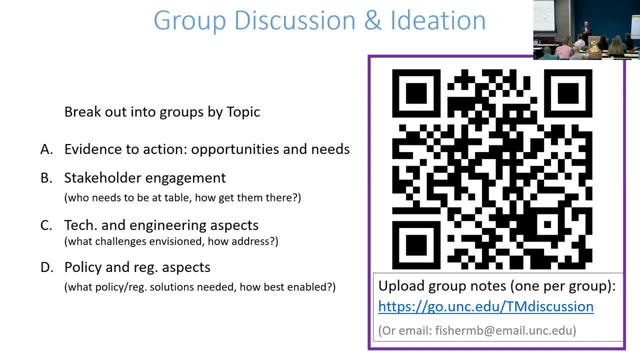 and they don't know what to look for. and christopher talked about certified products and it's all like: what does that even look like to a homeowner? how do they know what a certified product looks like? so i think that's a great point. that looks like a question back here. 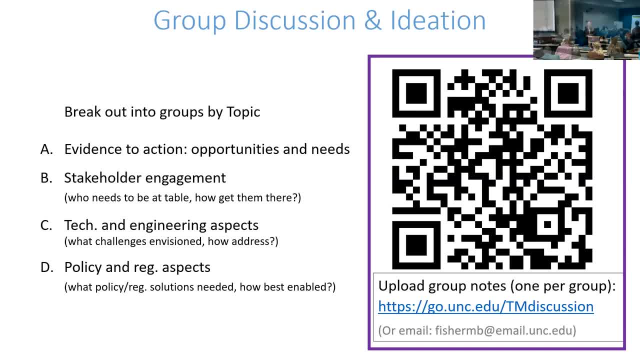 or comment. my name is jonah kudago. i think, from the policy level, we need to encourage the government to ensure certification of contractors, because there are very people who introduce many things into the ground without regulations or without adhering to any instructions. so that is one thing, and then the second thing is: um, i think we need to get our universities at the 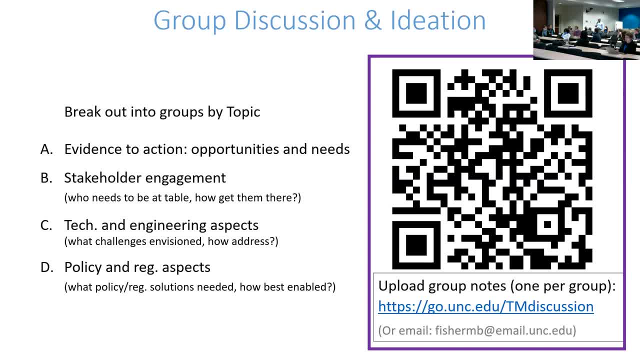 various countries involved. we need to empower them to know what they have to do on the ground to save the local condition. sometimes these are discussed at this level and 90 percent of the local universities don't even get to hear this or get to see this. so how do we discuss somebody's problem? 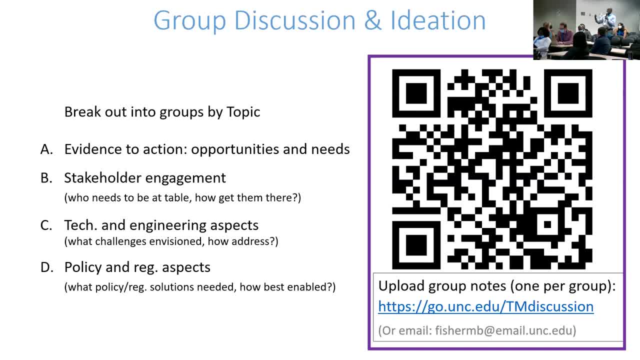 find solution for somebody who is not involved in solving the problem. so that is a big thank you. thank you, that's a great point. you'd have all the certified great products in the world, but if you don't have someone who's capable and competent of installing it, that's not going. 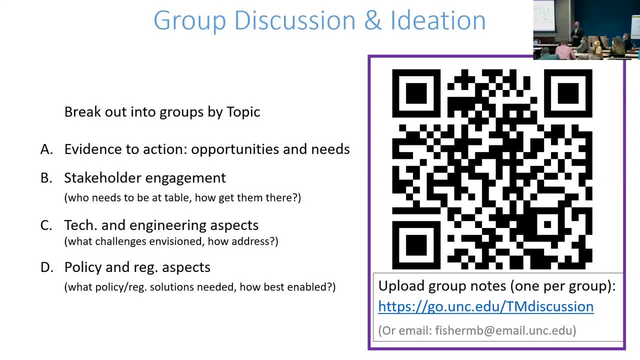 to defeat the purpose a lot of times. okay, yeah, i was. um, i guess my comment would be to also look at like a lot of these products are in unregulated markets in these well-known countries. so somebody's filling a gap and so just to see how we integrate that and get their perspective. 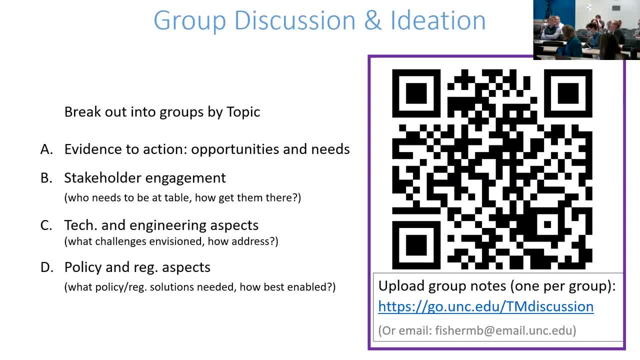 and how they fit into the larger scheme of things. um, because you can have a policy there but they're not no enforcement enforced, or and they're maybe not even getting that message in general. um, for that, and so that's again. we're in education. definitely, that's great. education is a big part of enforcement, because there are countries and 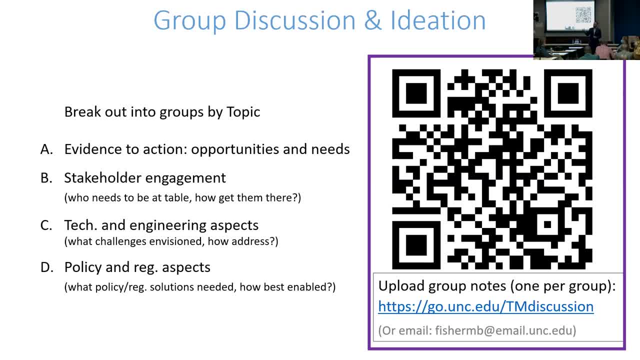 in regions that do have specification requirements, but it's very little enforced. So how do we address that? Probably have one or two more comments and it's at the top of the hour, so we're probably gonna have to adjourn after this. 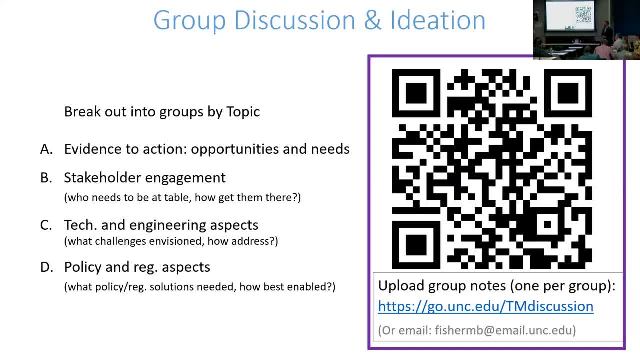 Hi, I'm Katya Cherkmele from UC Berkeley. I just wanted to make a quick nuanced point to follow up about the technology. So often we say you know there's tons of technologies out there, They're low cost, simple, easy to use. 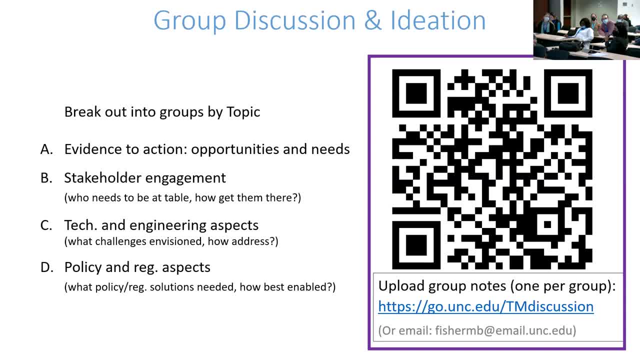 And we use these terminologies, but I think we have to think about who actually is doing the treatment and what is the gendered labor burden and the cost that's recurring as a result of doing this at the point of use at the household. Oftentimes it's women that are in charge. 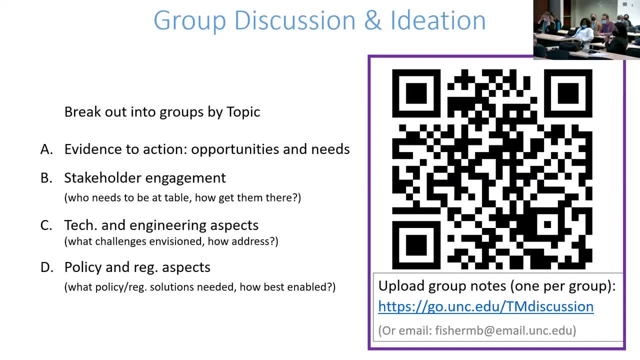 of provision of water and the treatment And a lot of these technologies. it's not like you pay the capital cost and they work forever. You have recurring consumable costs. You have to think about if it's an adsorbent based filter. 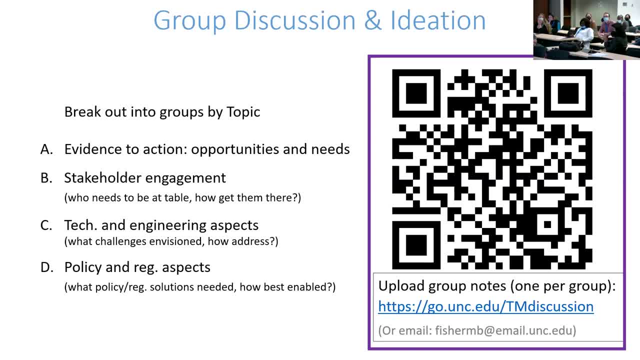 who's gonna actually come in and replace that? And if it's a membrane based thing, where are you gonna source the material? So there's also some complexities associated with actually operating and maintaining a system long-term, especially in resource constrained areas. There's one more comment in the back. 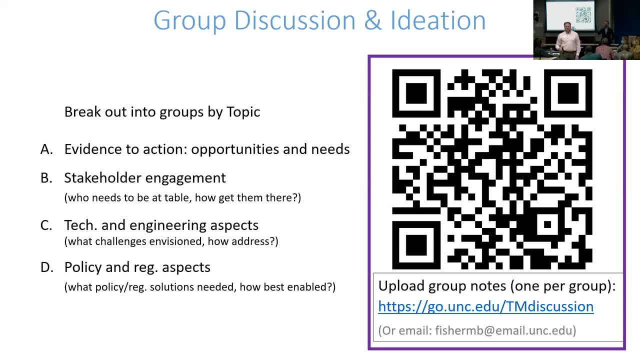 I agree with you a hundred percent. That's something that people and, especially when it comes to the operating maintenance. you may install a filtration device or some sort of mediation, but if you don't maintain it, it gets contaminated. You don't change the cartridges. 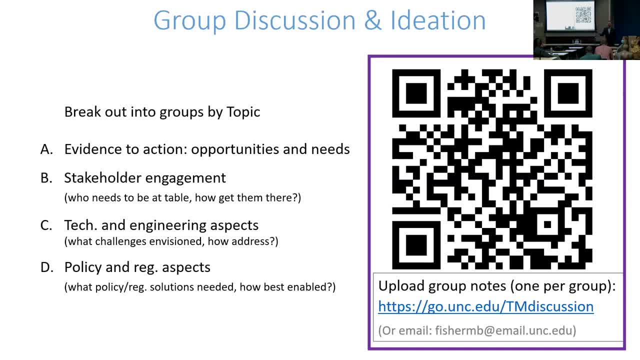 It actually gets. the water gets worse. It's long-term than it was originally, So it can even be worse than a bubble. Hi, my name is Christine Marie George. I'm a professor at Johns Hopkins And I've been working on epidemiology of arsenic. 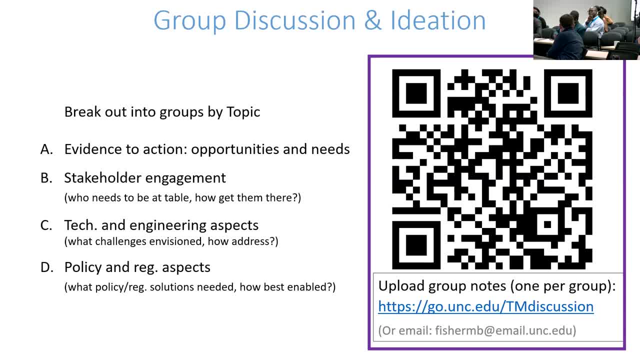 for the past 14 years And I'm actually giving a presentation at 3.30 on some of our household point of use arsenic filters that we introduced in partnership with American Indian communities in the Great Plains. But what I wanted to mention is that there's a lot. 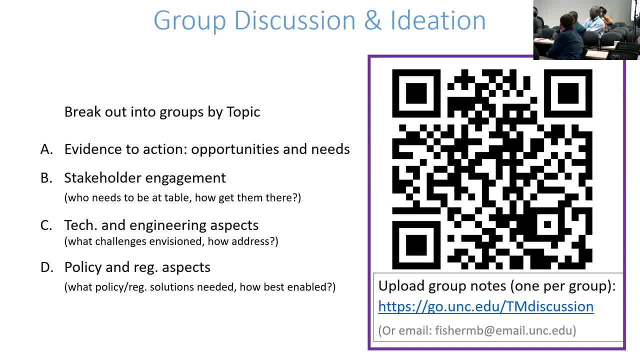 of community-based approaches that people aren't implementing. So, for example, I had lived in Bangladesh from 2009 to 2011, and had worked on a UNICEF project where we worked on sea-based arsenic testing, and it worked really well. 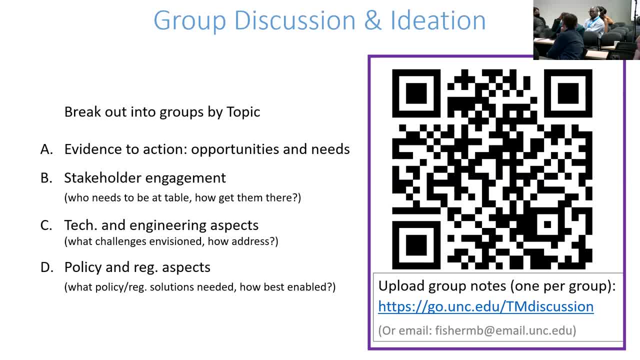 where people in the community were buying an arsenic test for their well, But after this we published a randomized control trial and nothing happened. So I kind of wonder what we can be doing based on the knowledge we've already gained from our research group.